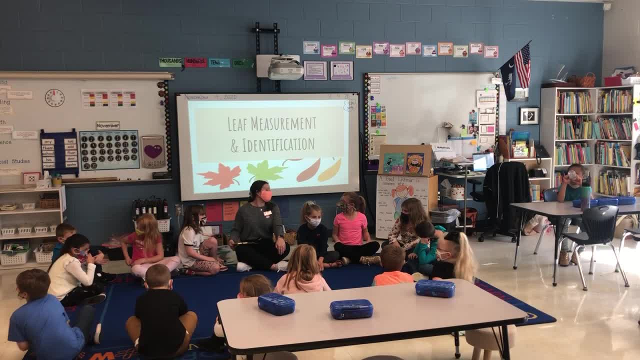 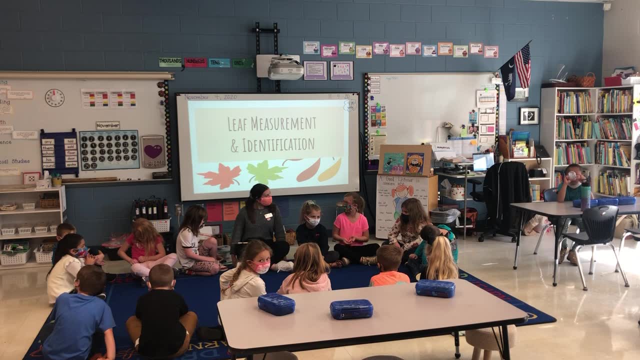 Um, like, they're all different. They're all different. How are they different? By their color and by their sizes and shapes. Oh, and their shapes: By color, sizes and shapes. So does anyone ever wonder how else we can identify leaves? 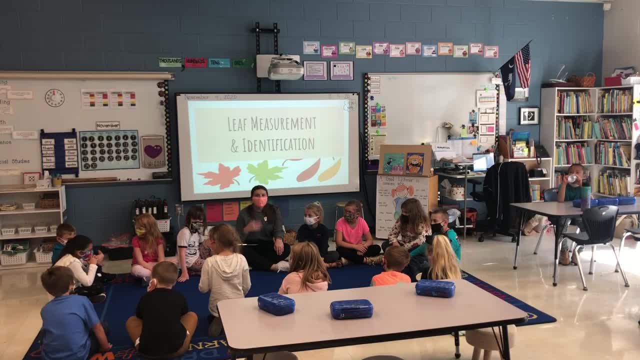 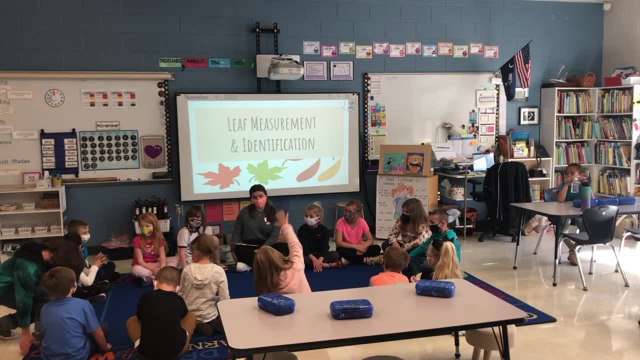 Jackson, do you ever wonder? Yeah, how do you think we can also identify leaves? by By measurement. By measurement, Oh yeah, I think that would be a great way to identify the type of or what characteristics the leaf have. 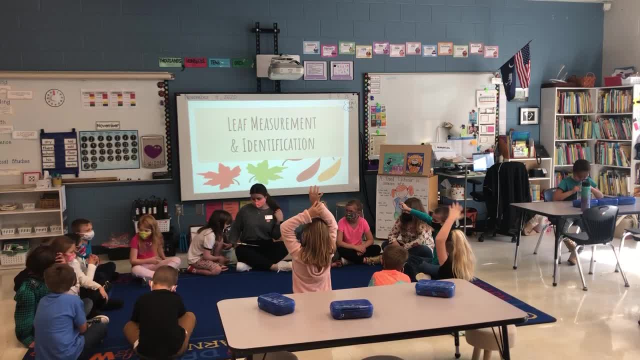 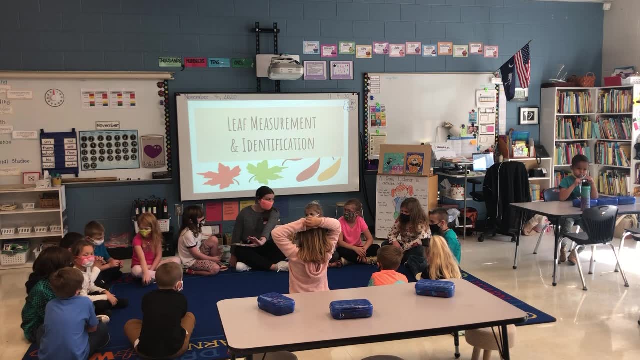 Um, so today we're going to measure these leaves and we're going to use two objects to measure these leaves. Okay, So, Jackson, you were right, We're going to use his prediction and we're going to measure the leaves today. 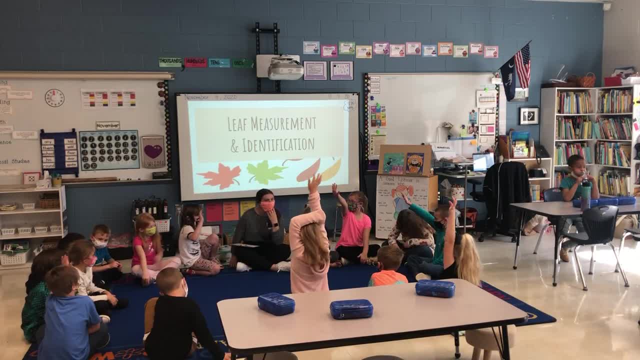 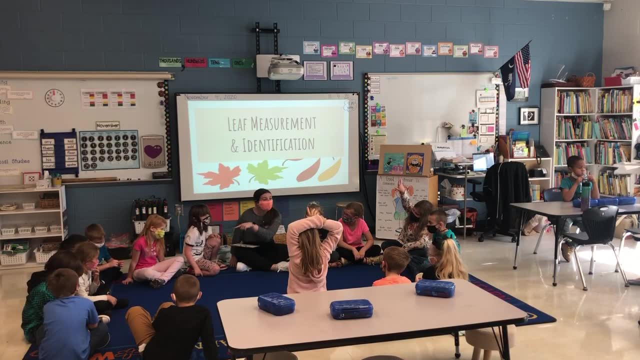 So how do you think we can measure them? What can we use, Isabella? what can we use to measure them? We can use a pencil. We can use a pencil to measure. A stapler, A stapler to measure. 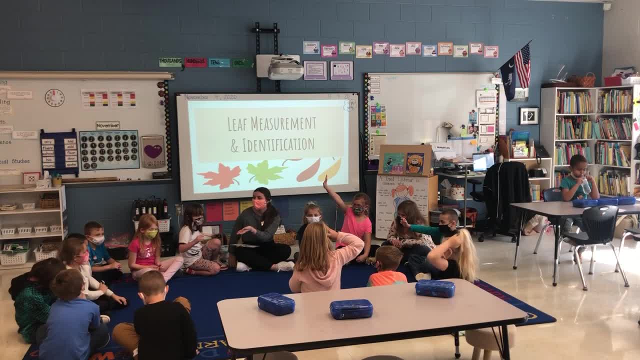 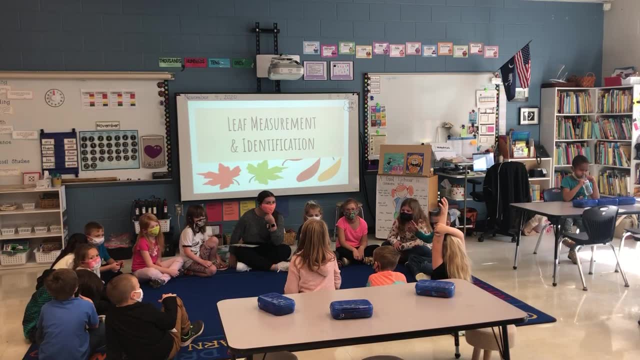 How many feet it is. Chelsea, A ruler, We could use a ruler. Wakely, what did you say? We could see how many feet or inches. How many feet or inches, Okay, so yeah, those are all ways that we can measure a leaf. 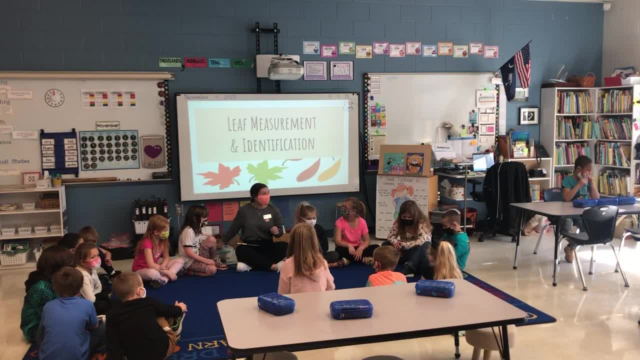 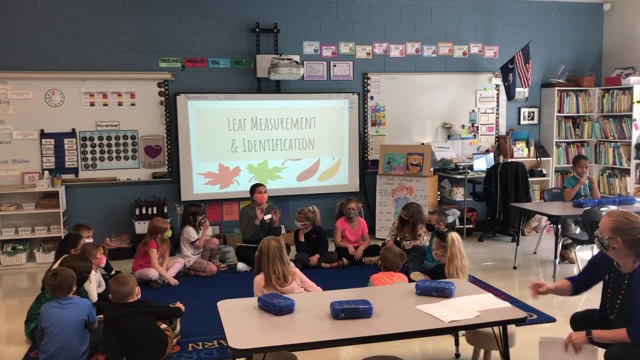 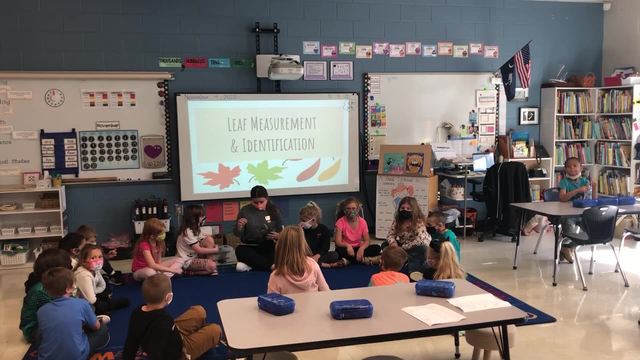 Um, today we're going to pull out a model. Yep, Noah said that we can use our feet, We can use a pen, We can use a mask. Can I have one bag of each? Certainly. Thank you, Yep. Okay, so I brought in some leaves as well. 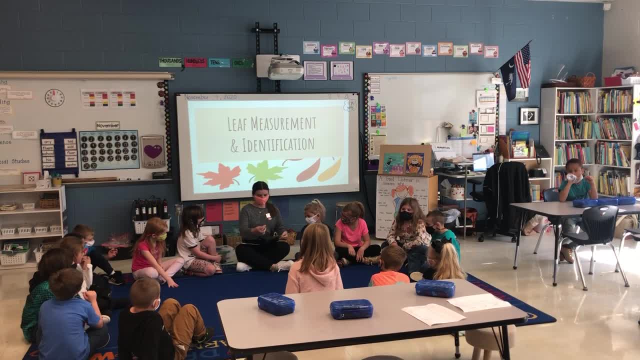 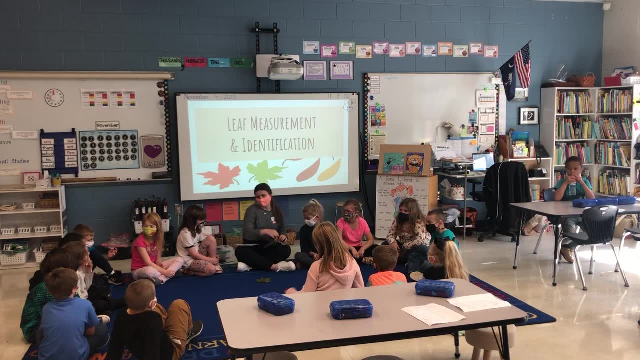 And so I'm going to use this one first, And then Ms Byer is going to pull over our forms of measurement. Thank you, She's going to pull over my forms of measurement, except for I have to bring them to me because I forgot I needed them. 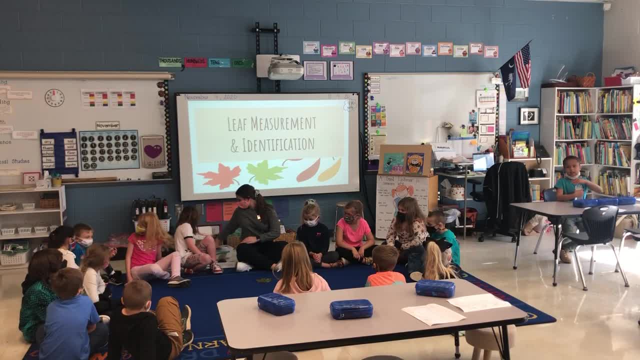 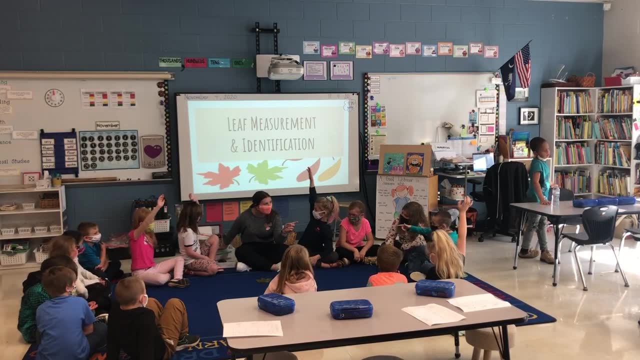 So we're going to use two things. Who has a guess of what one thing we're going to use? Noah, Um, colorful, Colorful, Colorful boxes. Carly Sue, Candy, corn, Candy, corn. You guys are both right. 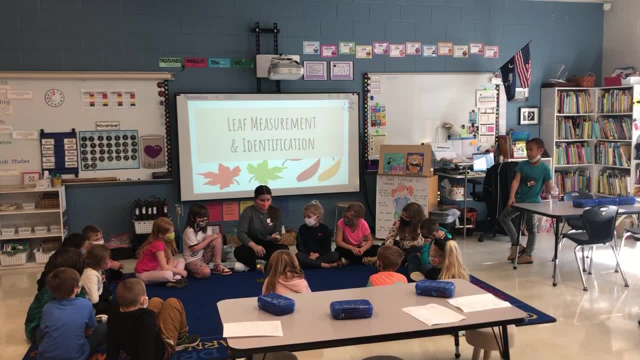 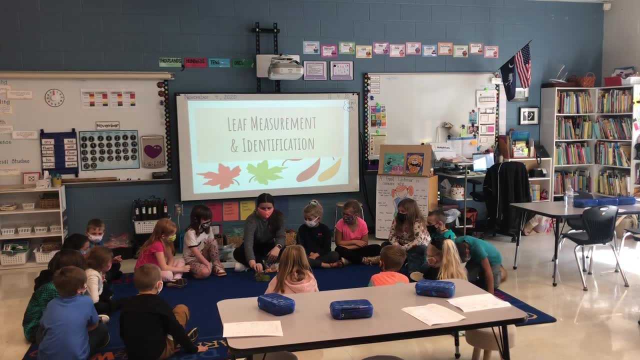 We're going to use these square tiles. Can we eat some of these? Um, maybe I did bring some more just in case. And then we're going to use candy corn. Okay, So what should I first do with this leaf? 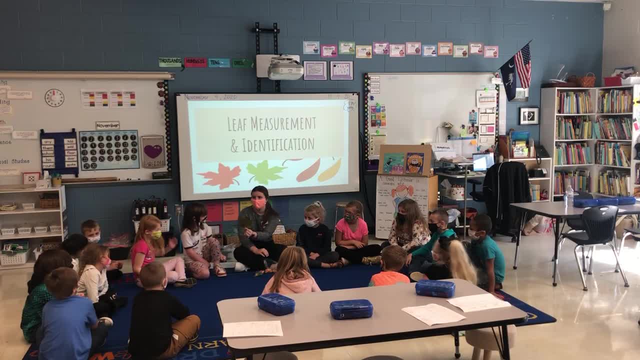 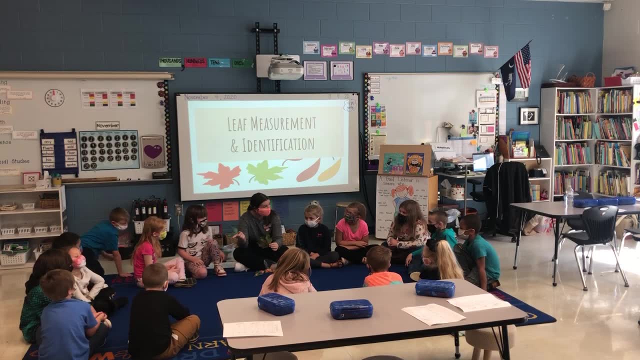 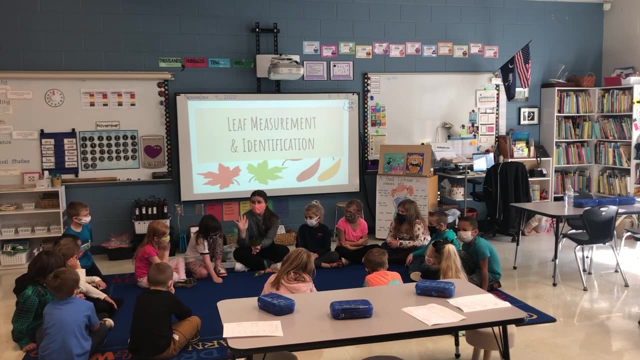 Jackson Measure it. So did you hear Jackson? Yeah, He used prior knowledge that we used with our other lesson to measure it with our hand. So I'm going to use my hand and I'm going to put it up, Thank you. 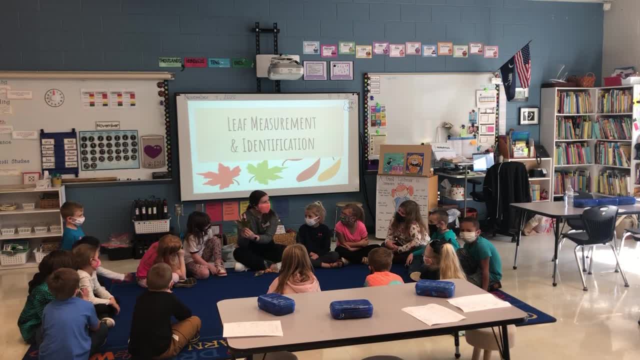 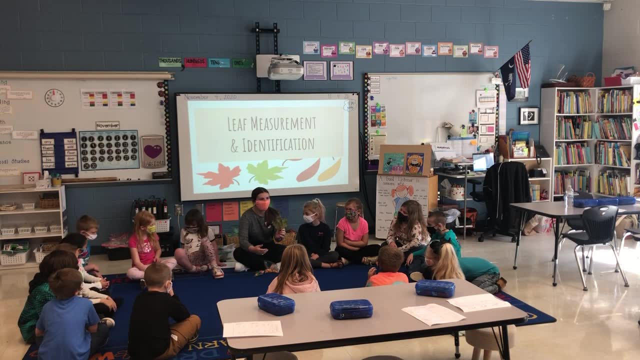 Do you think it's bigger, smaller or about the same size? Same size, About the same size. So this would be a Medium, A medium leaf. Okay. So should I hold it up to measure it or should I put it down? 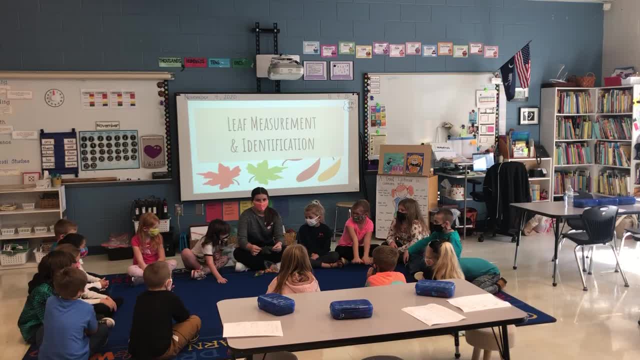 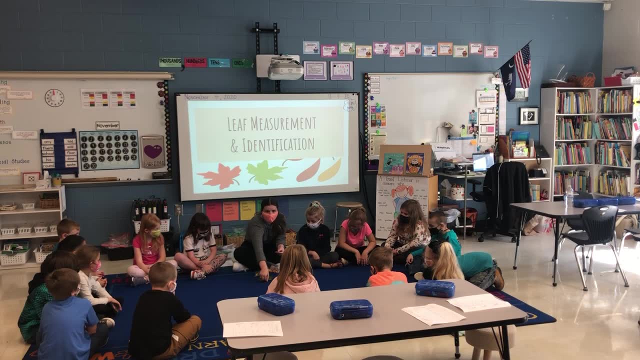 Should I put it over here? What do you think I should do? Put it down. Put it down Which way? Like this, No, Like that, Like flat? Yeah, Does it matter which side? No, Front or back. 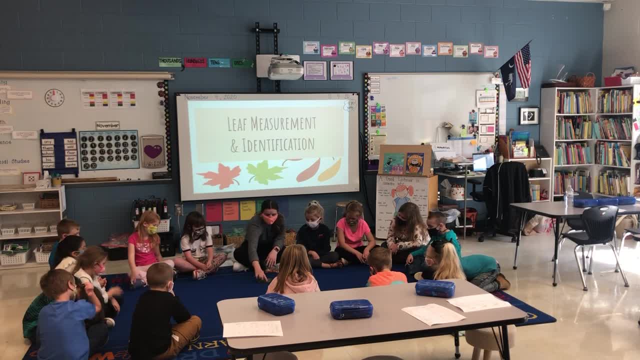 No, No, Because it's going to be the same. So some leaves might not have the stem, the stem on the leaf. So we're just going to measure the base. So I'm going to, we're going to find out the measurement of this. 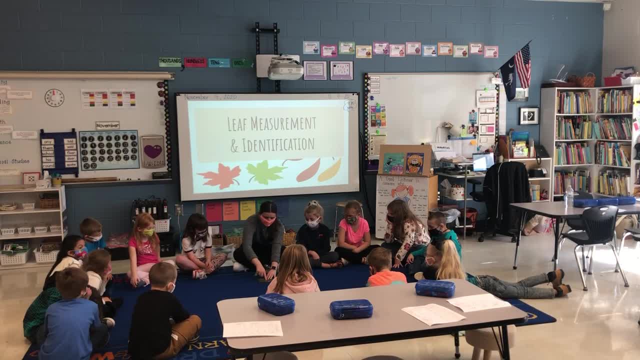 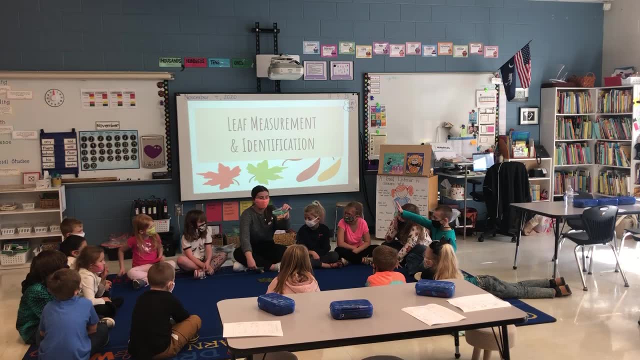 It's going to be the length, Okay, Okay, So let's cast a vote, because we're talking about voting this week. Who votes that we should use candy corn or square tiles? Okay, vote for candy corn. Okay, square tiles. 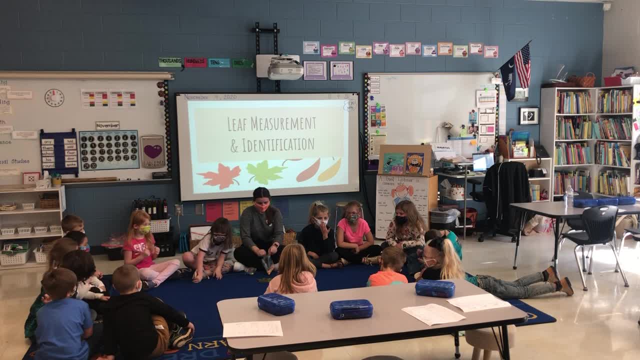 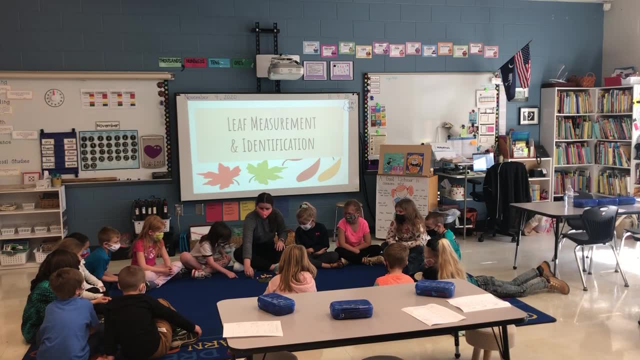 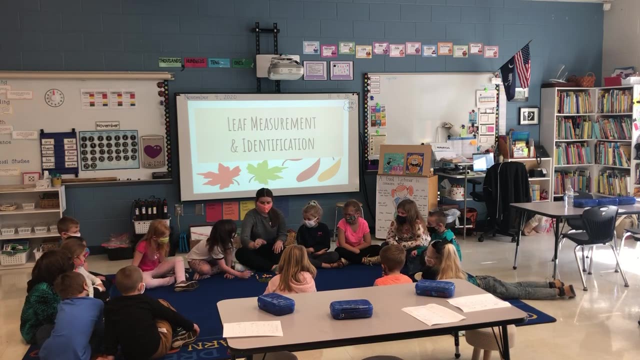 Alright, candy corn won. So how should I place the objects? Should I place them like, Yeah, all the same way? Like, should I put them space in between, or different ways? Where should I put the first one? Do you think it would be more beneficial to measure it all the way over here? 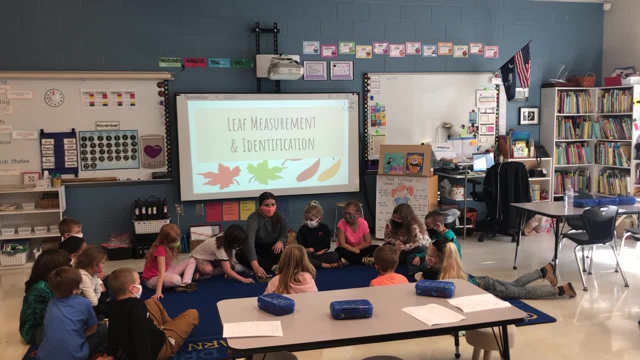 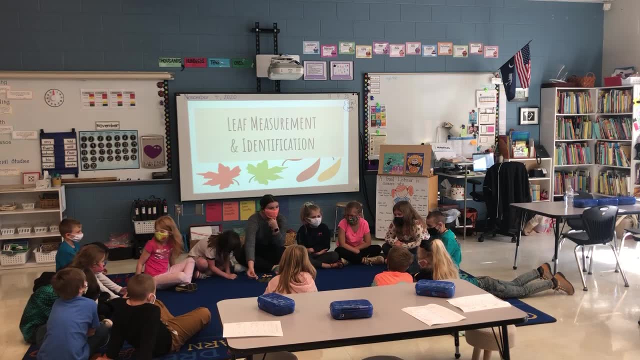 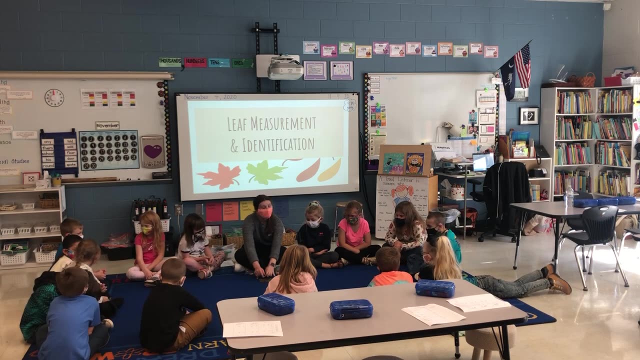 Yes, Or right here, Right there, Where at In the middle. Okay, so I'm going to place it Candy corn, Okay, if I don't put it on the middle. Amira said that I could overestimate how many candy corn it takes to measure this leaf. 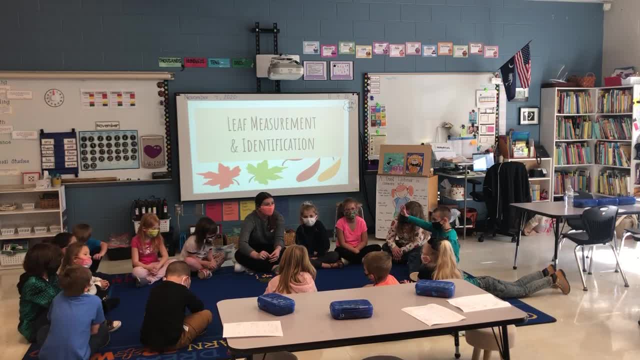 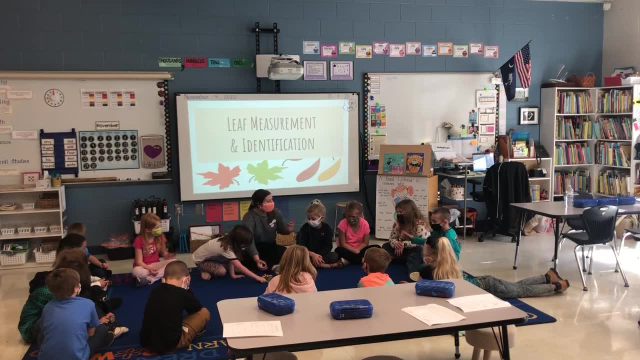 Yeah, and now you put the answer on Uh-huh. Okay, so where should I place it at? So we know we're going to place it in the middle The base. Ansley said we should put it at the base, because should we put it right there? No, No. Ansley said we should put it at the base. 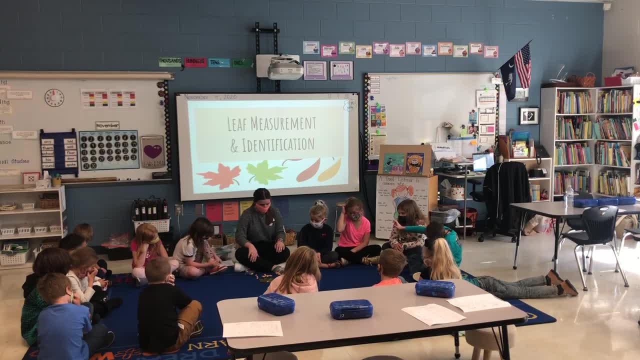 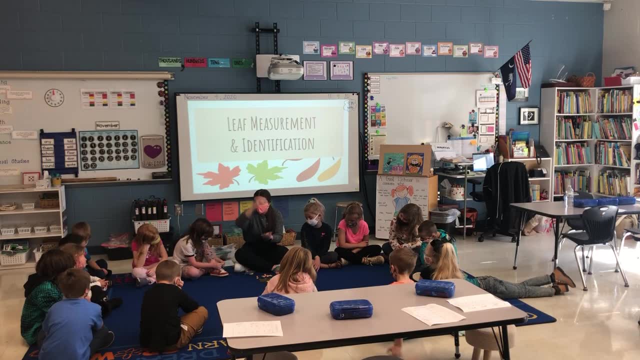 Why do you say that we should put it at the base? Because that's where the leaf starts. That's where the leaf starts to grow. So is it one candy corn? No, No. So what should we do? Add more, Add more, Okay. 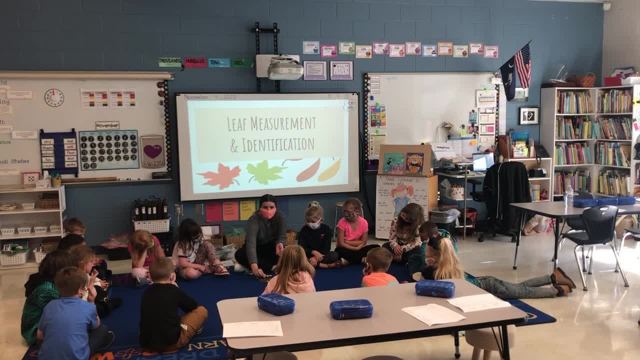 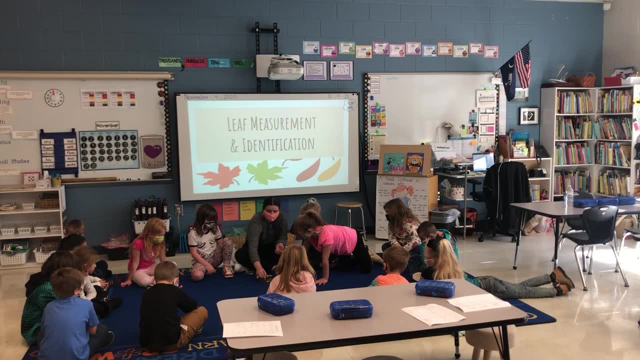 So where should I put it? Right here, Right here, No, No, Right on top of it. On top of it. Should I put it this way, or like this way, or this way? Yeah, The same way. The exact same way Ansley said. we should put it the same way. Why should we put it the same way? 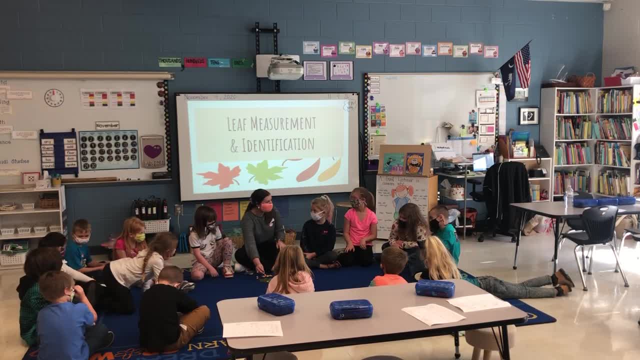 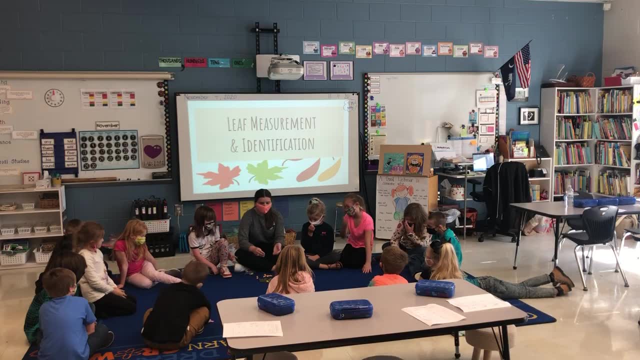 Because it might be the same, So it will be the same And like, if you do that, It could be smaller or bigger than the size it should be, Okay. So Ansley said that we should put it the same way so that our estimation of the length of the candy corn is like pretty accurate. 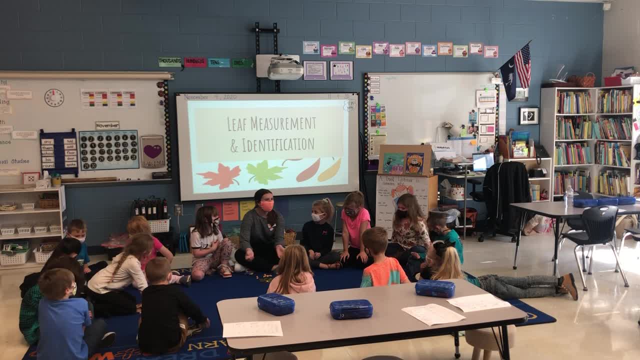 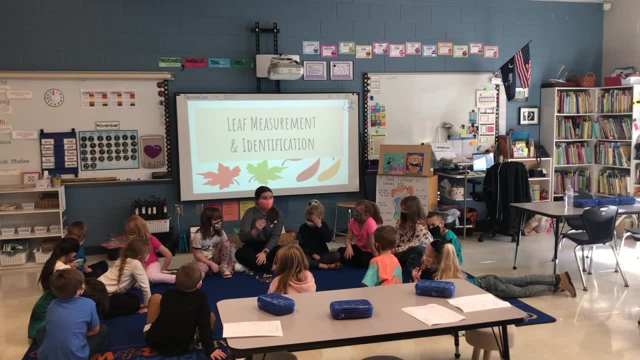 Instead of um, instead of like putting it different ways, it could mess up how many candy corn we use, right, Because we're going to say that, And then we could use all of them and you don't have a candy corn. 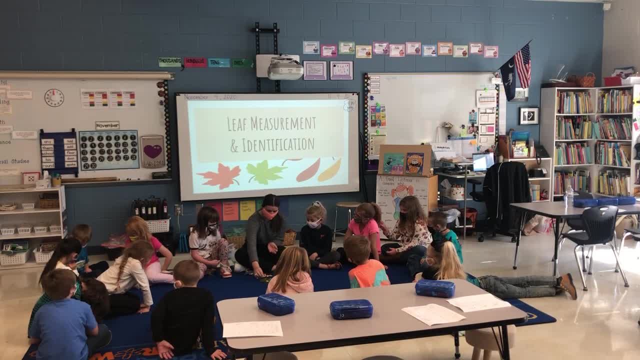 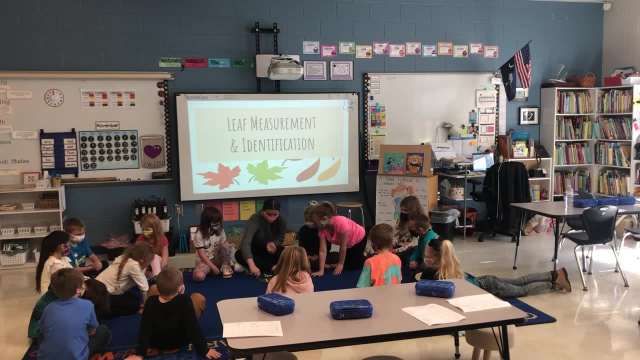 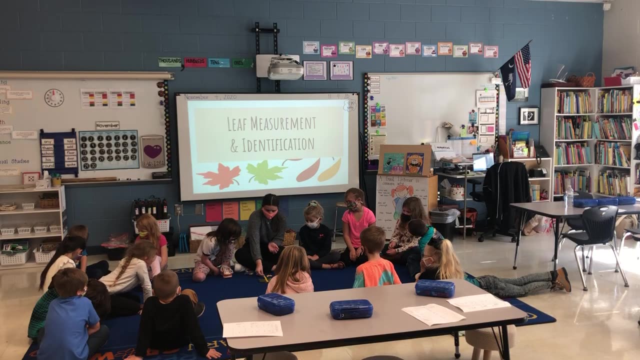 Mm-hmm, Okay. So should I just repeat that, Yes, Yes, Okay, And keep on hitting it until it comes all the way up to there. Should I add more candy corn? No, No, But I have all these candy corn. 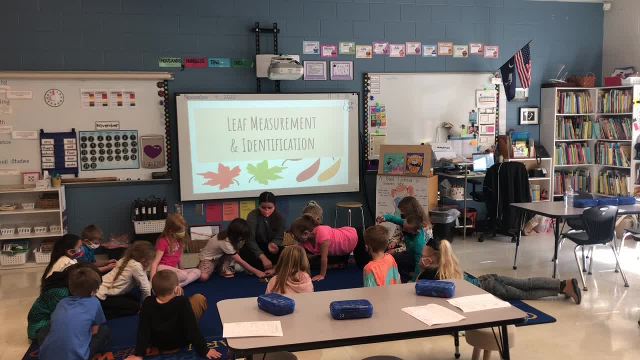 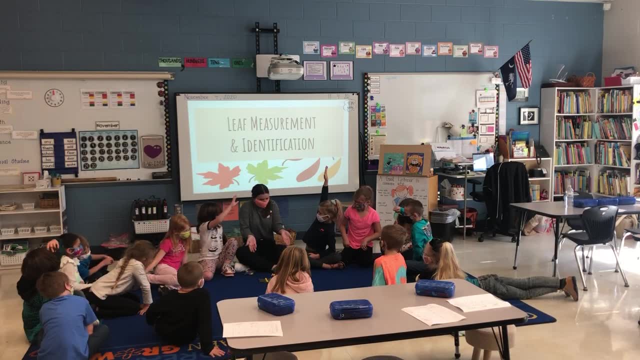 Wait, You have half candy. Take it away. Okay, So I don't need all the candy corn, because we'll only. Why should I not use all my candy corn? I have all this candy corn. You can use all of mine. 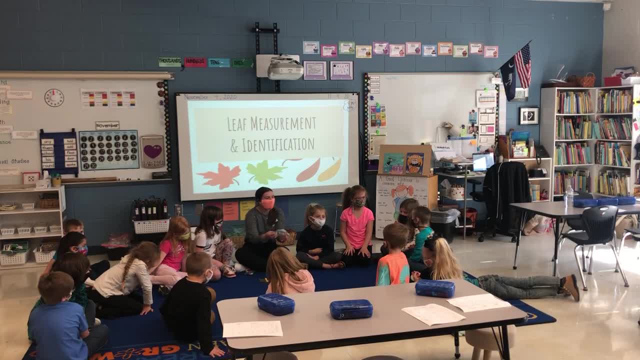 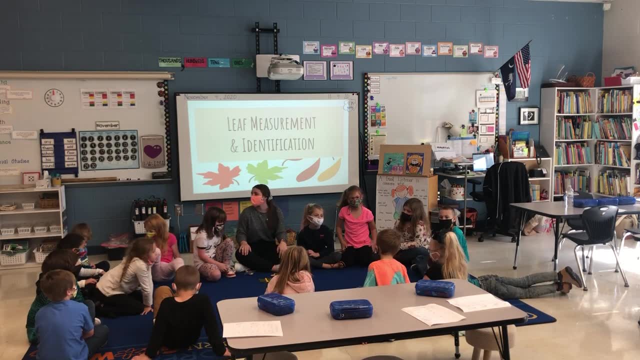 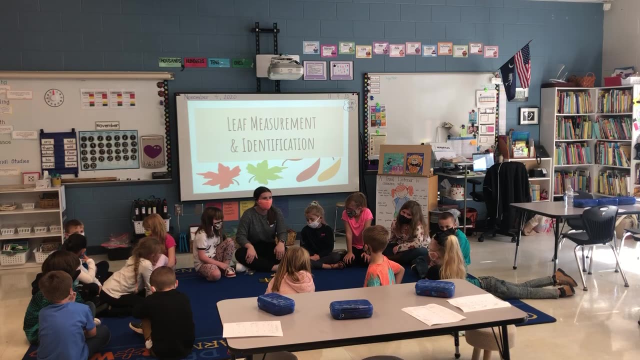 I mean, why do you think that I should only use, Like, why should I not use all of my candy corn to measure, Because it's only half feet long? Because, um you could, um you could, you can count them. but then you write the answer down, but then you'll have too many. 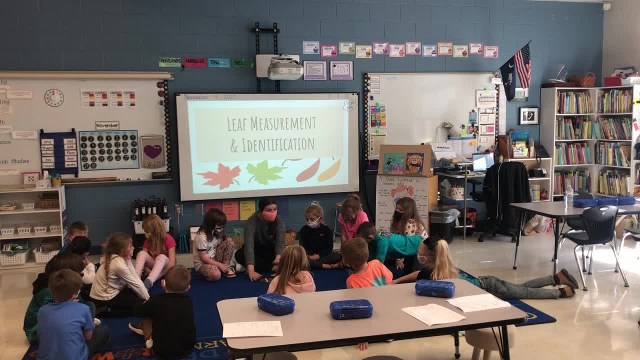 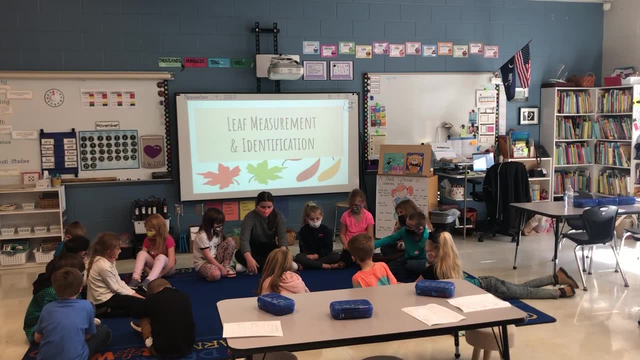 Oh, so I have to only use it to cover the least, or else, If I use all of it and I would have too many. Yeah, Okay, So all right, So I shouldn't keep going. No, Should I add more at the bottom? 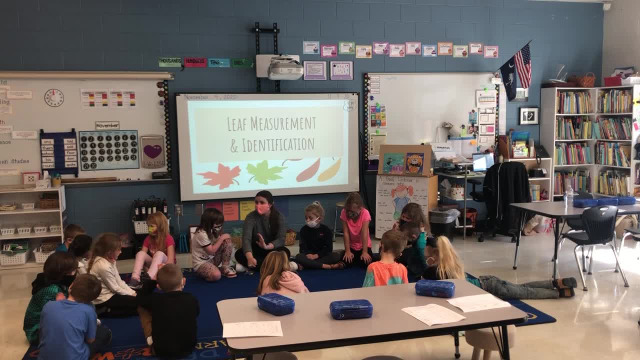 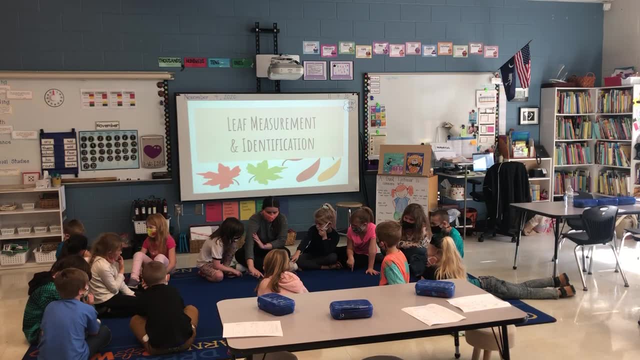 No, No, Okay. So let's count together, okay. Can we see how many candy corn? Yeah, Yes, One, two, three, four, five, six. So what would we say to describe this leaf? There are 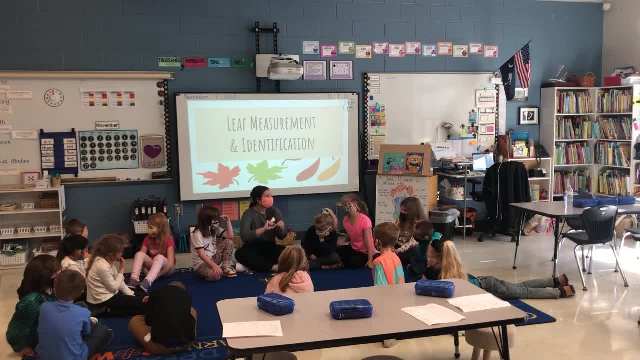 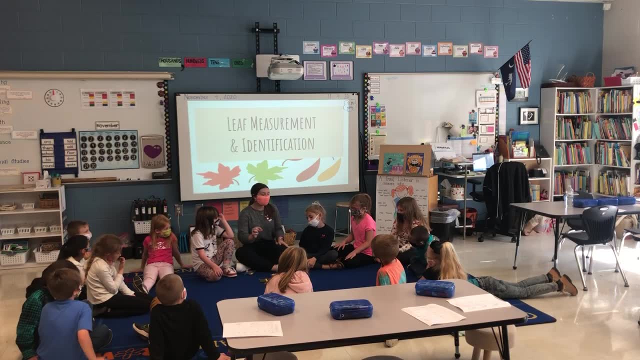 Six inches long. Is this an inch? No, Okay. So Ellie Ann just said that it's six inches long, Six long corns, But then Ansley just corrected her by saying it's six candy corn long. So why so? how do we not? 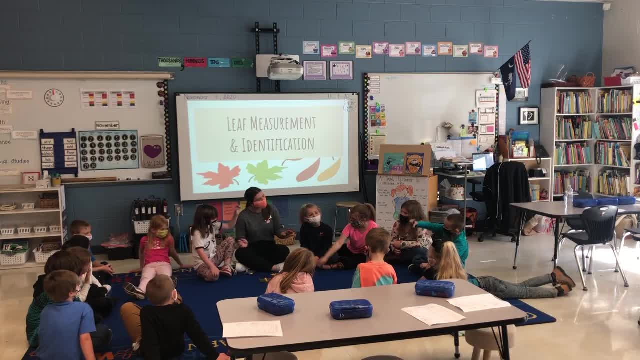 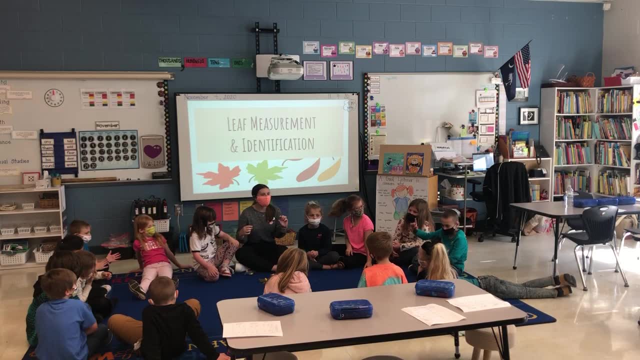 Um, why are we not saying inches? Because it's candy corn, Because it's candy corn, Because it's not short, Mm-hmm. Um, what would we use that would say inches, Amir? what would we use? A ruler? 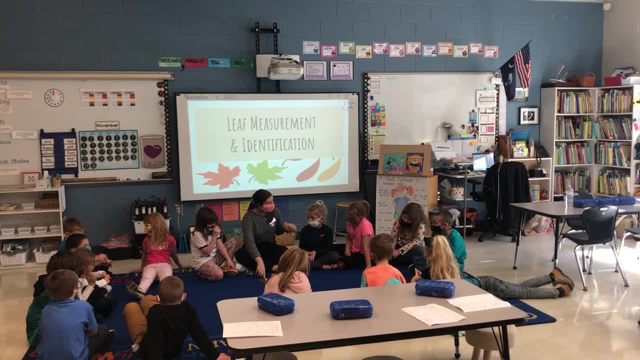 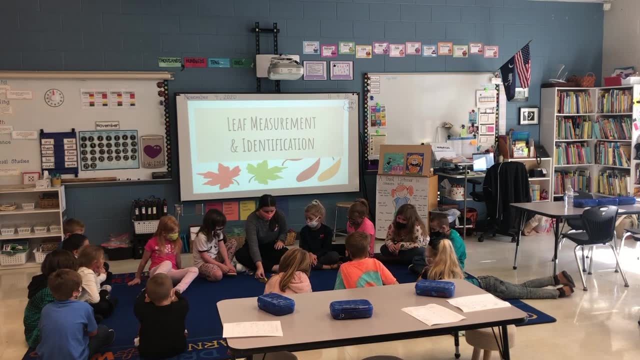 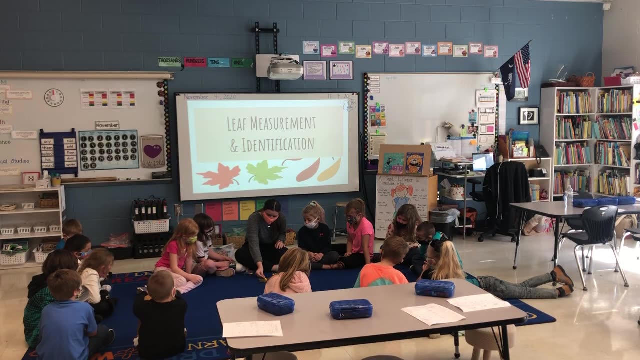 We would use a ruler. So for this measurement, like Ansley said, it is six candy corn long. Okay, There's so many pieces here that you couldn't fill in with another piece, Okay, So, um, Ansley just pointed out that there's a little tiny piece that wouldn't fit a whole candy corn. 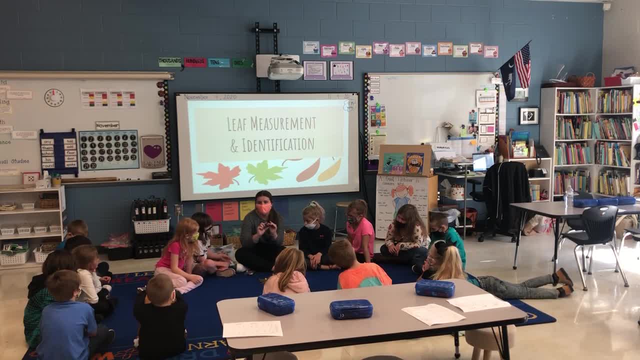 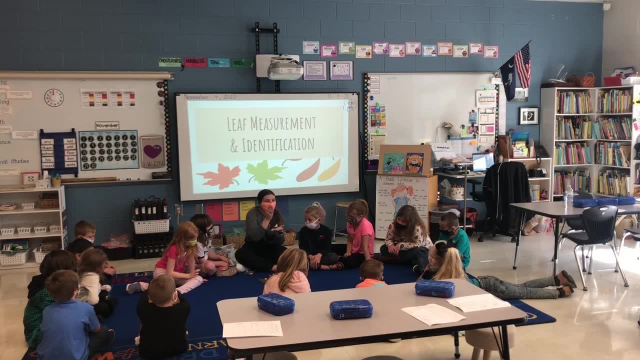 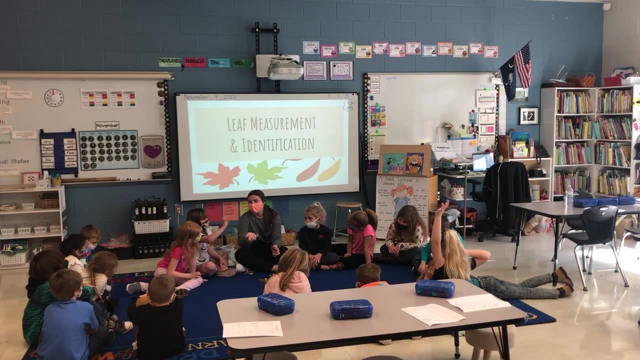 So I think, um, since the candy corn is only one size and there's not little pieces of candy corn, we're just going to say that it's six, rather than. a ruler has those little um other marks. So it's like if it's three inches but there's a little bit more, it'd be like three and an eighth of an inch, because it has those tally marks. 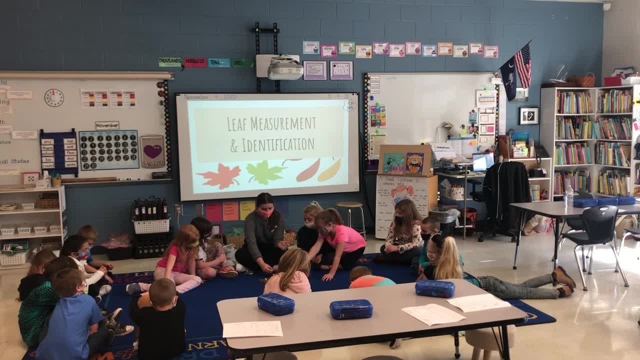 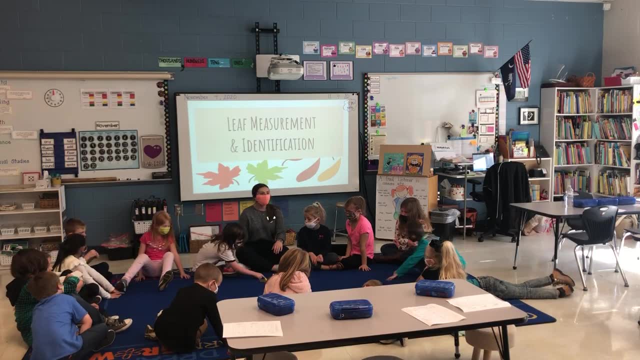 Or you can break it up in half and put it there for a little. I have a connection to the marker. I know it's solution. Um, you can say it's about six inches long. Oh Okay, Did anyone hear what Carly Sue said? 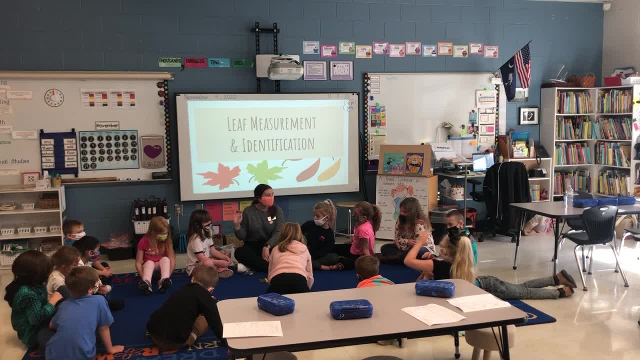 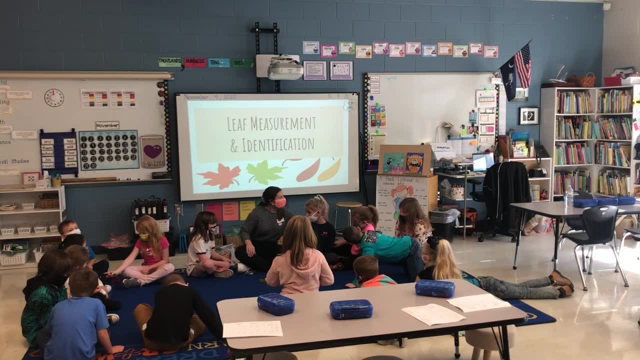 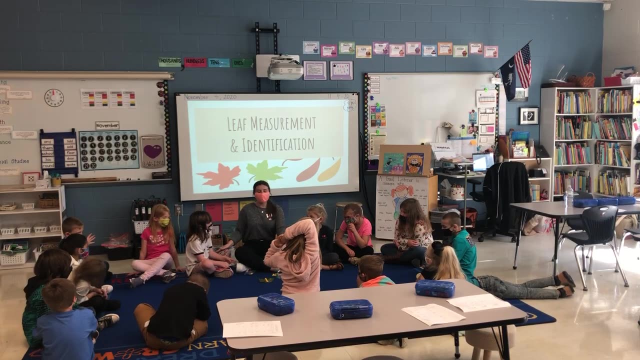 Yes, I did, I did. What did she say? It's a. it's about, um, it's about six candy corn, Um, so, um, thank you, Um. Carly Sue said that we could say it's about six candy corn long. 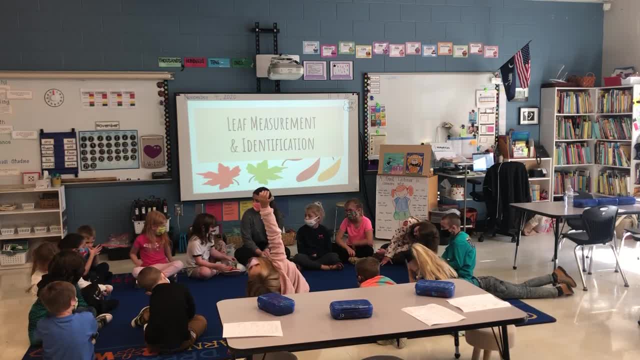 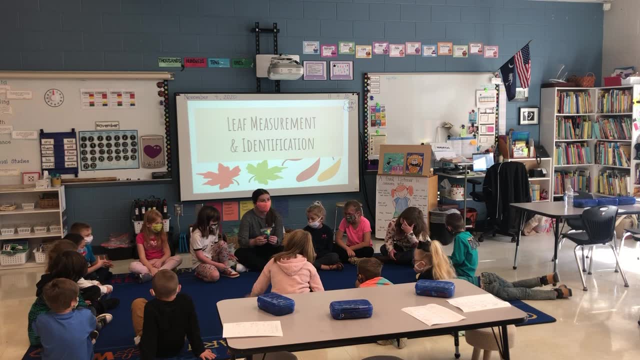 And so what does that word about mean for us? It's almost there, but it wouldn't be enough for a whole candy corn, Mm-hmm. So it's closer to six, Yeah, Yeah, Okay. So do you want to measure with the square towels now? 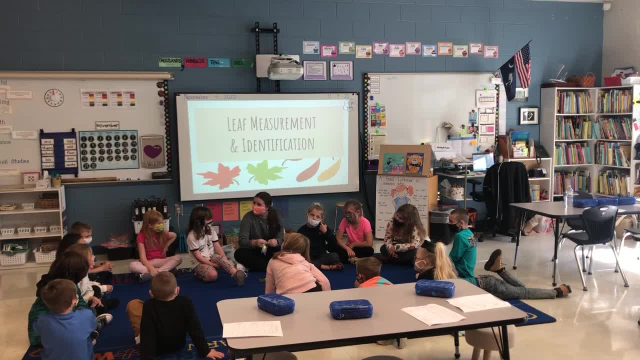 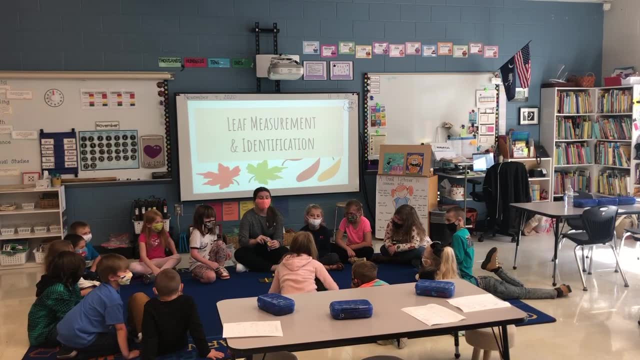 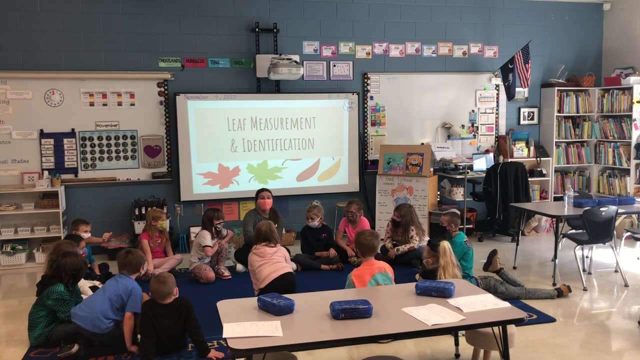 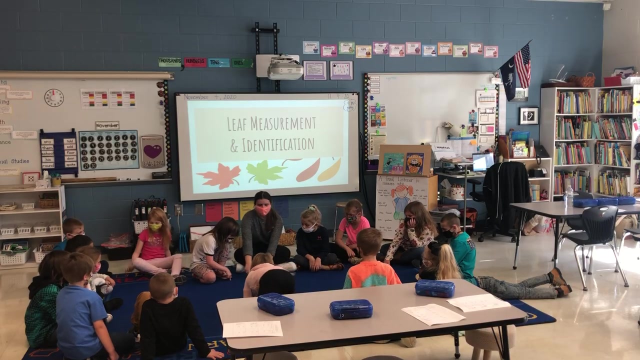 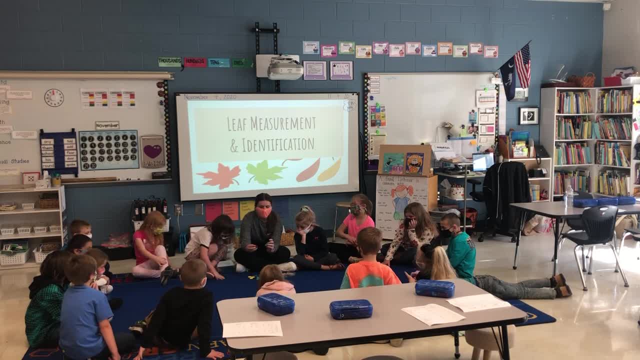 No, No, No. So should I use? oh wait, I have a ton of different colors. does it matter the color of these squares? No, No, Because what does it matter? Like what matters about this? They're the same size. 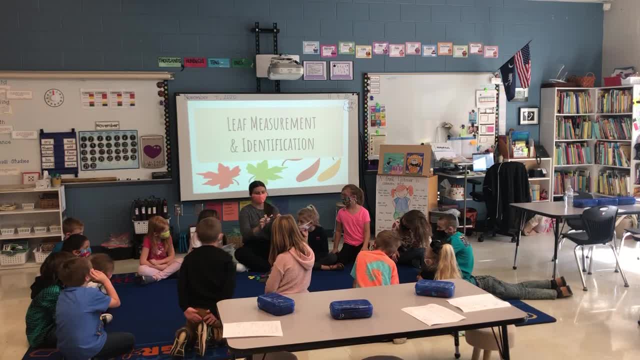 Ellie says that what matters about using these square tiles is the same size. Well, I already measured them and see. look, if you're concerned, if they're not the same size, you can just put them on top of each other and see that they're the same size. 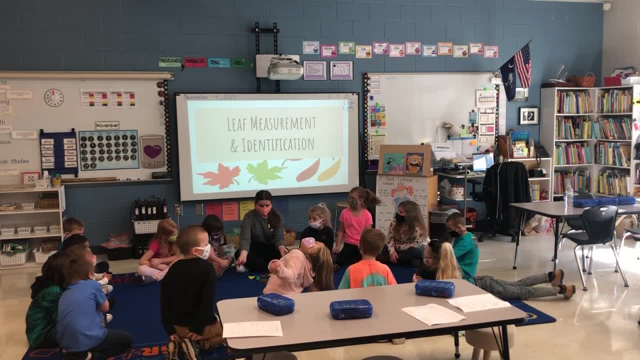 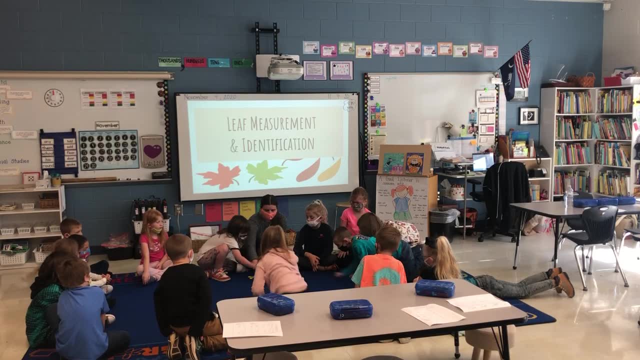 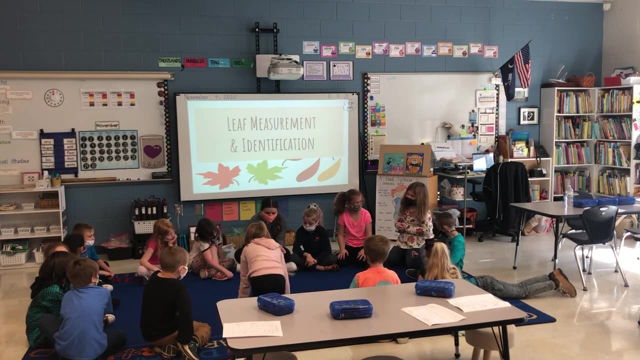 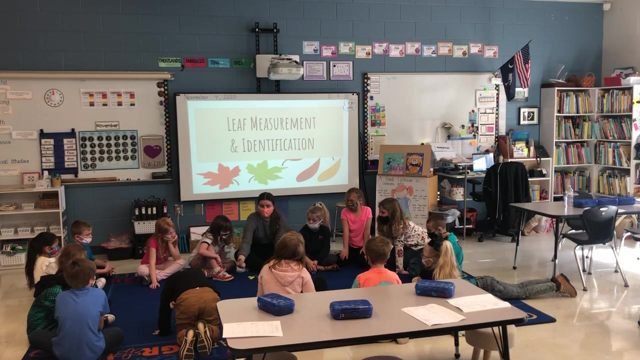 Yes, So can we say things are the same size? Yes, No, So should I start over here? No, You should start at the base. At the base, Yep, Thank you. Okay. is it two square tiles long? No, Should we add more? Yeah, Or should we take away? Add more, Add more. 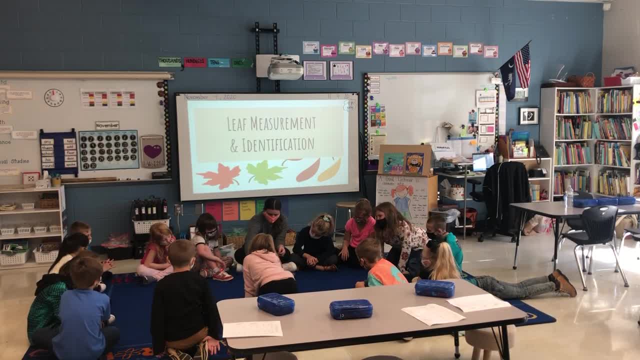 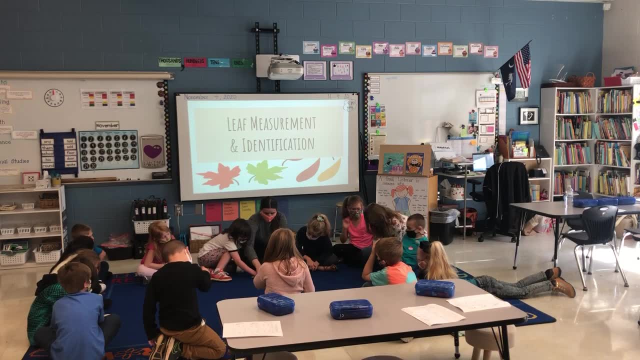 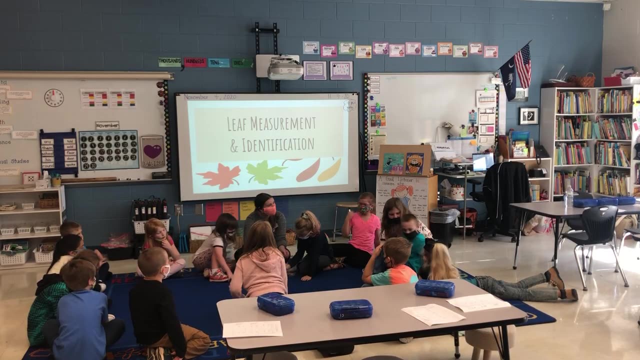 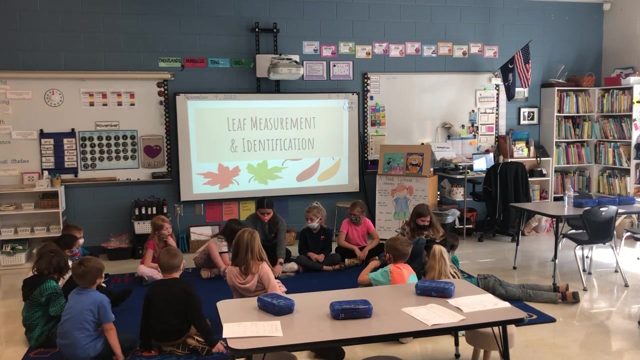 I think it's going to be four. Is it four, Or is there a lot longer? About two, three, four, Four, Okay, Oh, we can fit another one on there. We can go up to that. Can we check our spots too, Okay? so, oh wait, what happens if it's all like this? 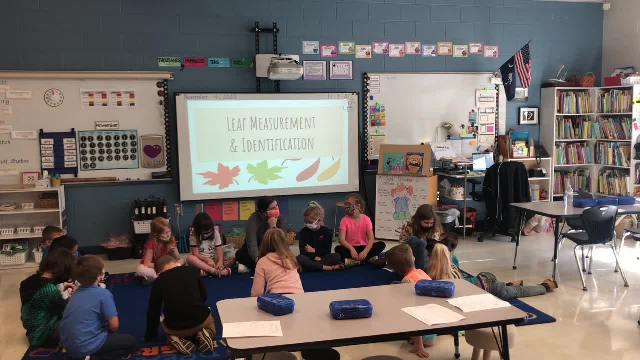 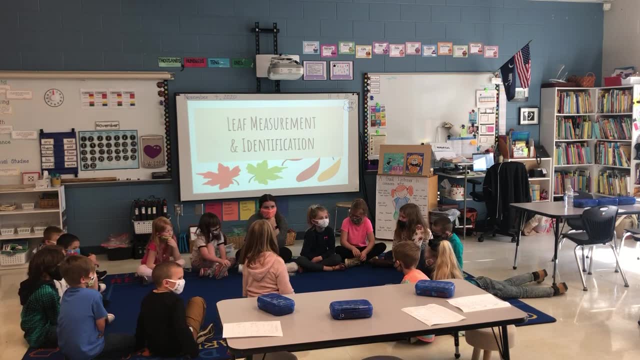 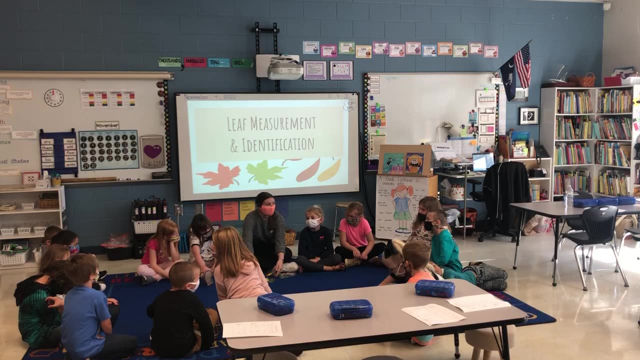 What should we do? So is the measurement correct if it's going to be all like this? No, Jackson, what do you suggest we do? Jackson says that we should make it straighter. Okay, so it can be kind of difficult to place these on the leaves, because they can fold up and stuff. 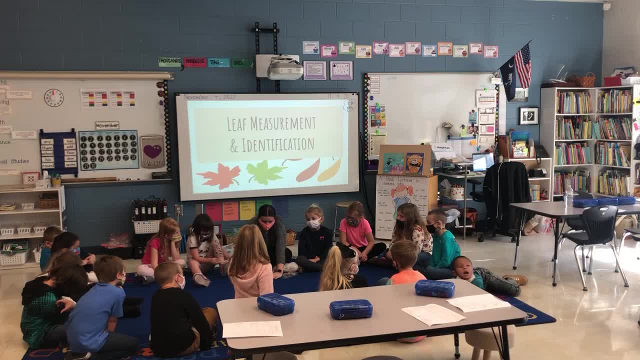 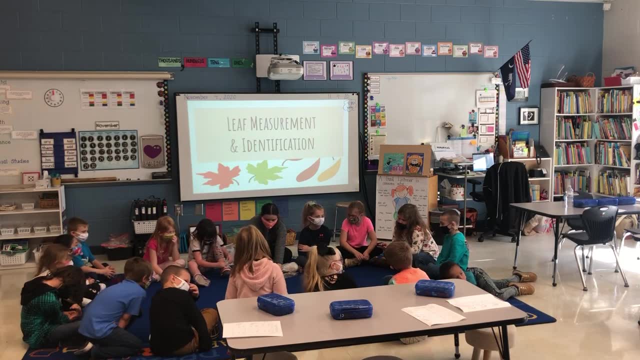 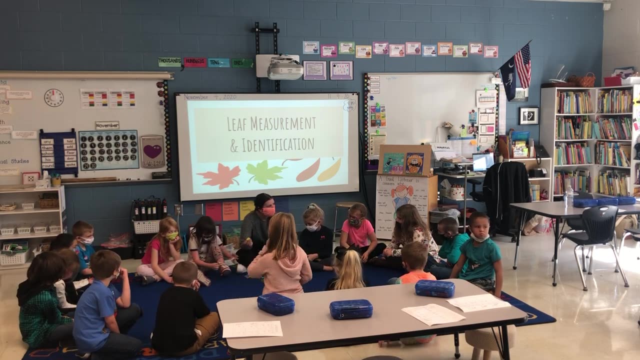 but we're just going to have to try to flatten it and then flatten. Okay, it fits. How many are these? Five, One, two, three, four, five, Okay, so what can we tell? if so, was there more candy cane or more square tiles? 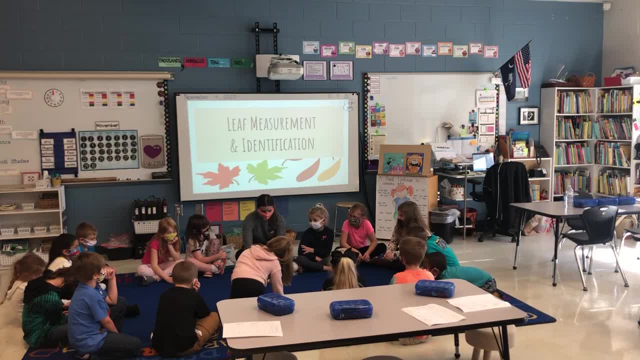 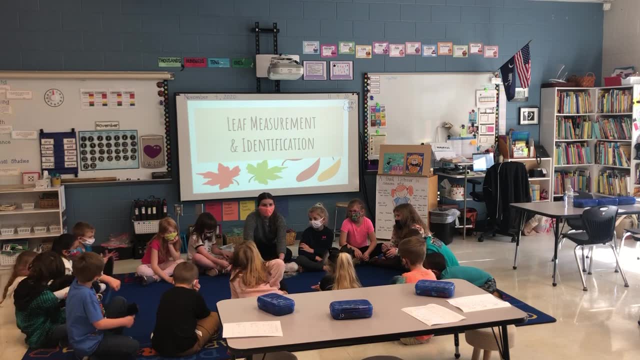 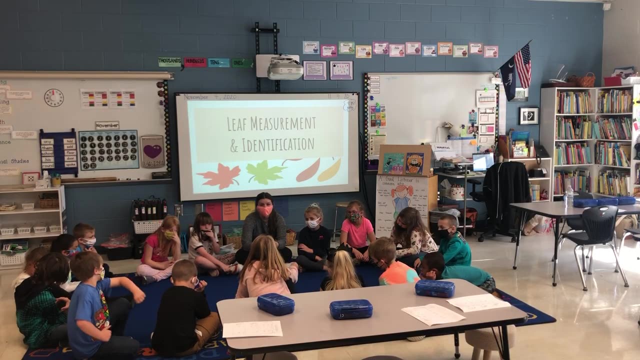 Candy corn. Oh sorry, Candy corn, not candy cane. So what does this tell us about measurement? More candy corn, but more candy corn than the leaf, because it's all the size of the candy corn. Yes, So The candy corn is smaller because it's a candy. 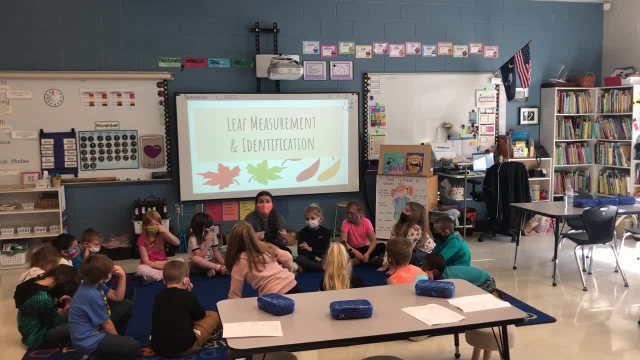 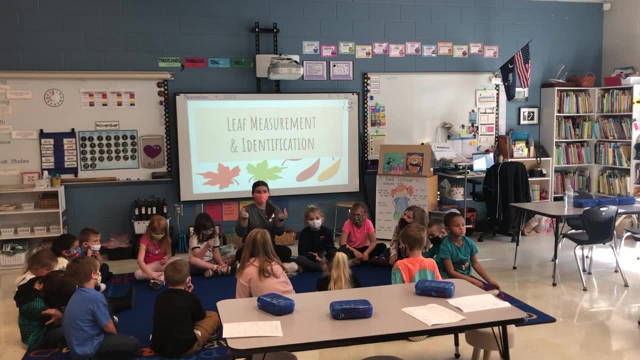 So when we're measuring, we can't just assume like everything's the same length, Like this is not the same length as this, right? No, no, it's not the same, But it was actually five and the candy corn was six. 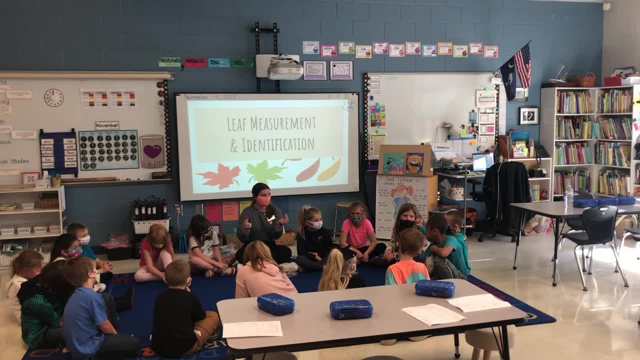 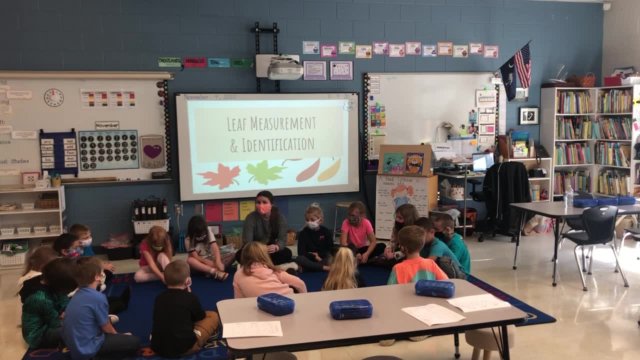 For example, you must be six year old, but you must be five and you're not tall enough. Okay, That's a good example. So does everyone understand, like, how we were measuring that? Yes, Okay, so that's what I want you guys to do. 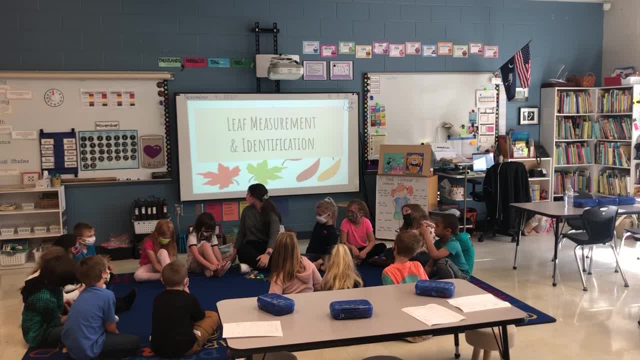 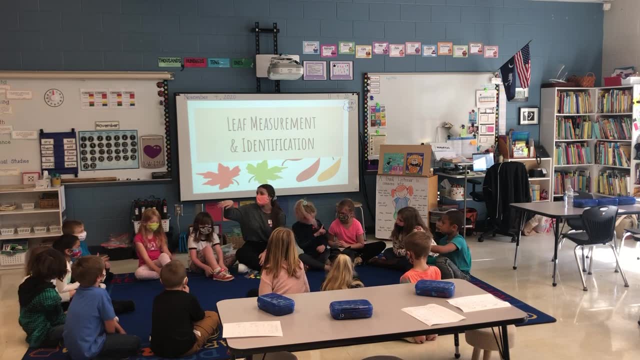 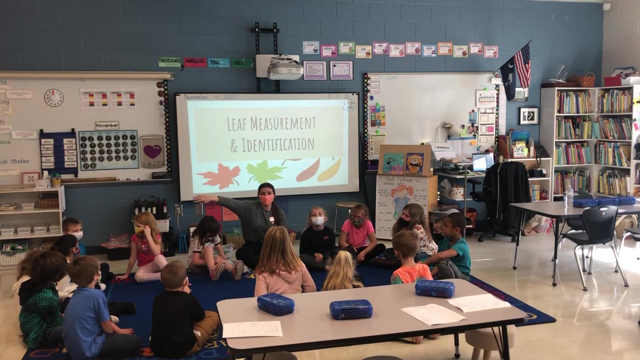 in just a few minutes. Yeah, actually Wakely. you kind of just: yeah, we're gonna do partners, but so you're gonna use like your table partners. okay, And so Wakely, since Zachary and you are alone. 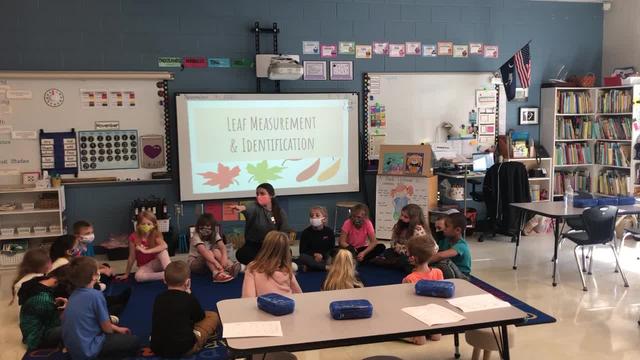 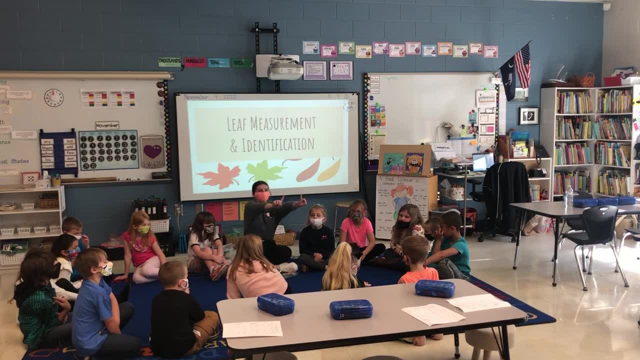 you'll be together. Bryson's not here today, so Chelsea and Ansley will be together- them two- And then you guys will be a group of three at the small table, And then Genesis and Noah will come together, And then there's only two of y'all today. 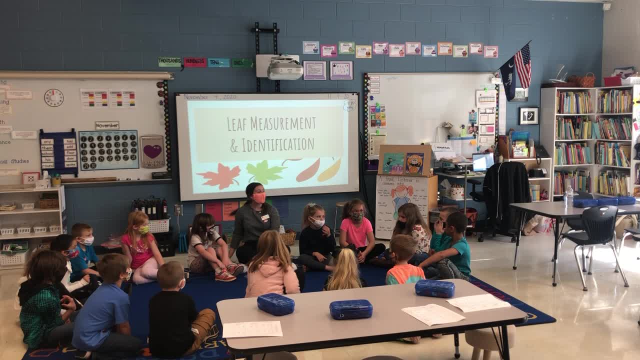 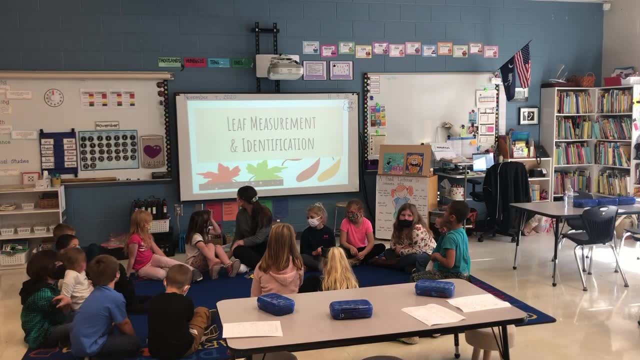 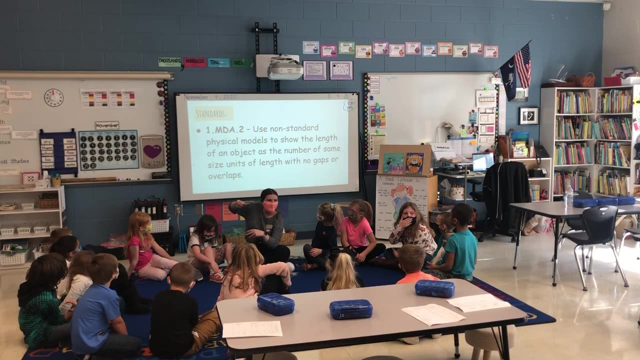 And then there's all three of you guys today Mask up, Mask up And mask up, because you are with partners. Okay, so today, our objective and our standard is using non-standard physical models. What is a non-standard? What would that be? 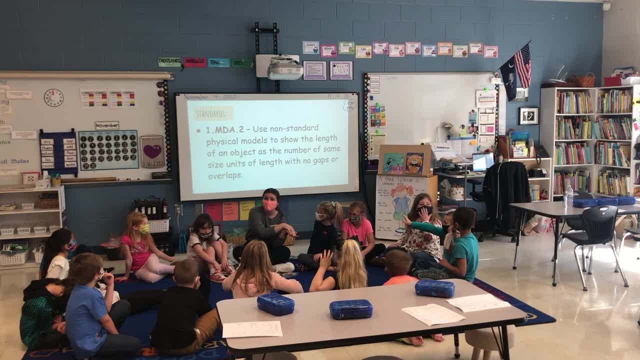 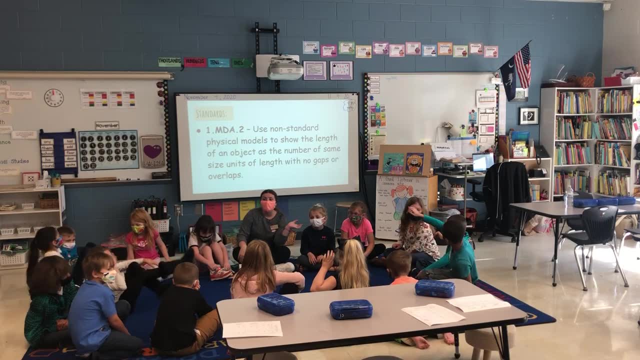 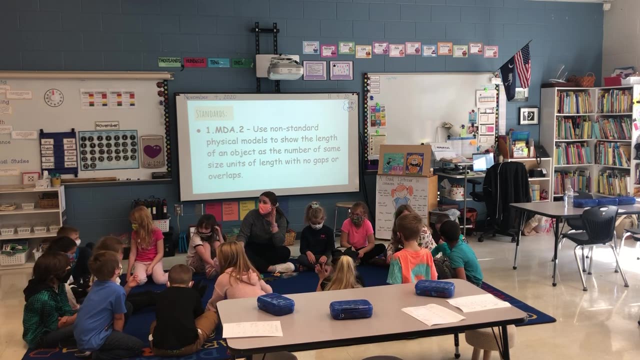 Or do you want to just tell me what a standard is? Tell me what a standard form of measurement would be first. Does anyone know what that would be, Jackson? what would a standard form of measure be The right thing? Do you want a little help? 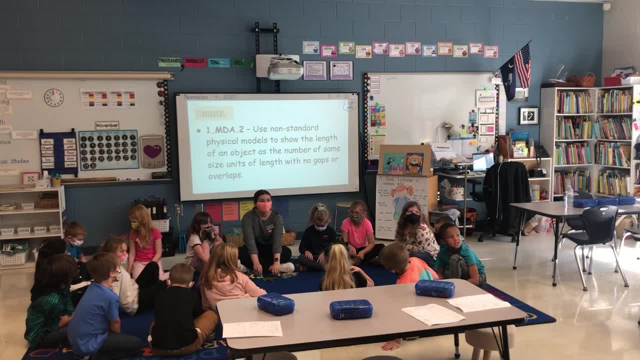 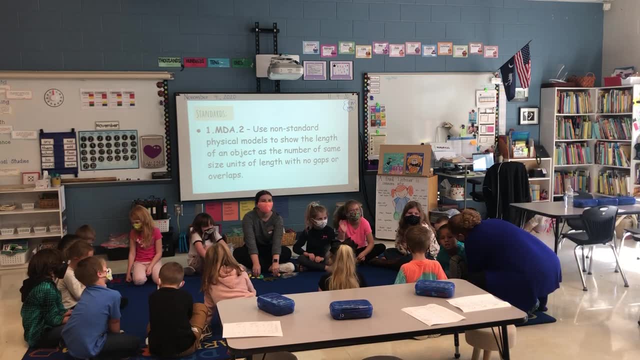 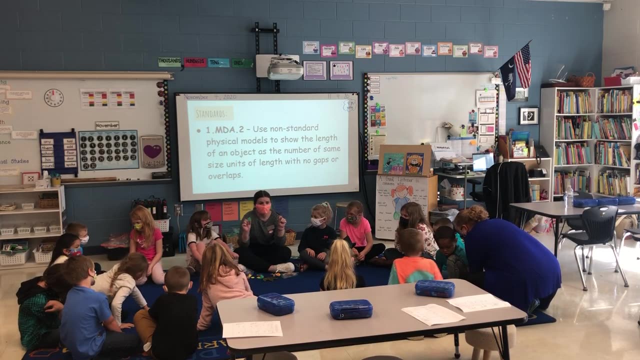 Or Amira. do you know what a standard form of measurement is? A standard form of measurement is something that is measured and it's Like you measure something. Okay. So I'll tell you what the non-standard form would be. These are non-standard forms of measurement. 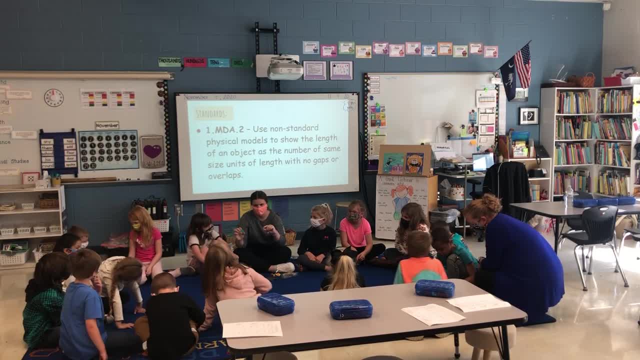 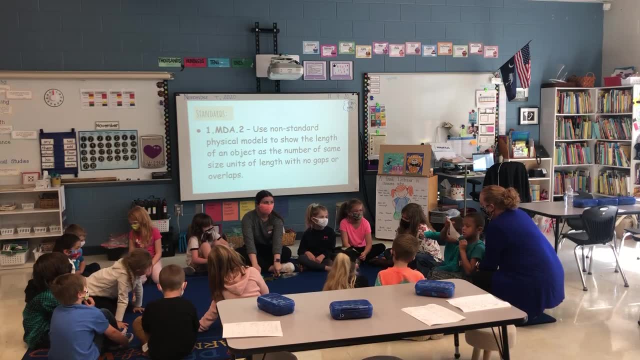 So, using these as the non-standard, what would be a standard form? A ruler, Carly Sue, a ruler would be a standard form of measurement And you can put it on the side of the week. So we're gonna use a non-standard form of measurement. 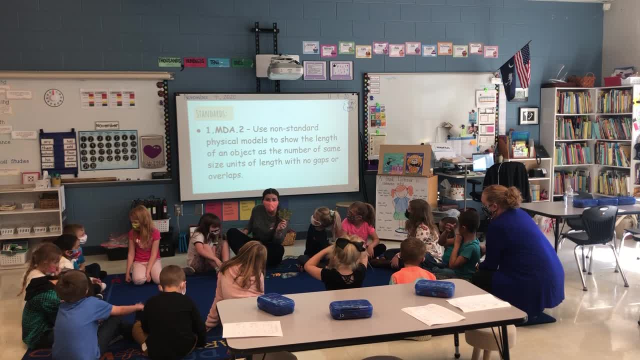 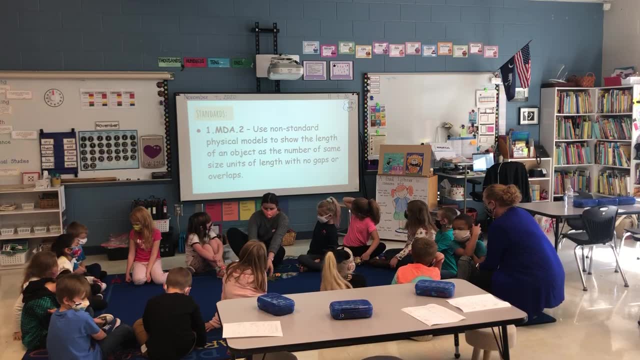 to show the length of an object, And our object is A leaf. A leaf, Same size units, The same number of size units and length, With no gaps or overlap. So do we line them up or do we put them far out? 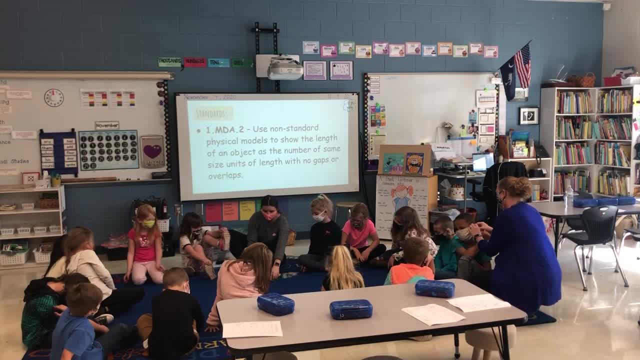 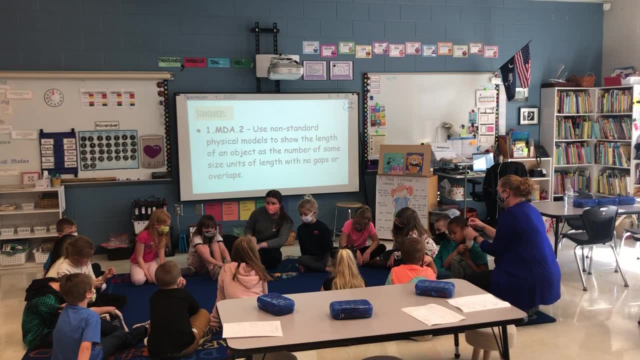 Yeah, We line them up. We line them up, So that means there's no gaps or overlaps. Wait, should we put them on top of each other? No, No, No. That means that you just have overlap, An overlap. 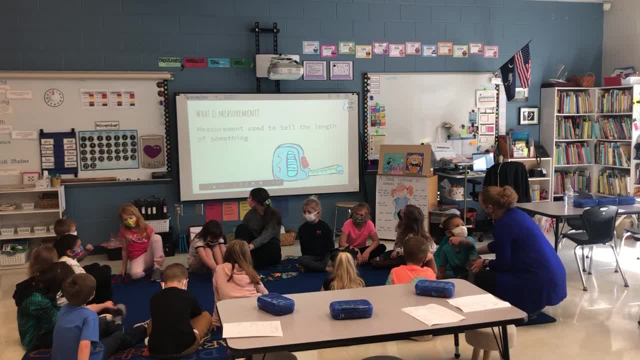 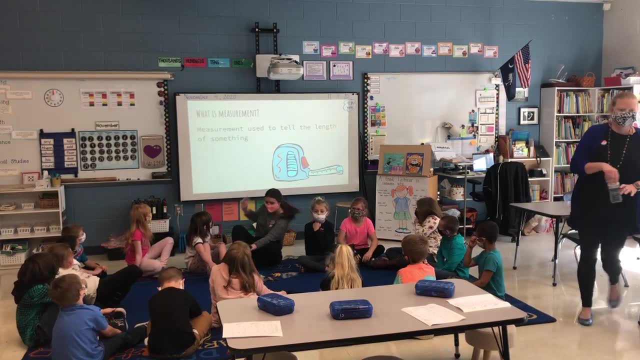 Yep, An overlap instead of what you actually need to do. Yes And then. And so what is measurement? Measurement is to tell the length of something, And so what are we using for our measurement? Candy corn, Candy corn. 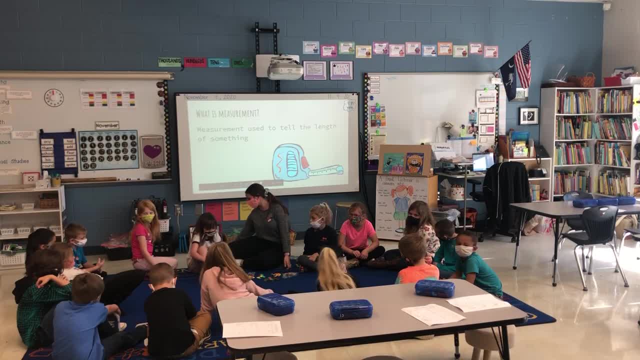 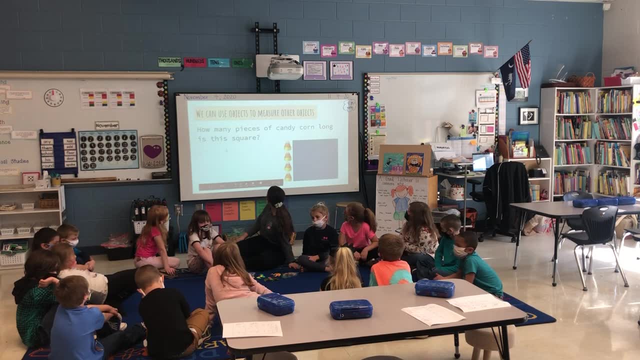 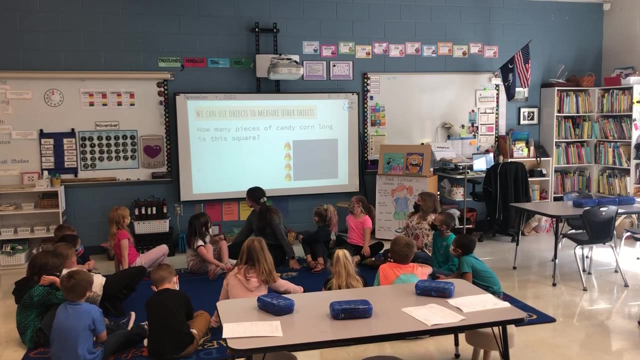 We're lining the square tiles to measure the length of the leaf. Okay, And so how many pieces of candy corn long is the square? Four, Four, Four, Four, Four, Yep Four. And so then we're going to. 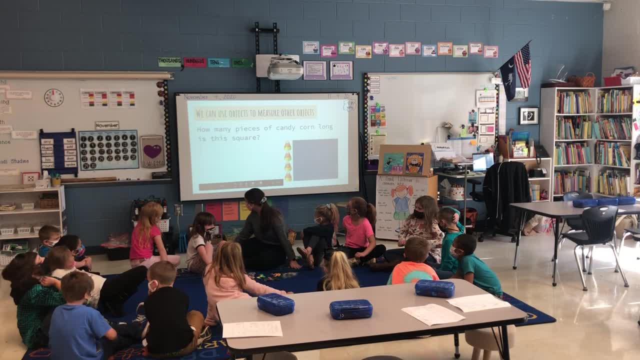 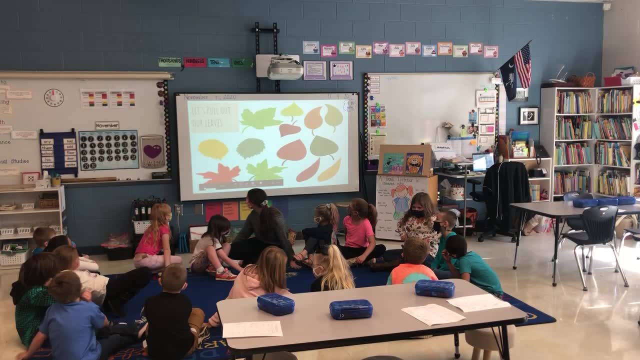 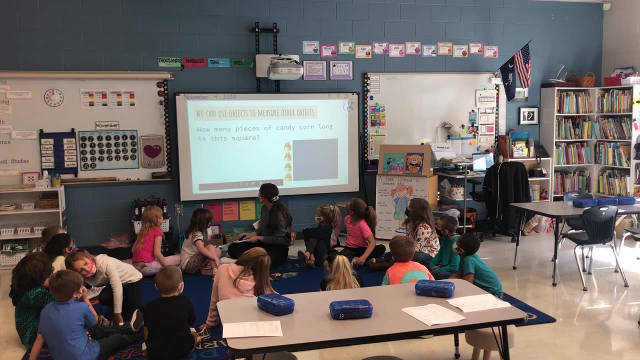 Sorry, This is hard to use the mouse. Oh, Oh, my goodness, You guys. what's up? It's being a little cantankerous today. It just doesn't want to do slide five. It's being a little loppy. 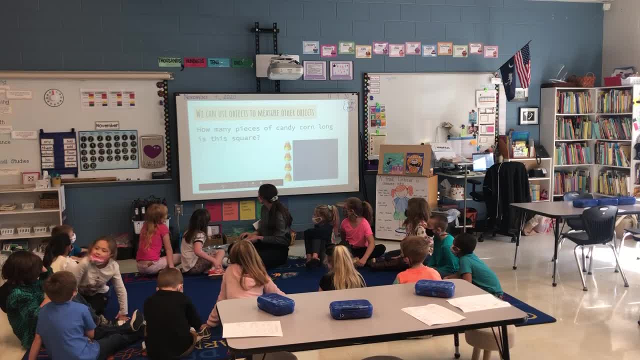 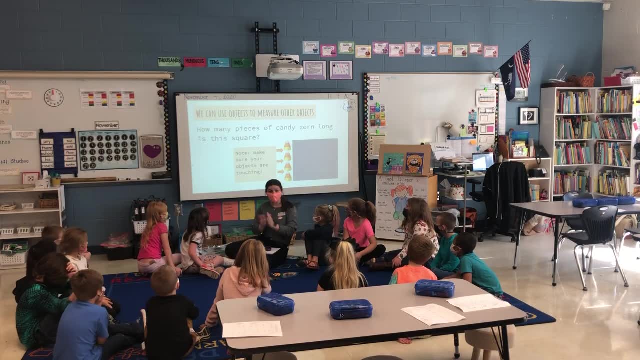 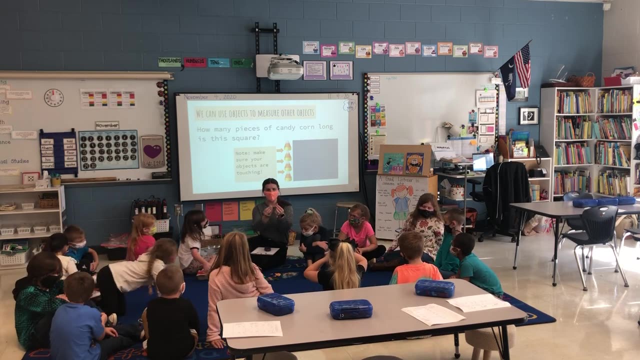 It is. It's okay, We'll get the-. We'll be flexible, Yep, Okay. So we're going to remember not to put any space. You got it Okay. So we're going to make sure that they're touching. and what else do you think they should be? 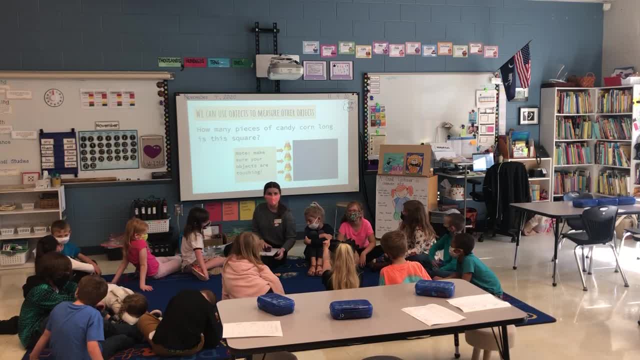 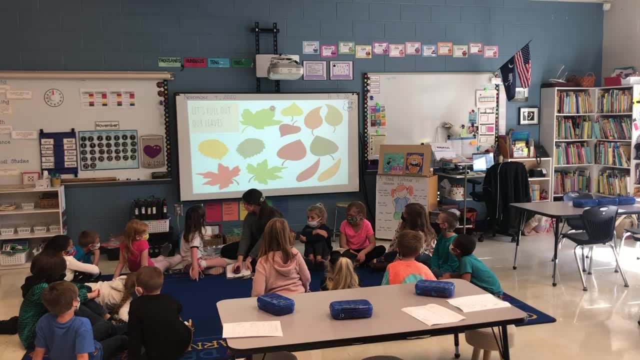 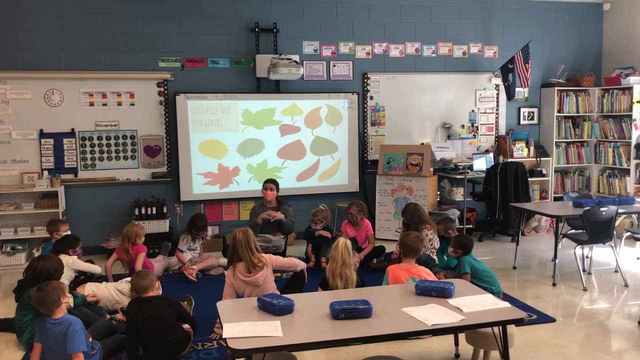 The same way or the same direction. Yep, they're all the same way. Okay, so I'm going to hand you your leaves again, and so then you're going to go back to your regular tables and you're going to work in pairs or partners or in a small group. 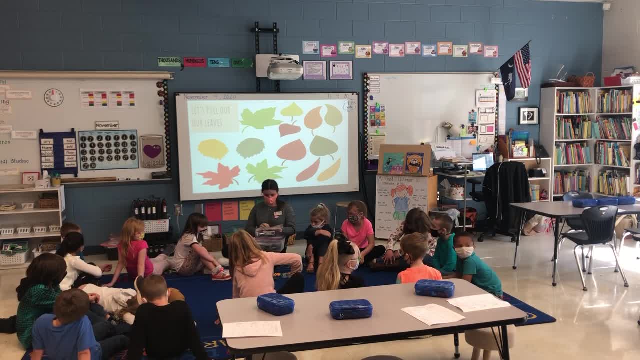 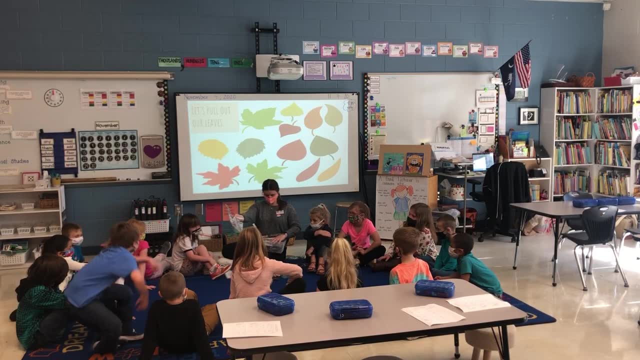 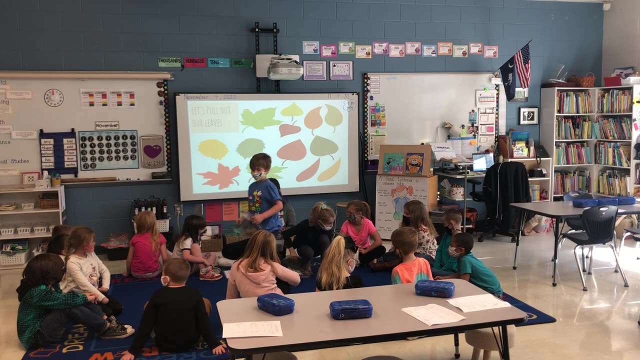 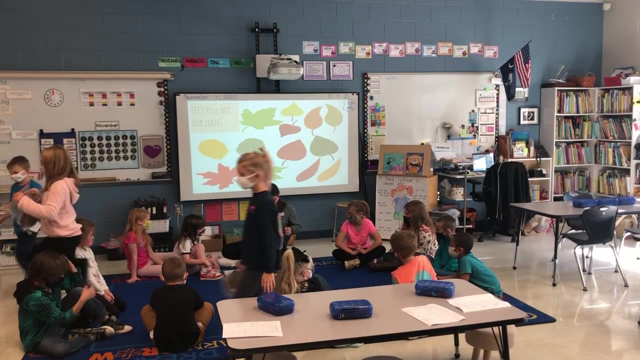 with the people at your table. Does that sound good? Yes, Okay, This one might be in Aspires because there's your name: Jackson Ansley, Zachary Wakely, Bryson Weston, Carly Sue Amira. 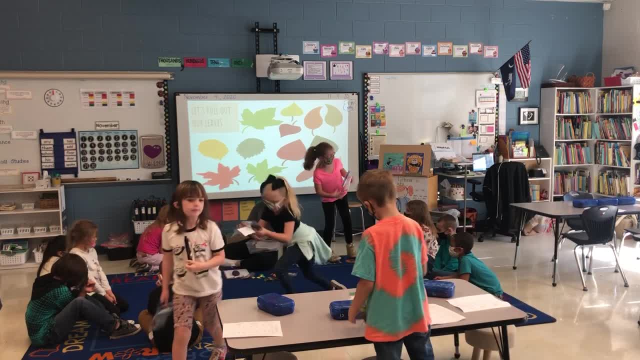 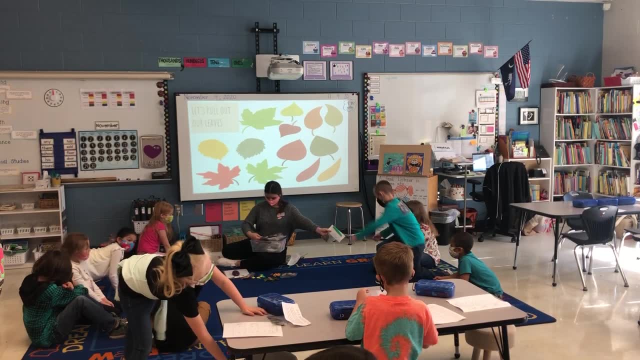 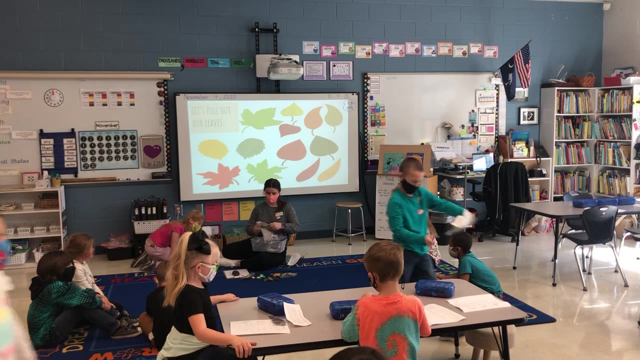 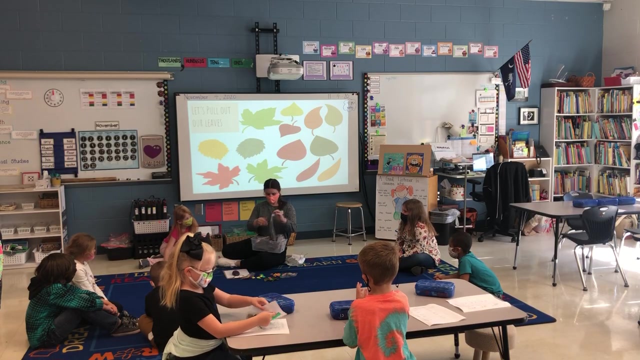 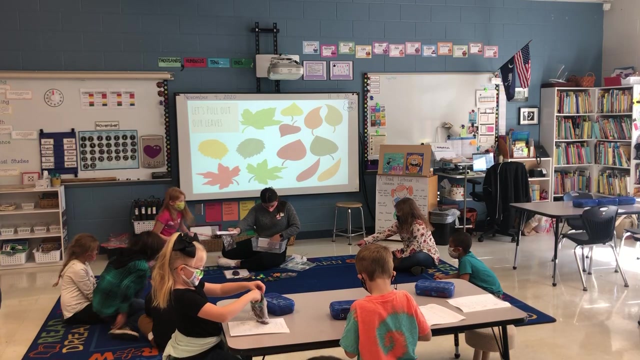 Ellianne, What Weston or Brown Noah, I'm going to put 10 points. Paul Davis- Timothy's not here. Julian Justin, W mnie nie teklar. Oliver Elijah, Ingrid B, finances, Kareem. 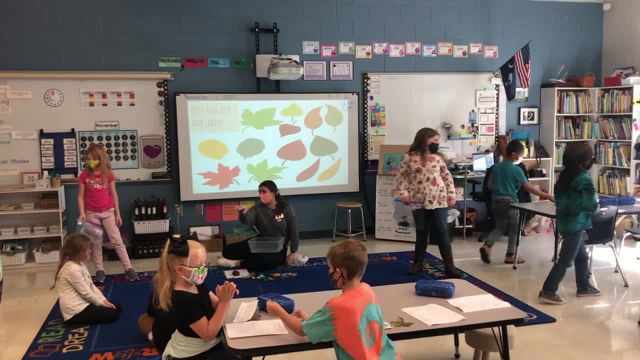 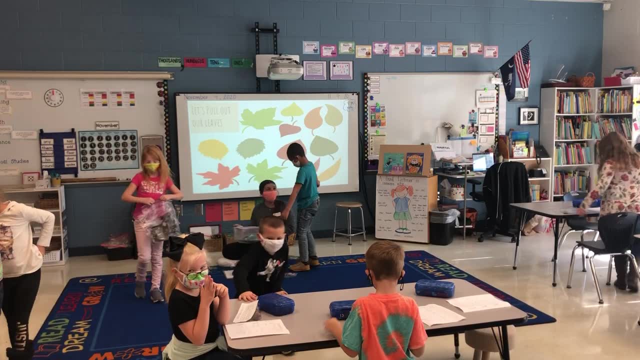 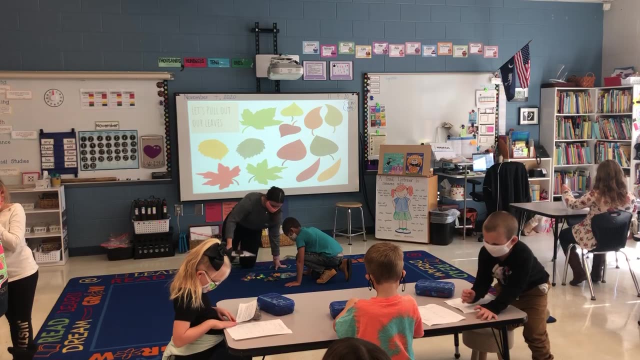 Kareem nenhum. Isaac Kareem, nothing. And then Walter Andrade, Ostos Hagrid, whilst Audrey Regula Melissa And lisa Teresa, Matthew пальato Alberto. Okay, so, ladybugs, do you see that sheet in front of you? 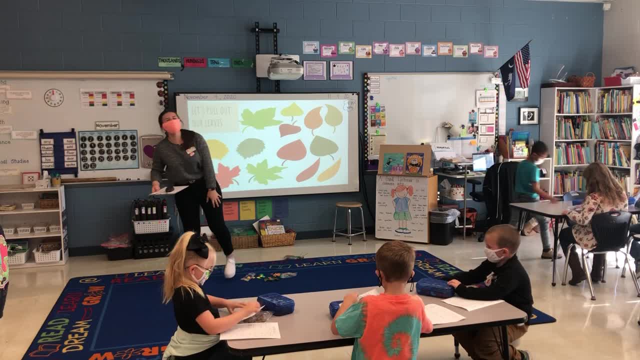 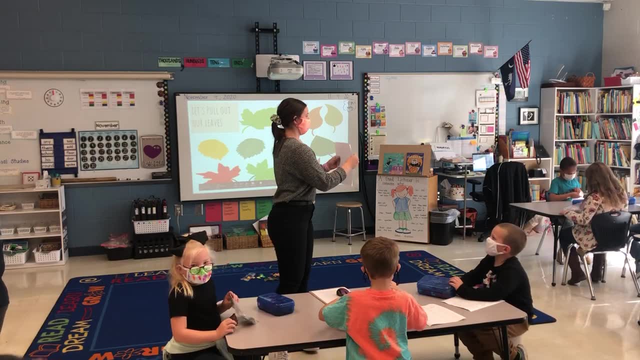 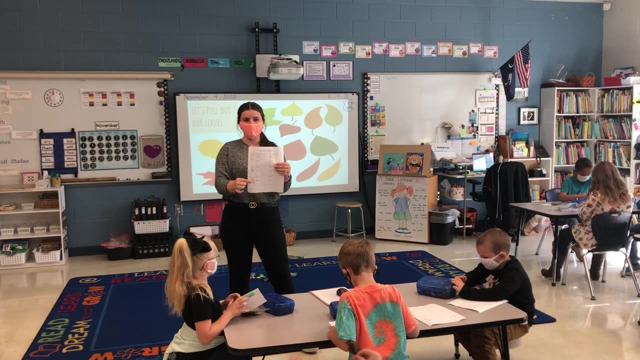 Yes, Okay, I'm going to borrow Amira's real quick, And so can everyone look at their sheet, Okay, so on this column we see that it is labeled small, medium and large. So how did we say that we're going to define the shape of the size? 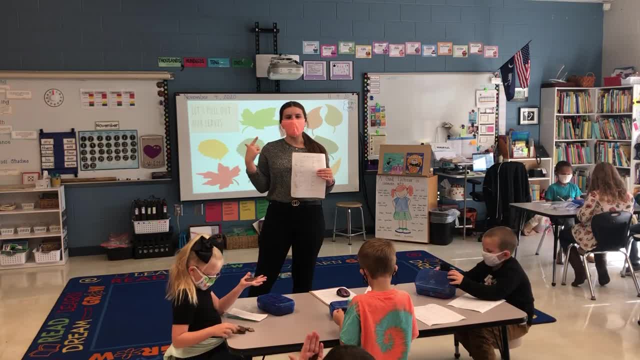 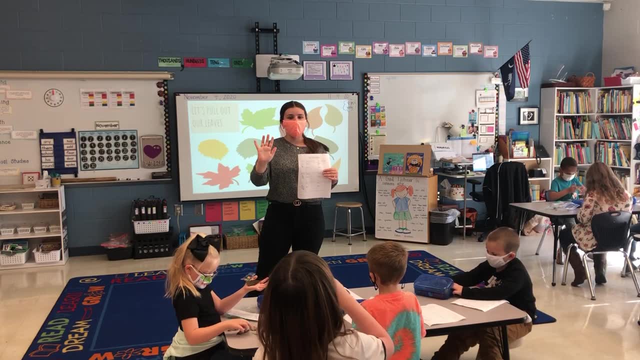 By hand By hand. So, Carly Sue, can you remind us how? if it's what? If it's smaller than the hand, I mean that it's small, But if it's about the same size, it's a medium. If it's bigger, it's a large. 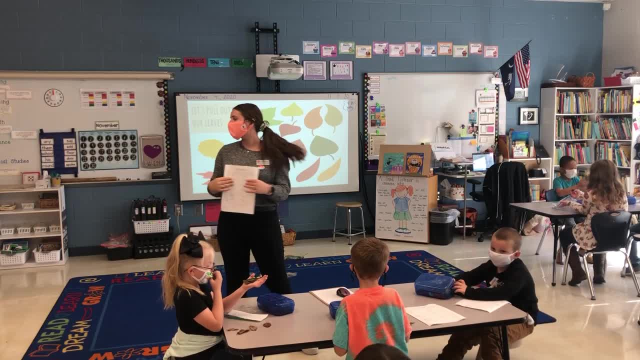 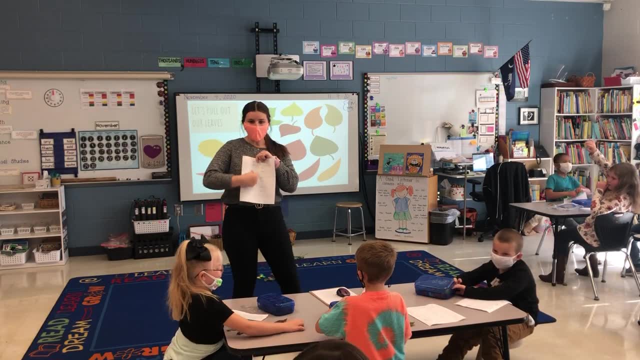 If it's bigger than the heart. yes, Thank you, Carly Sue. So what I want you to do on this sheet of paper is you can see the number of square tiles on the middle column and the number of candy corn on the bottom. 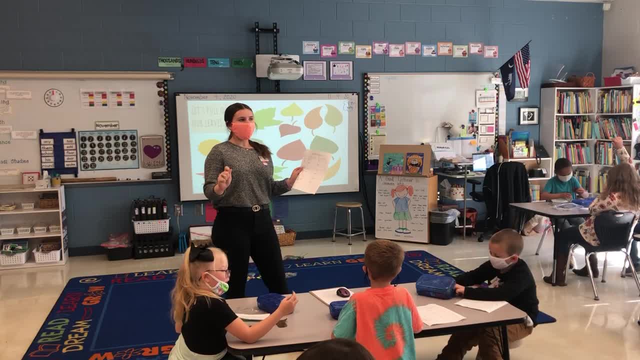 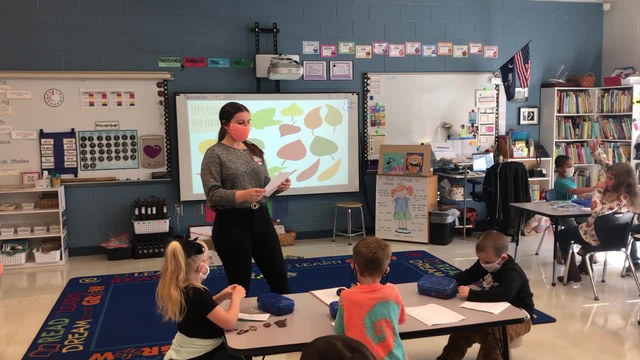 Right column, And I want you to write how many candy corn or square tiles it takes. and we're going to do both. okay, So can we remember? back to our leaf down there, What would we write for the number of square tiles? 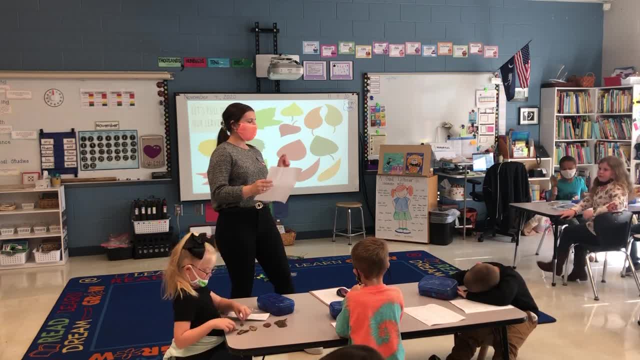 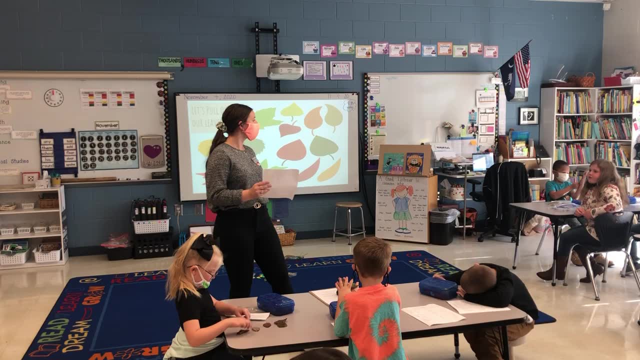 Reagan Reagan, what would we write for the number of square tiles? Number of square tiles. you might remember how many square tiles you have. Yeah, how many of that leaf of square tiles do we have Four. We have four. I think we might have had one more. 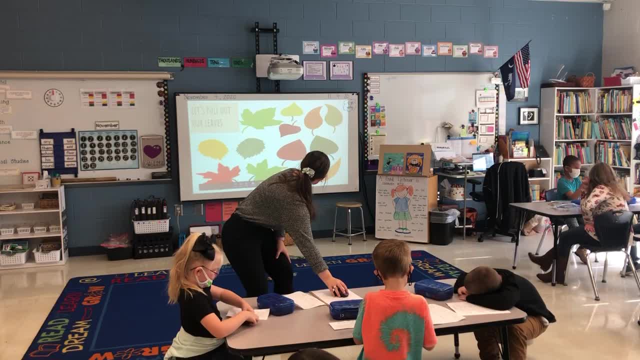 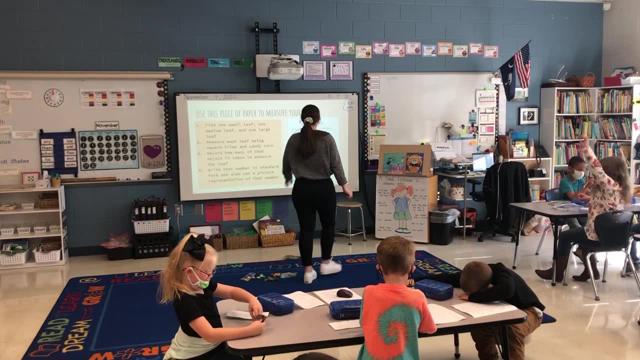 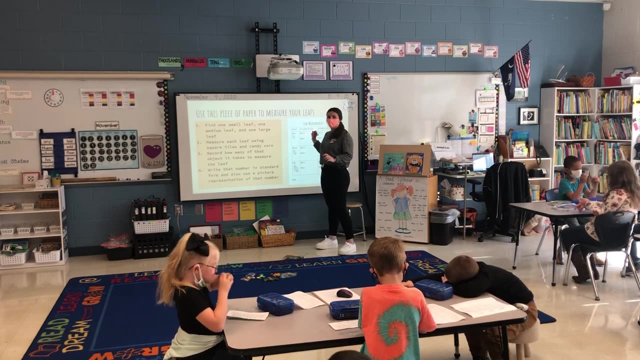 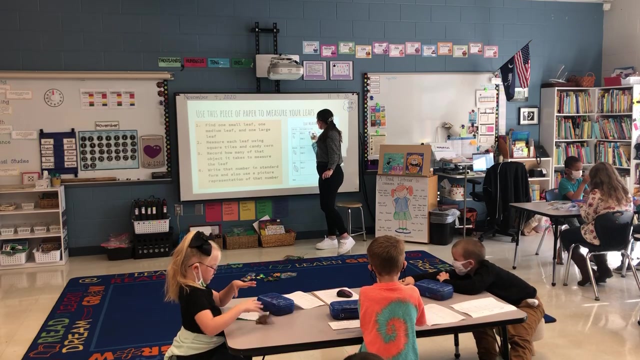 Five. So what we would do is: let me okay. so Reagan reminded us of our square tiles long We had five. So, Lady Bucks, can you look over here, Thank you. So I'm going to write five and then I want you to draw. so how many would you draw? 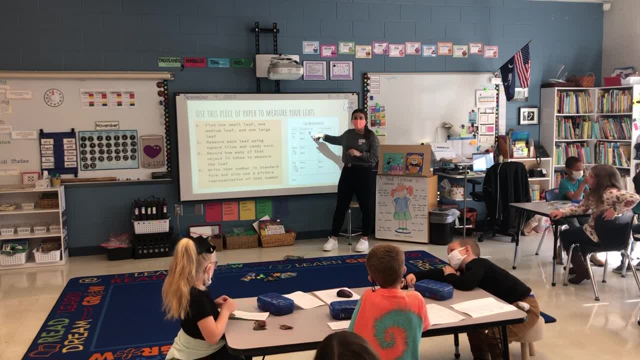 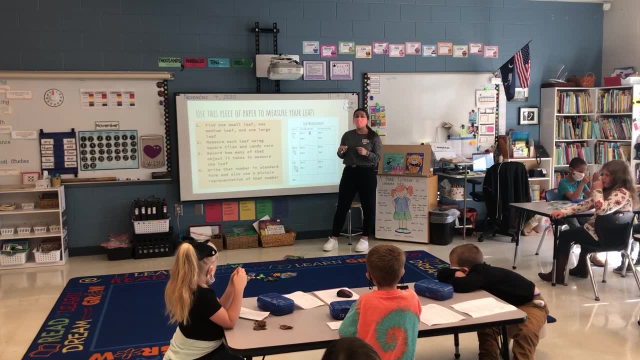 One One, One, Five, Five. So what do you think would make the most sense of what we would draw? Five leaves, Five leaves, Five. Five tiles, Tiles, Five. what kind of tiles? Square, Square tiles, Okay, 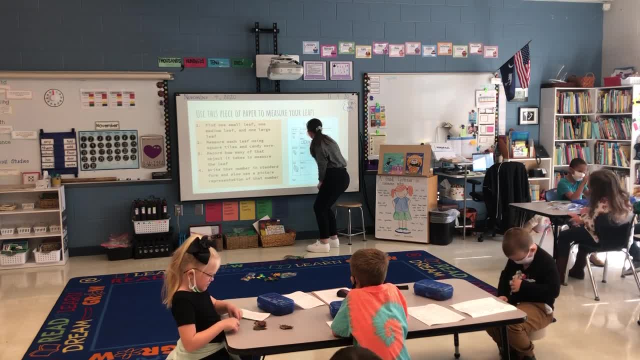 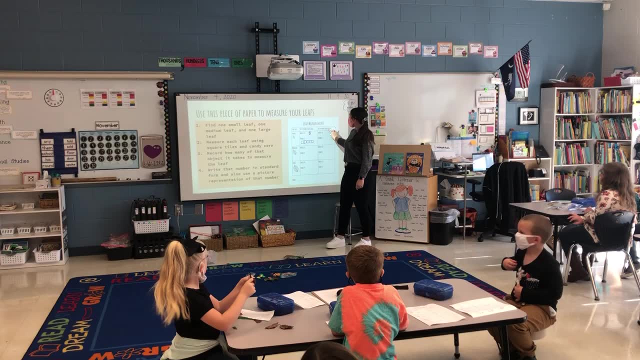 So I'm going to draw one, two, three, four, five. Oh, I'm sorry that was for our medium leaf, but it's okay. What about how many candy corn long? That's six. That's six, That was six. 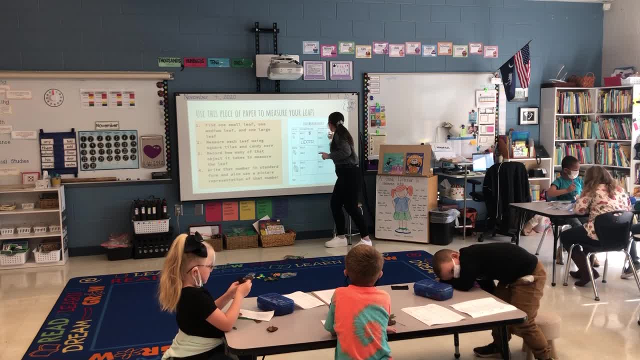 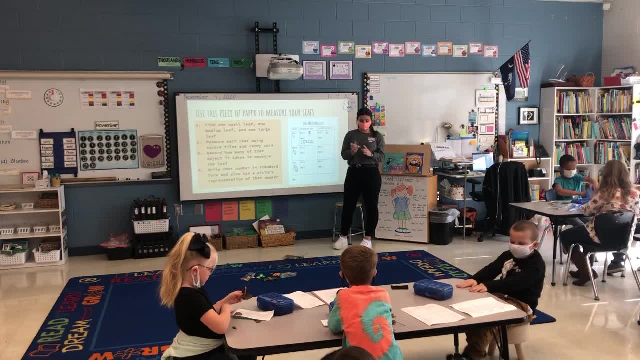 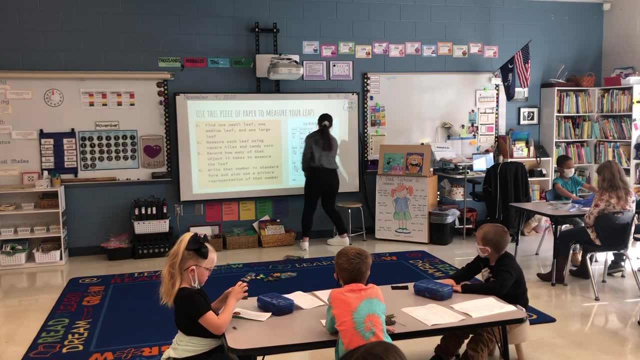 should we draw Candy corn, Draw, Draw candy corn. Should I worry about the colors and stuff? No, What could I do? Just draw it, Just draw it, Just draw it. It's too perfect. I'm going to draw like: what kind of shapes do they look like? 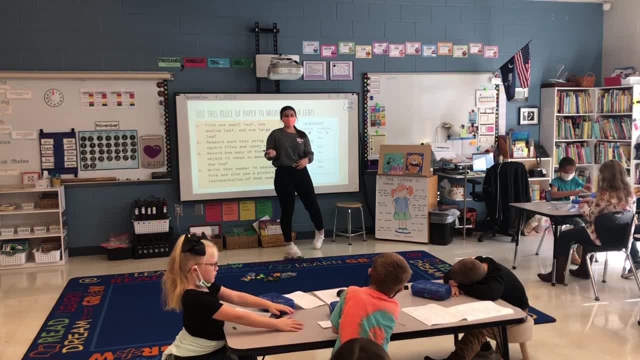 They look like a triangle that has curves. Yeah, it looks like a triangle, So I'm just going to draw a triangle and we'll represent that as the candy corn Kelly, and that shape has a name: that's called a curve. 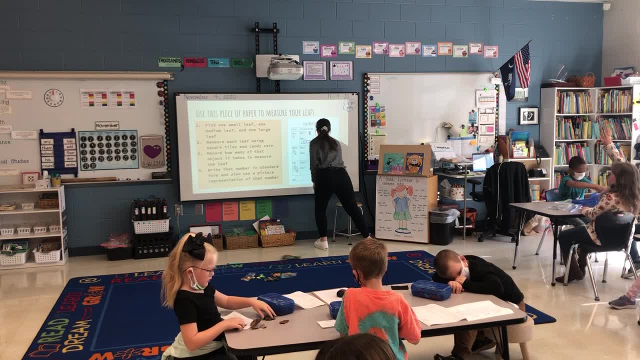 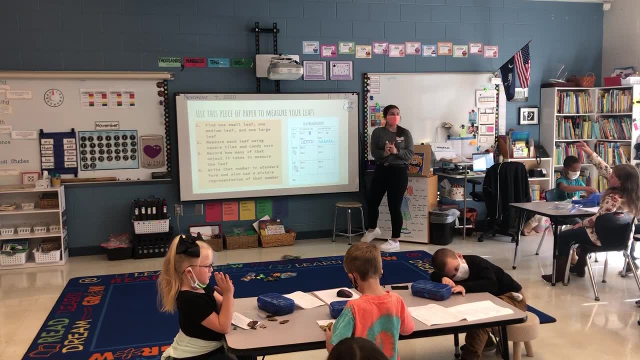 You're going to do a triangle, Okay, Okay, that's what it's called. I expect curves like that. Okay, ladies, does that make sense? Yes, Just a bridge of a triangle. You can just use a different one. 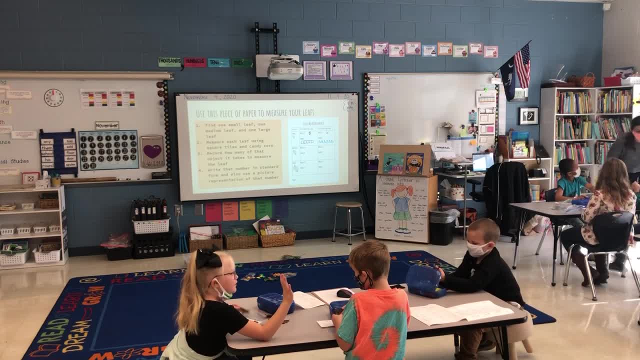 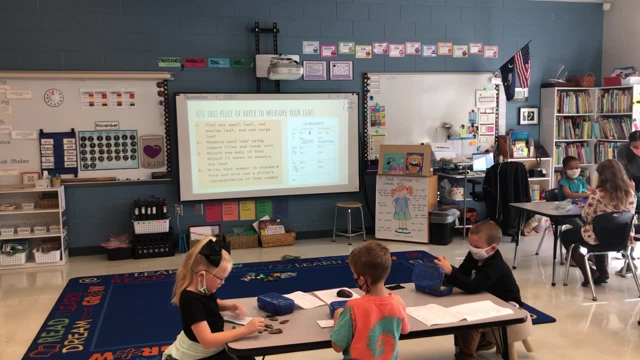 All right. so what leads you to the first one? What Small Can I see? if there's a small, There's a small. So maybe this right here. Okay, just one, One at a time. One at a time. 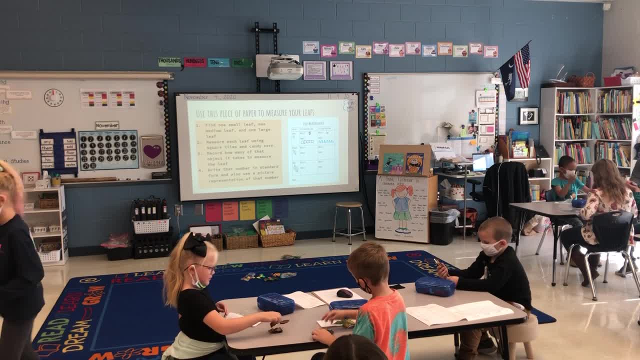 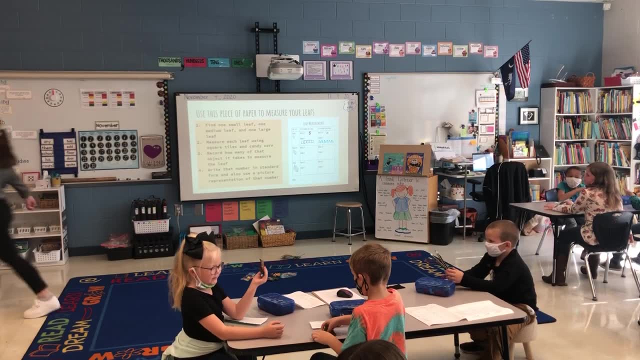 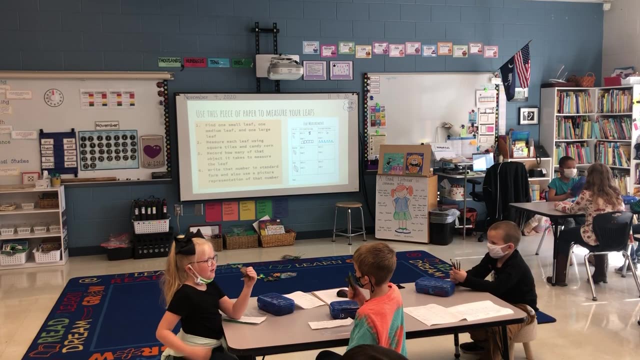 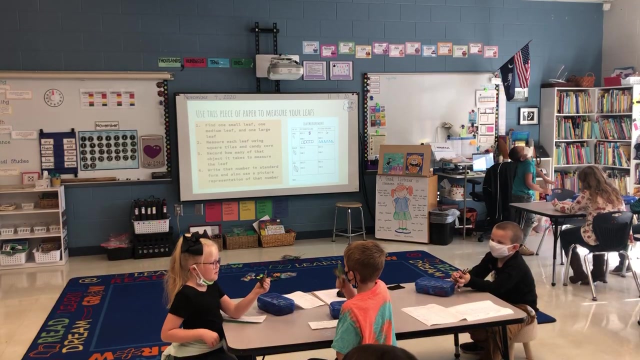 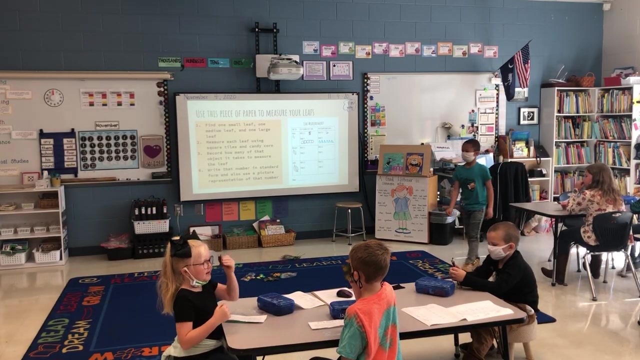 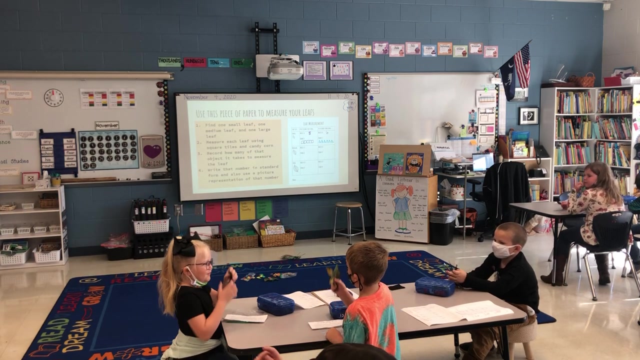 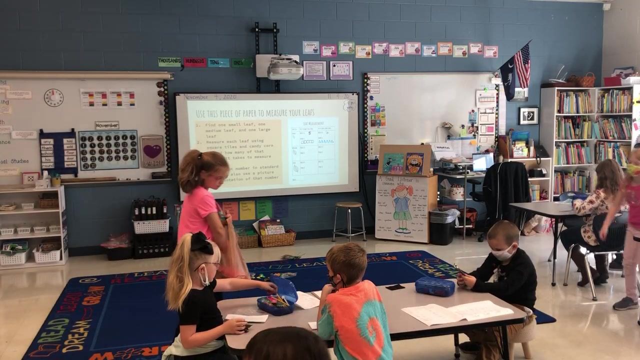 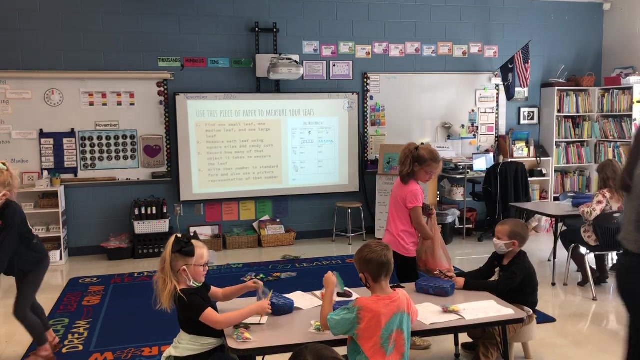 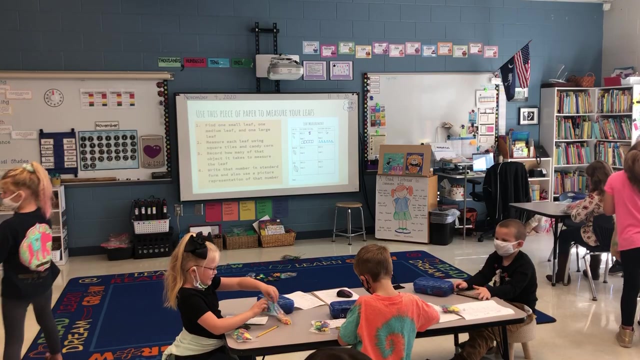 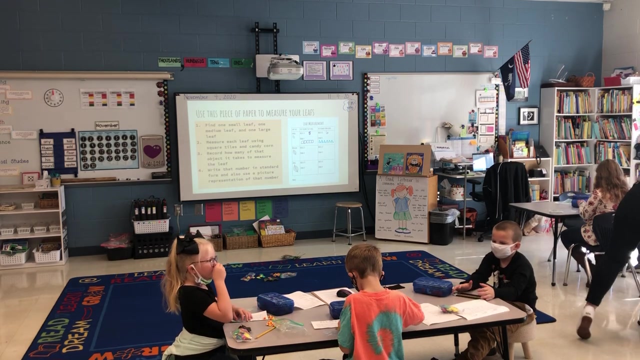 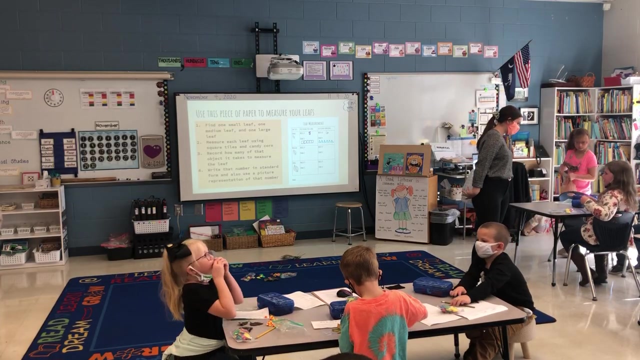 One at a time. Okay, so where are you going to measure it first? Alright, so we'll get one small mass. Andrew, come on, I'm sorry, I need to do this. So what leaf are you starting with? Alright, so, ladybugs, you need to pick your three leaves. 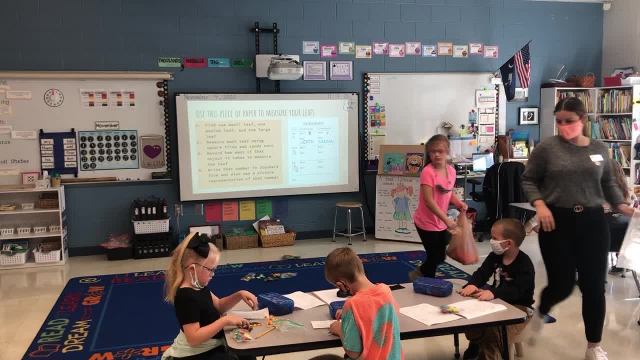 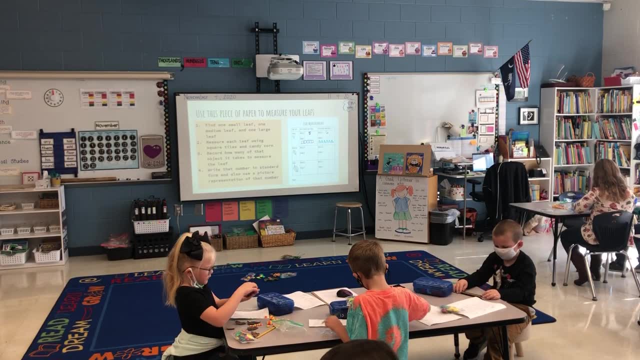 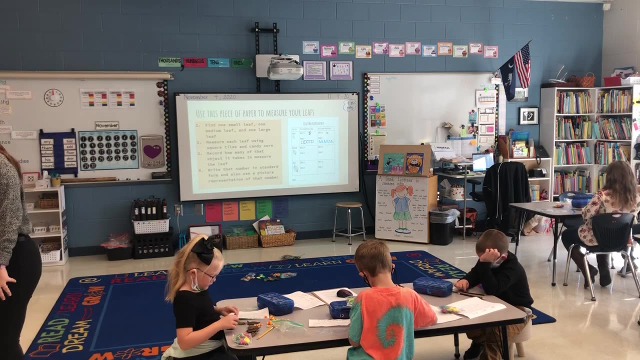 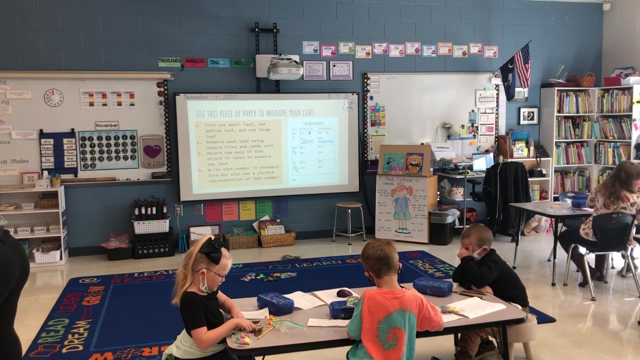 Your small leaf, your medium leaf and your large leaf. Okay, that way you've got them. Go follow me and point us along. Okay, so write it and then draw it. I'm going to take two. I think it's all of them. 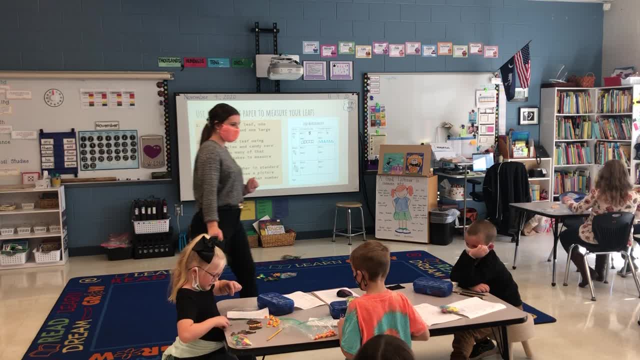 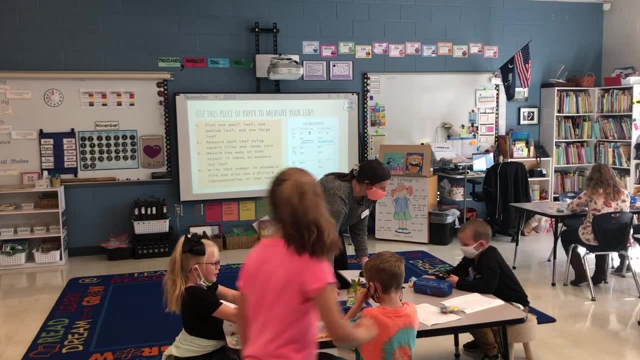 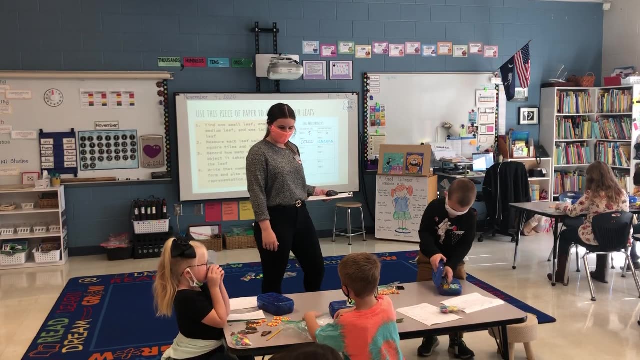 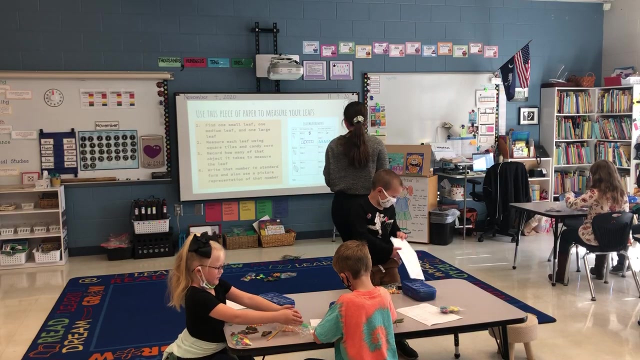 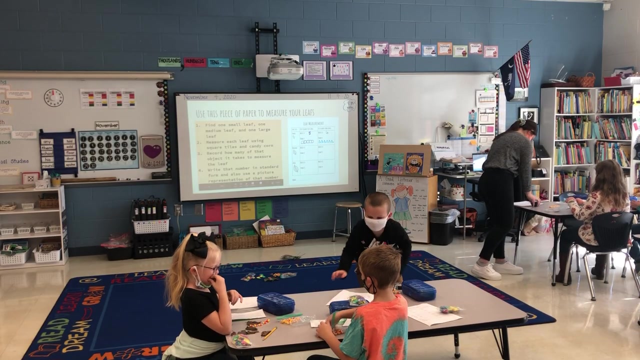 No, that's not all of them. There you go, Jennifer. So where's your small leaf? It's your small one. you measured with your candy corn. Now, let's measure your small leaf first, Now your small one. 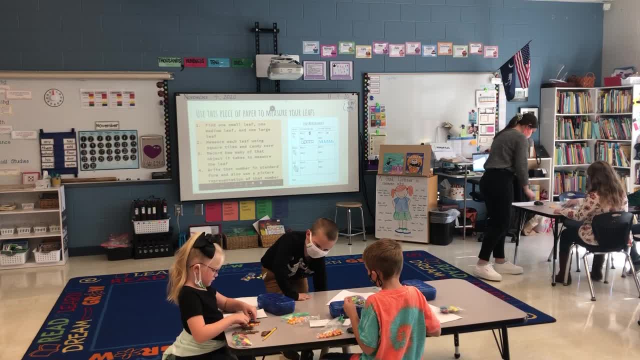 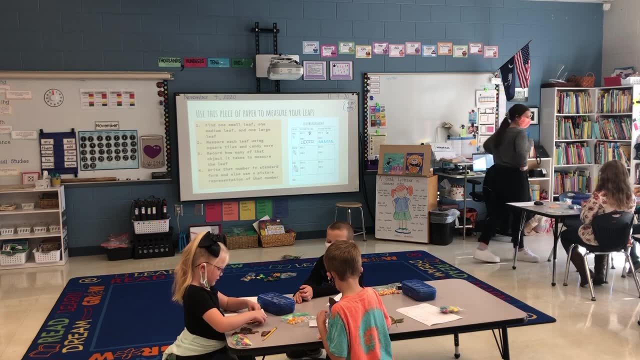 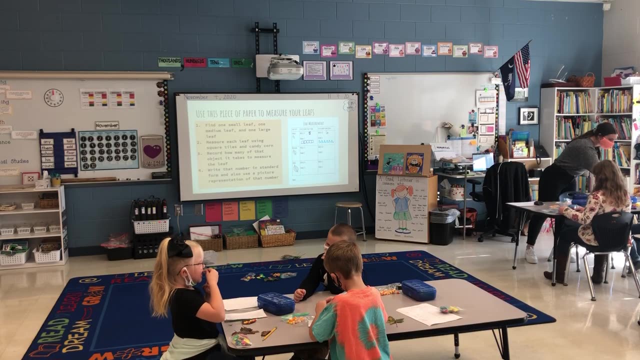 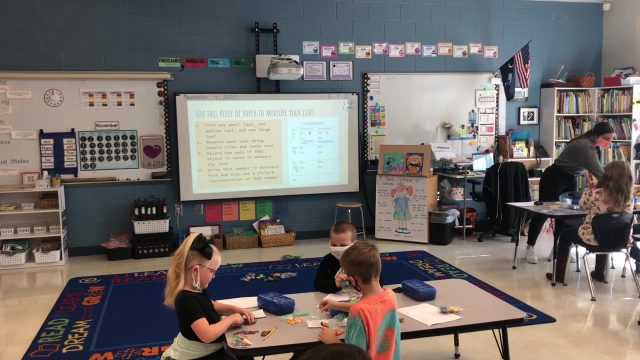 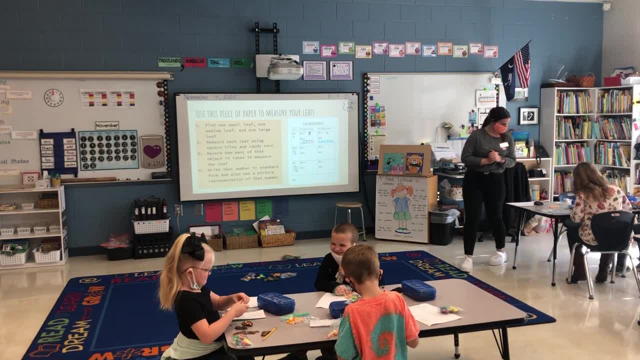 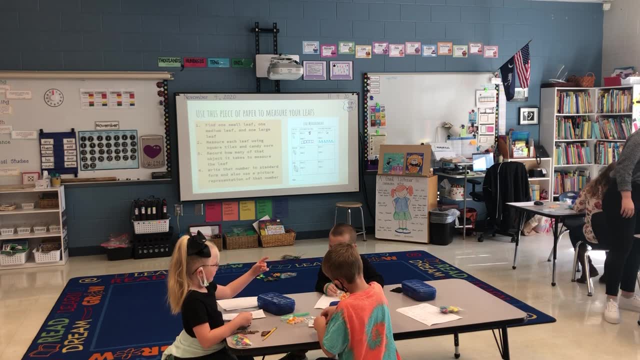 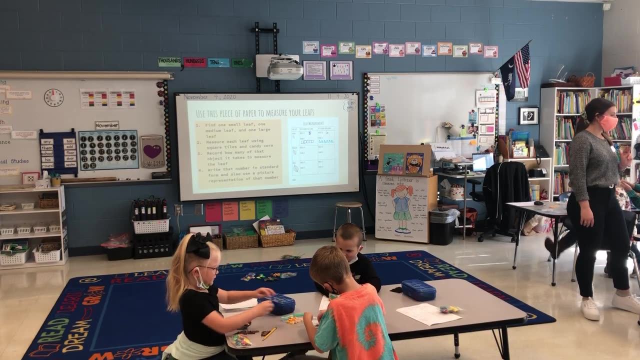 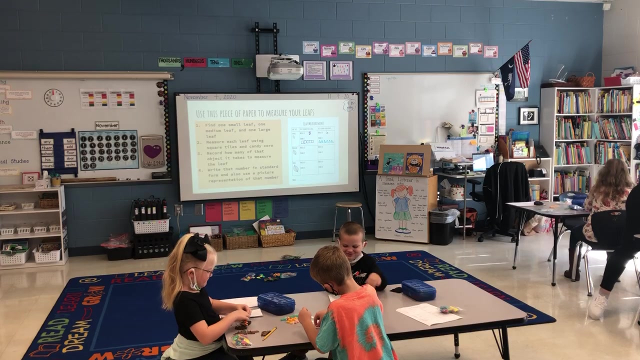 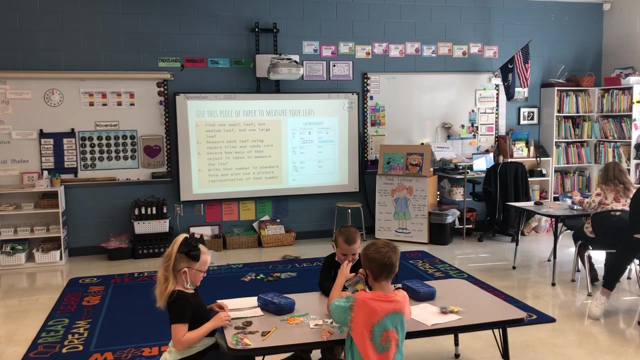 Write that number and then draw it. Find your medium leaves. Which one's your medium size? I'm gonna put one coin in the middle And keep that Three blocks tall, Three, Wait, Show me what you're using. I'm gonna use a blue. 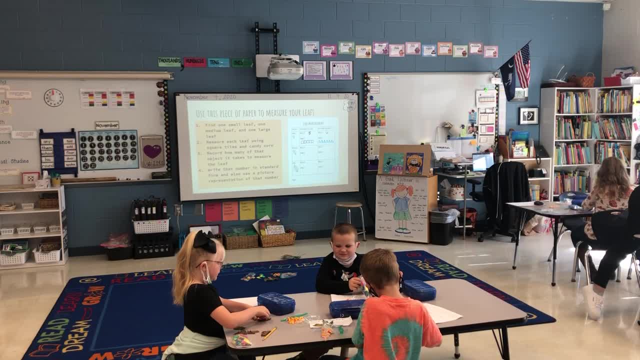 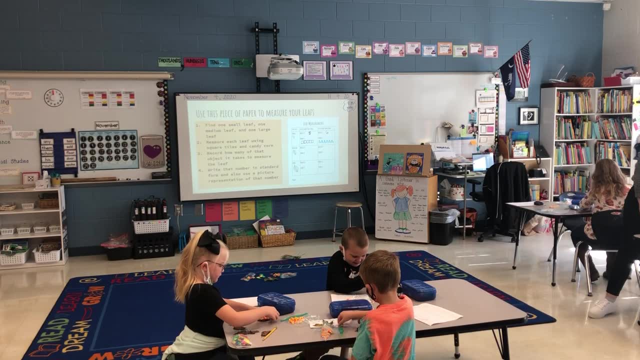 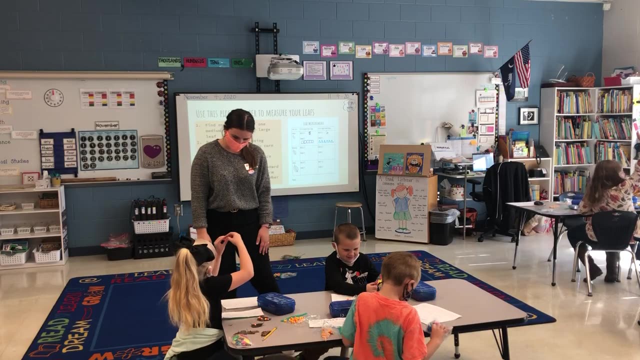 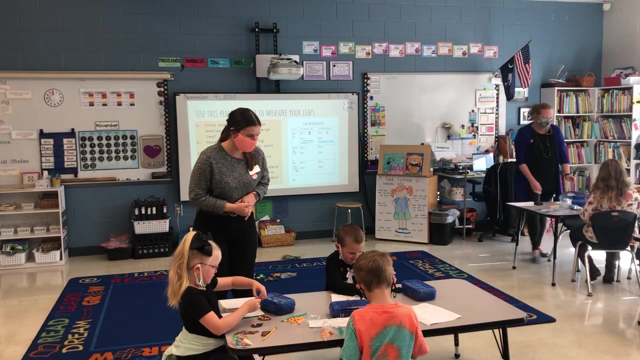 Blue is the prettiest color We'll see. Oh, it's candy corn, Ah, it's candy corn, Candy corn. Two, Three, Two, Three-square, Uh-oh. Okay, let's look. First we need to have what? 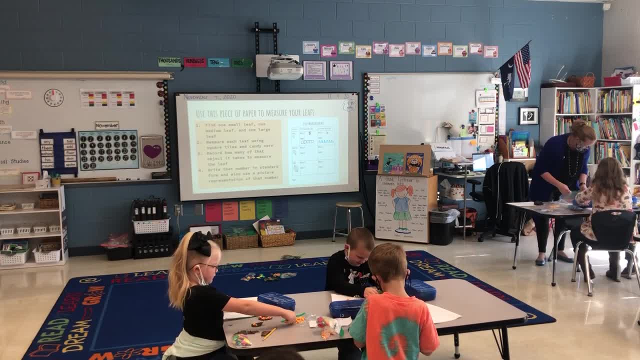 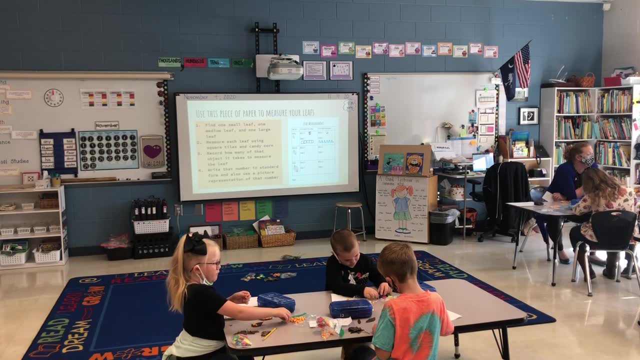 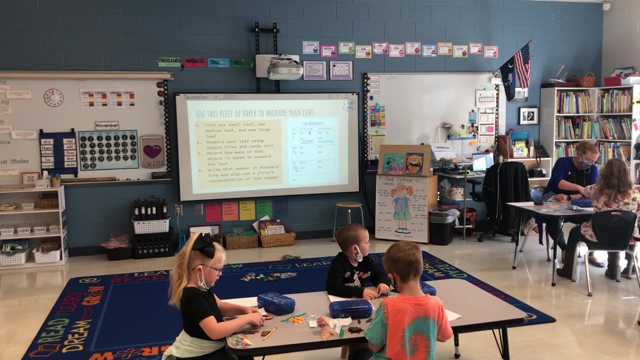 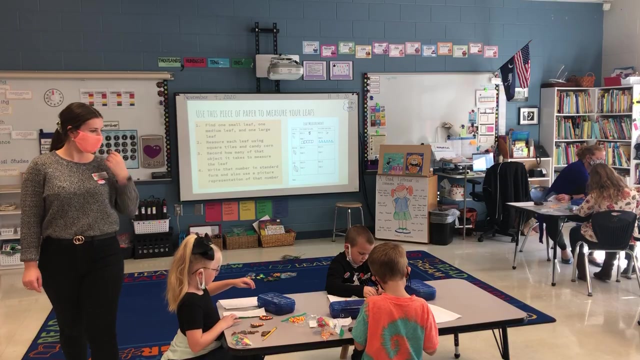 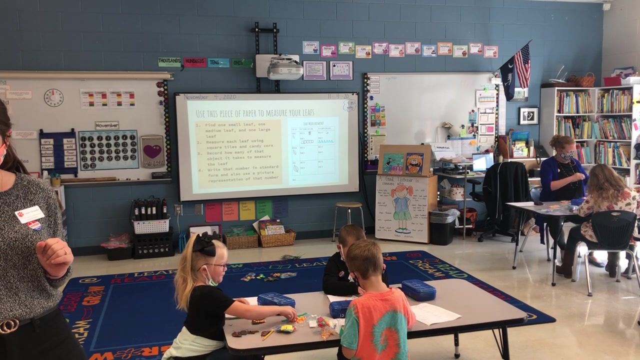 You got it. Let's start with that. Two How many dollars? You can't even ask for any dollars. That's right. That is a small one. My leaf can't hold it. My leaf can't hold it. Do you need help flapping it? 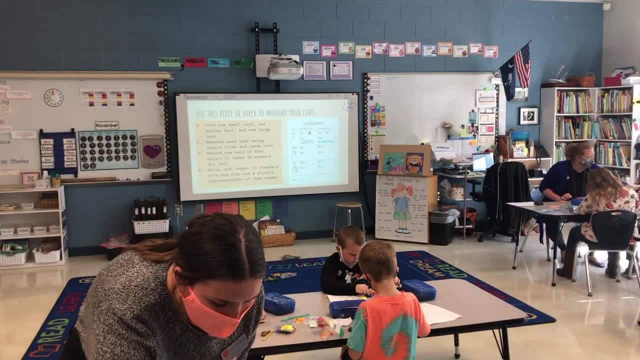 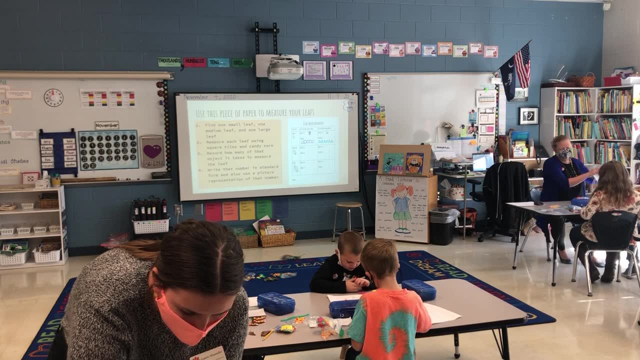 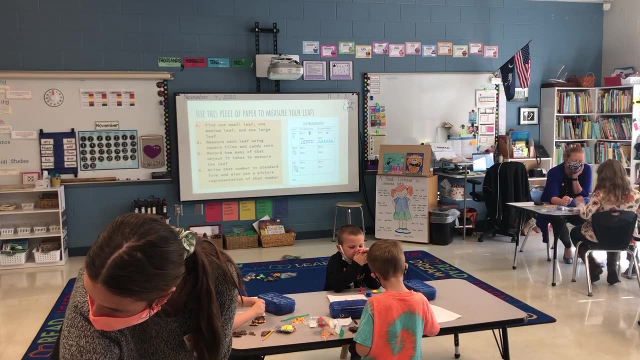 Do you want me to hold it flat so you can label it? Put the candy corn down. Oh, that is harder. Let's try putting it over like that. Oh my gosh, I'm sorry. Yeah, yeah, yeah, If it broke, just use a different one. 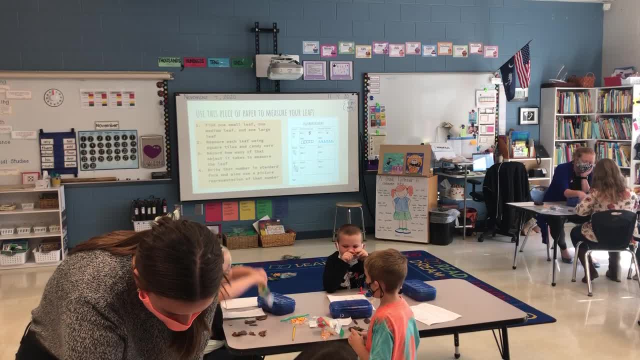 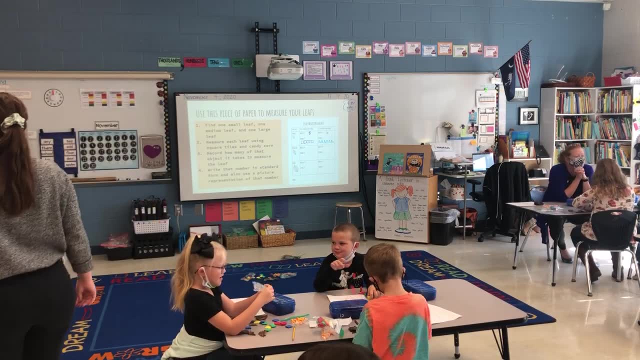 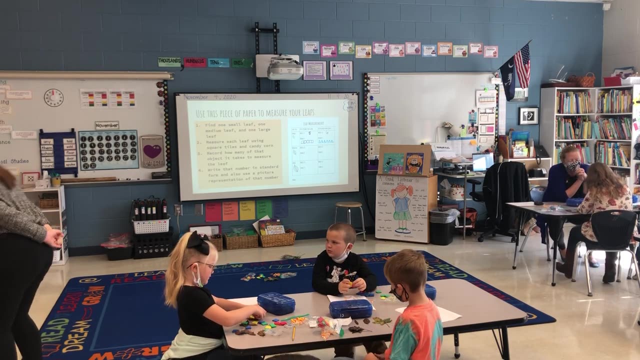 So is this your small one or your large one? Small, Okay, so you found two. Oh, so then it's three. Very nice, I got one. I got one. Thank you. Two, Two, You need to pull it down, You can just go check. 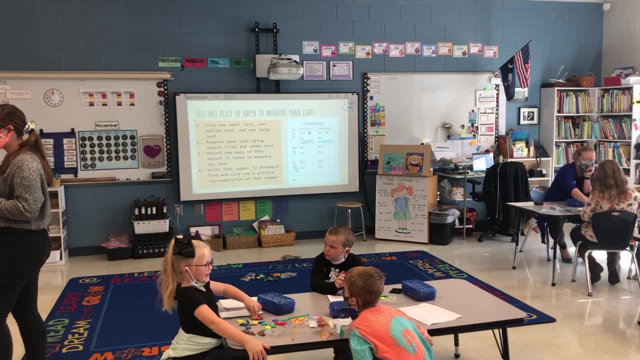 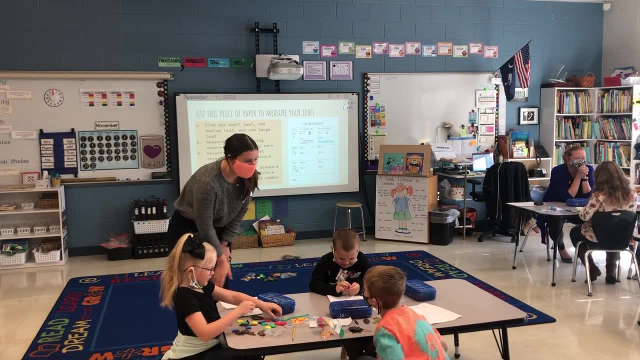 Let's not do that. Red Apple, Apple Apple, Cherry, Cherry, Grace, I got one. Okay, so can we record our findings now? Have you found anything? I said no. Can Remington have a leaf? 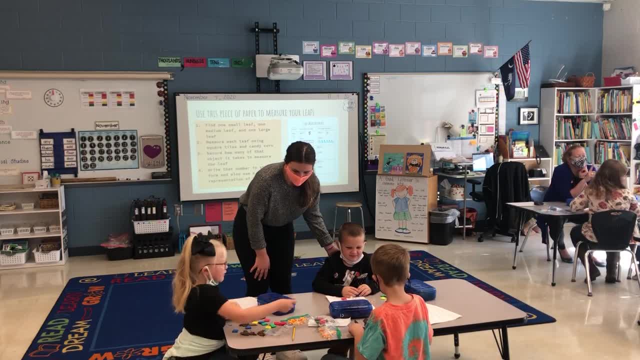 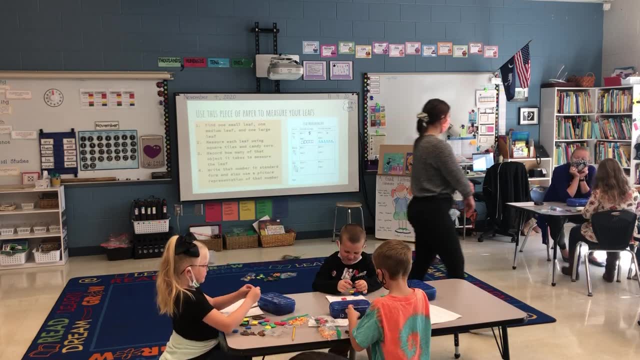 I can measure it. I think it might be shared. I can share this leaf. This leaf is about to come out. No, you need to pull it right now. No, it can't, Let's say it's not. Okay, so let's do a whole onion. 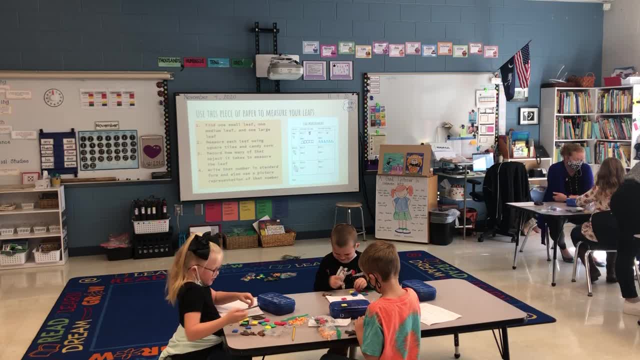 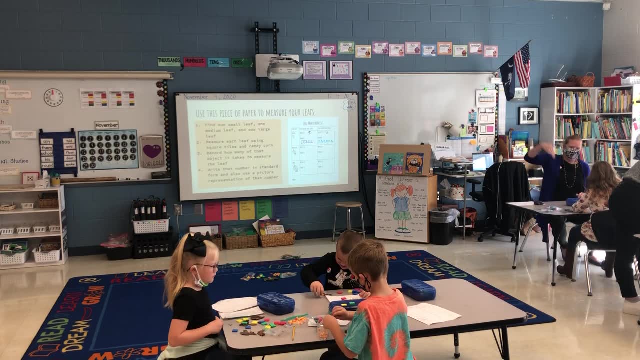 And put it somewhere else. So write it here. Yes, Can you write it too? Remember that about sign. Remember you talked about that Exactly And you put it somewhere else about I don't know. Um, no, I used it. 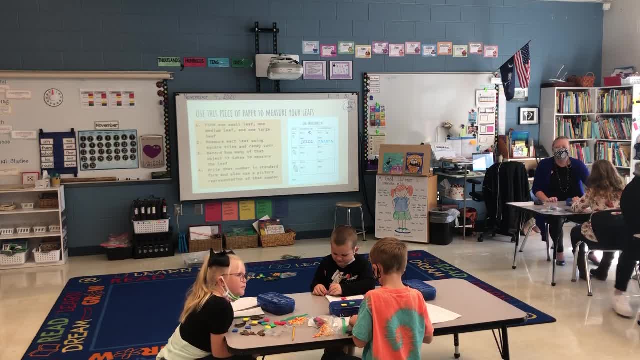 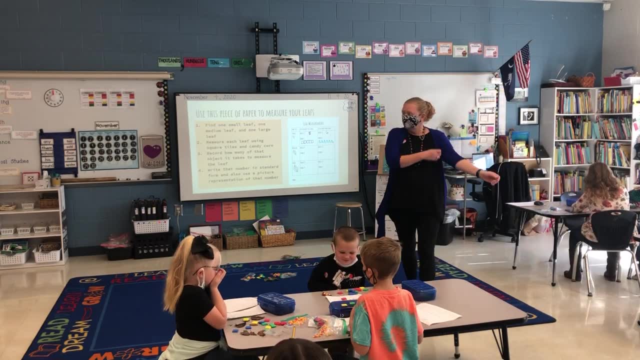 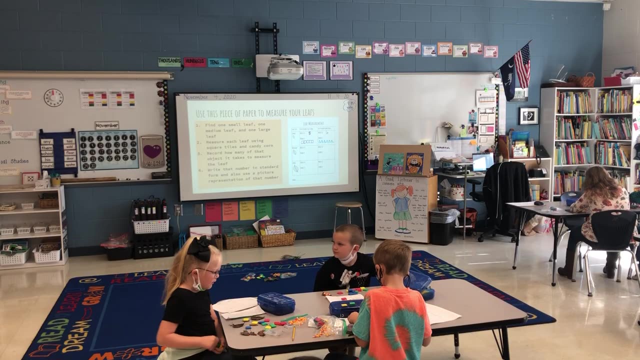 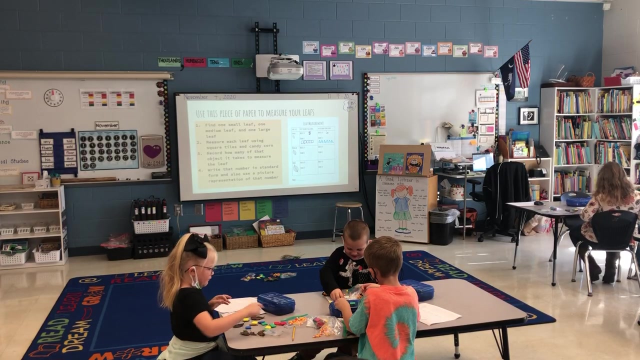 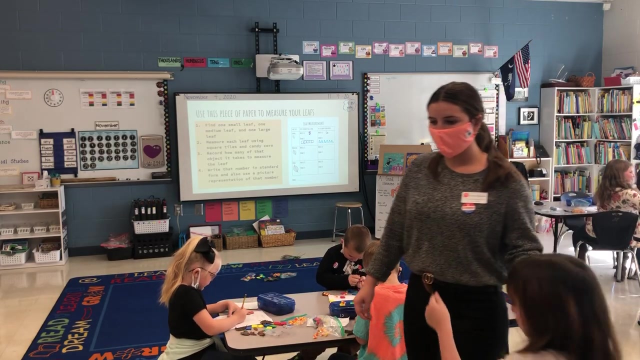 I don't have any medium Girl. I don't have any medium. Okay, so well, we're supposed to be working with Jackson, so can you say, Jackson, we're working together. Can I borrow some of your bags? 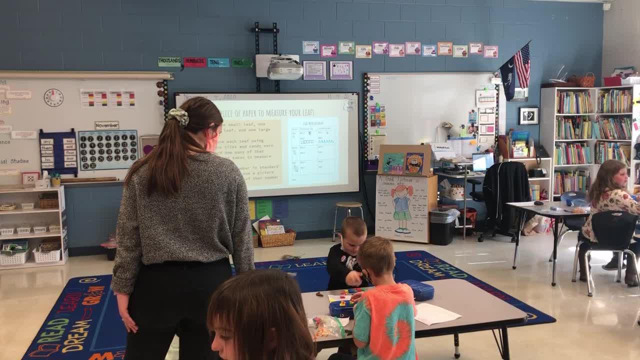 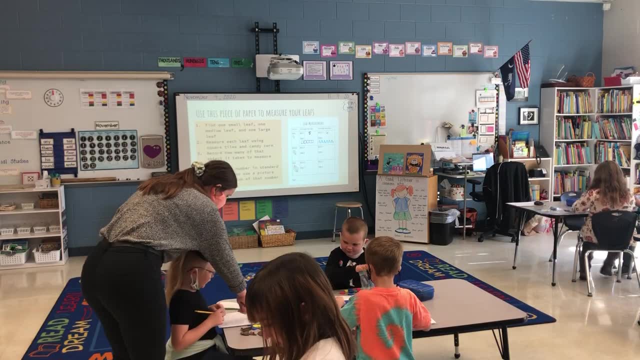 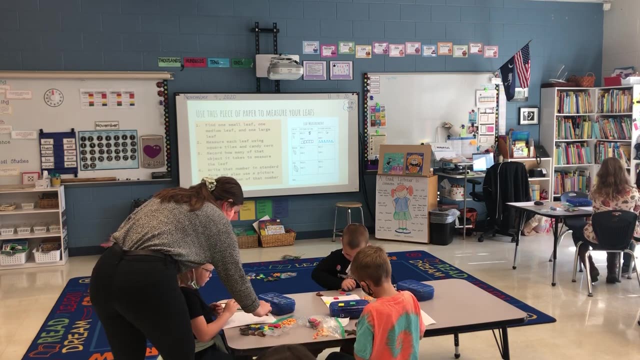 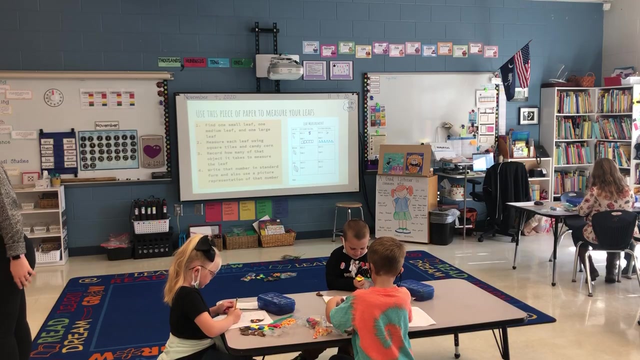 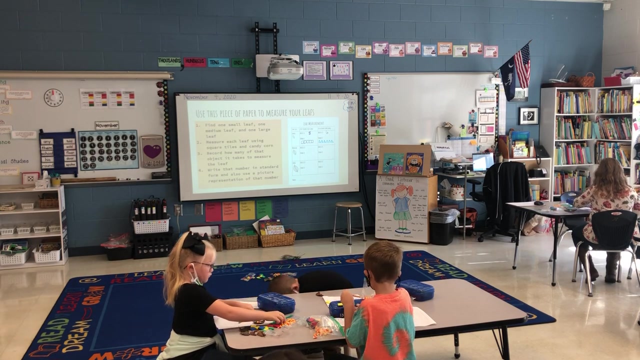 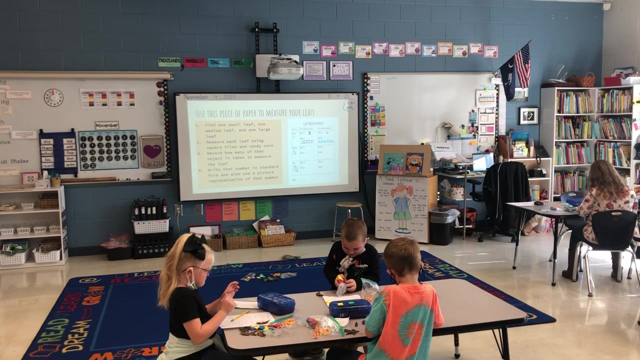 A medium. I want Jackson's bag. Okay, that'll be good, That'll work. It's not pretty, I know. I want Jackson's bag. One, Two, Look, Three, Three, Hey, Four, A four-square card. 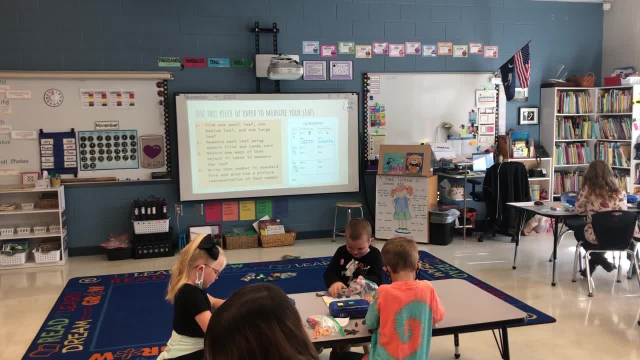 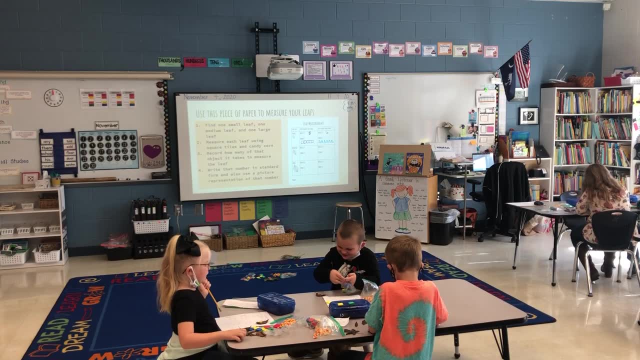 Okay, I'll also need a candy measure with your squares. Yeah, that's it. What do you use for your squares? Oh, We're gonna write down this. It's eight, One, Two, Three, Four, Five, Six. 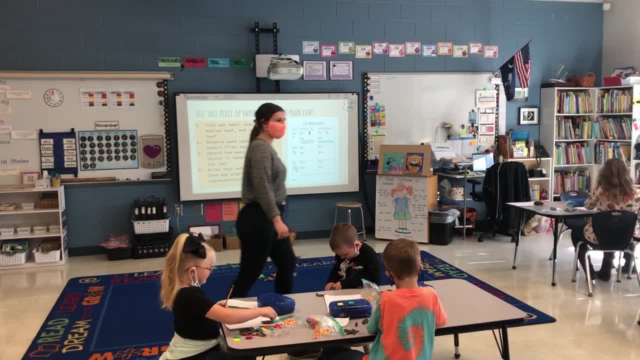 Seven Eight Nine: 10., 11., 12., 13., 14., 15., 16., 17., 18., 19., 20., 21., 22., 23., 24.. 25., 26., 27., 28., 29., 30., 29., 30., 31., 32., 33., 34., 34., 35., 36., 37., 38.. 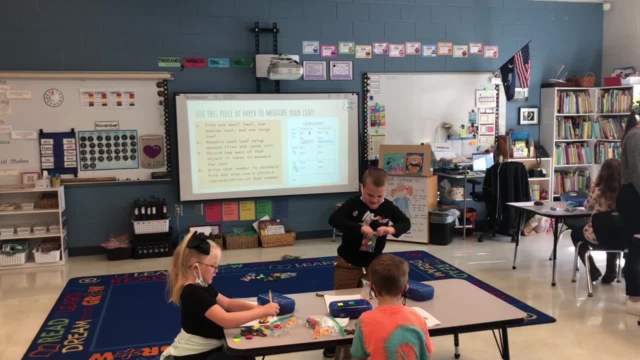 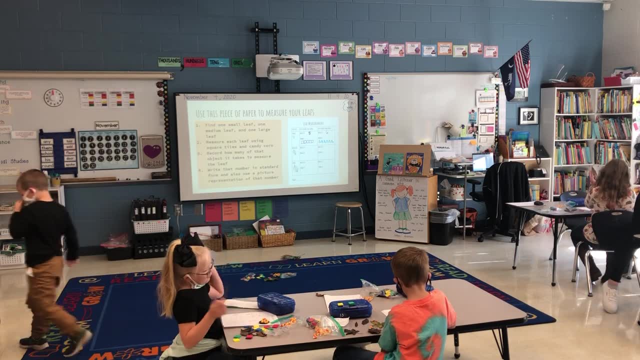 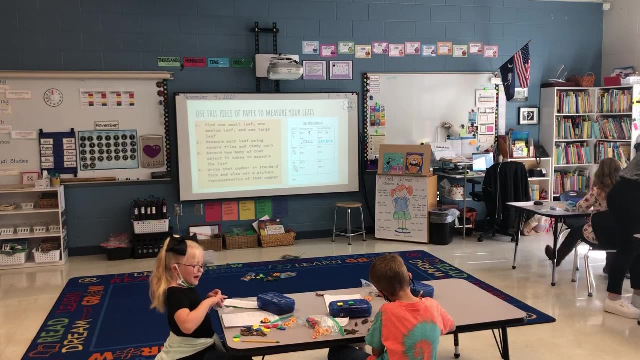 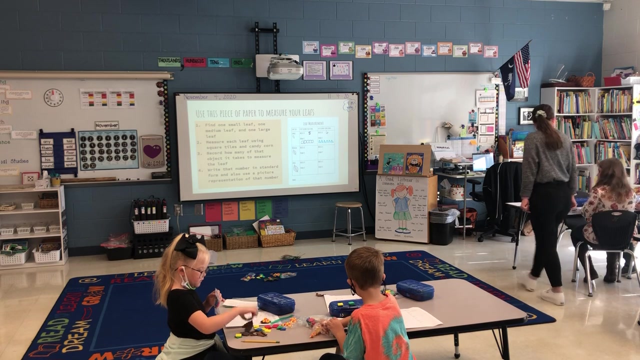 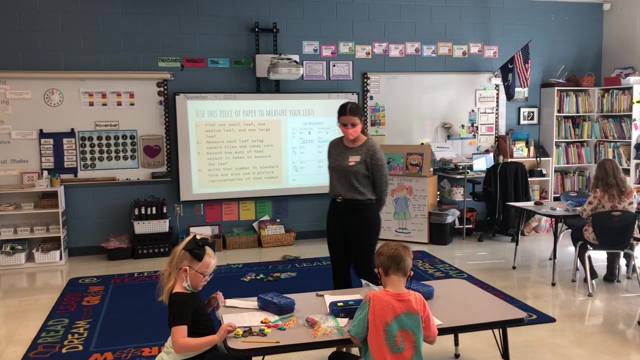 38.. 39.. 40.. 41.. 43., 2. 5. 51.. 2. 2. 3. Two, three, four, five, six, seven, eight, nine, 10,, 11,, 12,, 13,, 14,, 15,, 16,, 17,, 18,, 19,, 20,, 21,, 22,, 23,, 24,, 25,, 26,, 27,, 28,, 29,, 30. 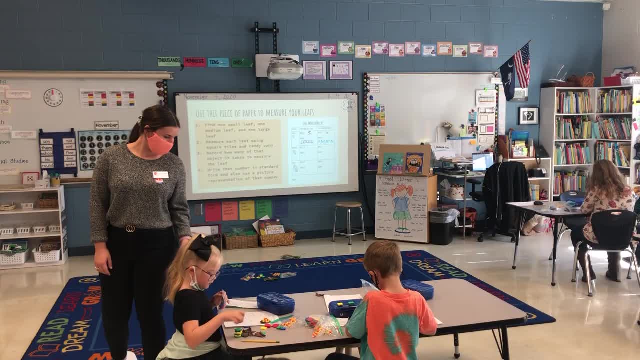 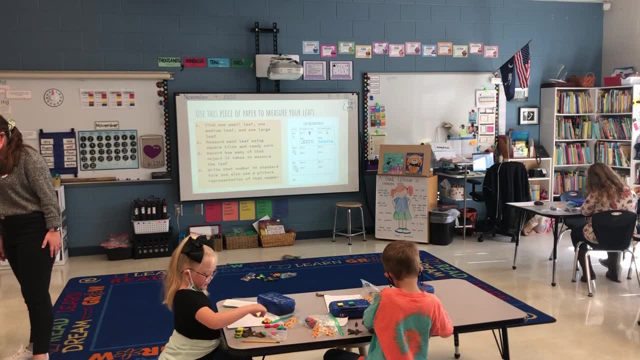 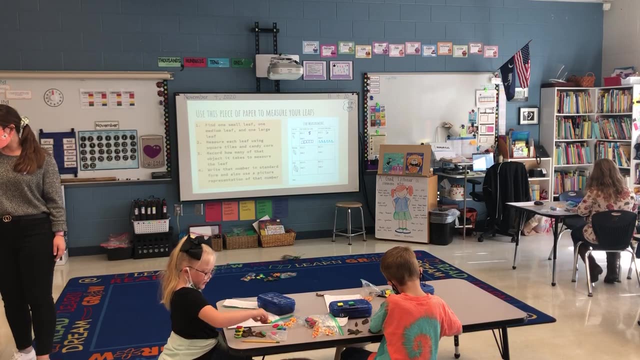 There's actually six pieces. Are you going to measure with your candy card? So show me How small This is the smallest. Is that a piece of sweet? Let's see how many it is. Whenever you're done, you can get a smaller one. 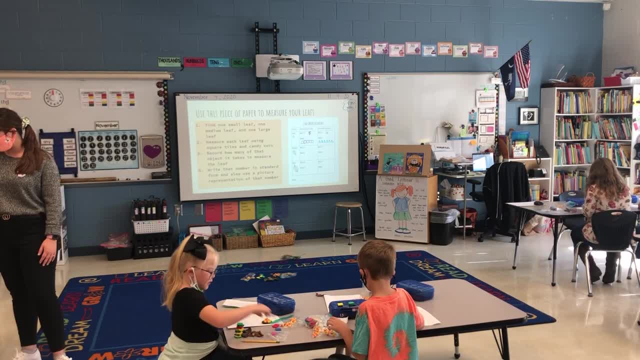 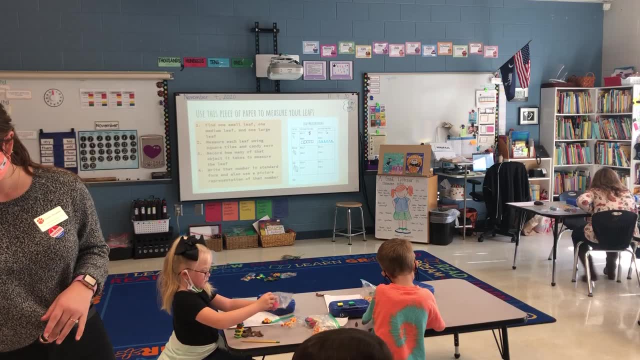 I didn't even try to grab a pattern. Okay, you are a leaf bat. Here's your leaf bat. I need a large one. Okay, you need a large one. Okay, What did you use for your large leaf? Oh, this one. 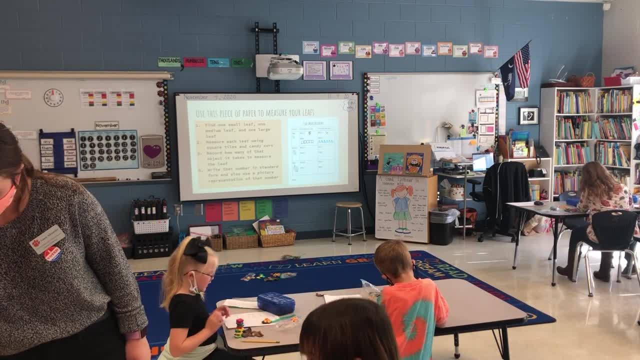 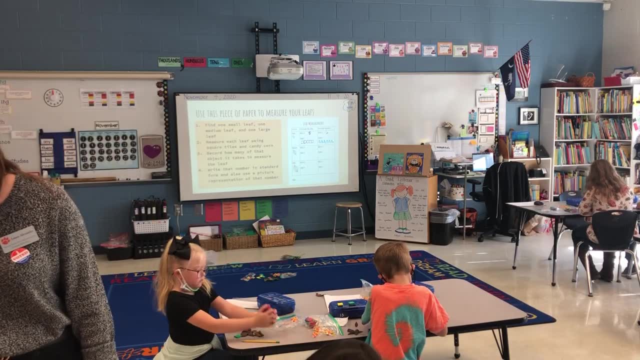 Okay, Measure it with the candy corn. Okay here. So, Carly Sue, you're going to measure it with that one, because Jackson said you could, And so then you need to measure those same leaves again with candy corn. Okay, I need that one. 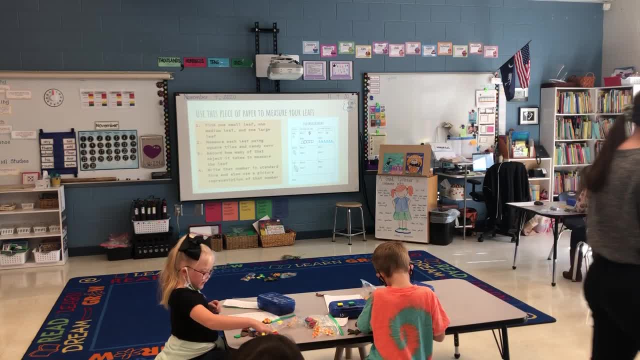 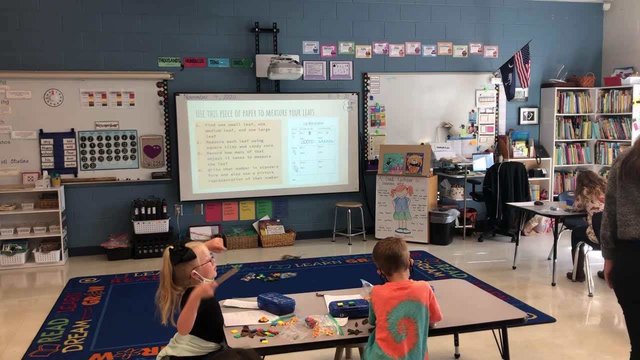 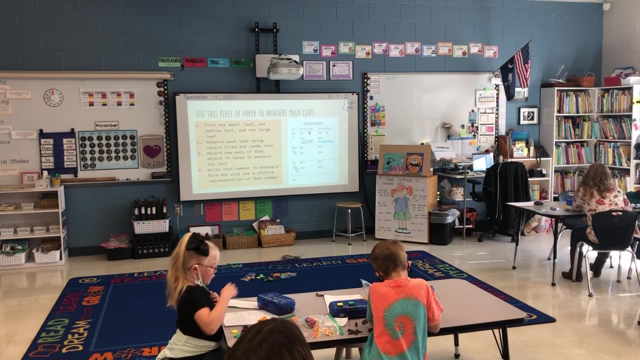 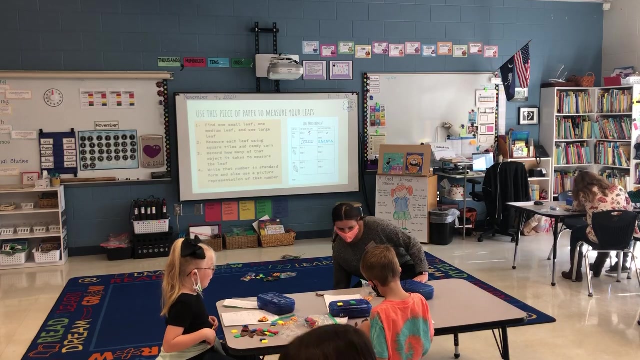 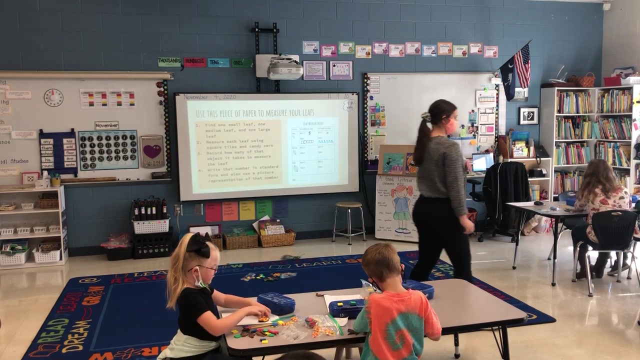 Carly, Please Sue Larry Tadda. Oh done Three. Thank you Four. I need red Four. Five, It's about five long. Okay, It's five, Yum yum, yum Four. 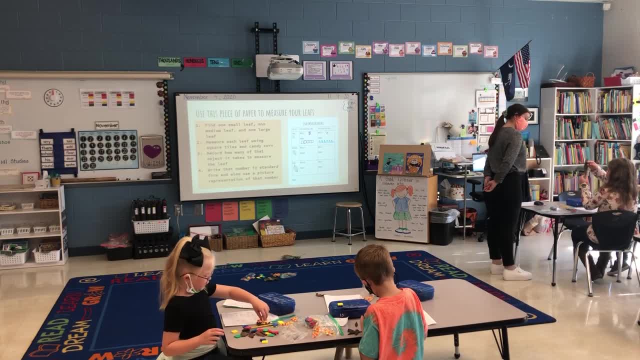 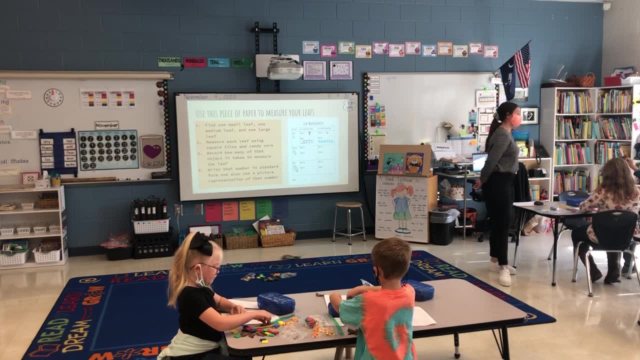 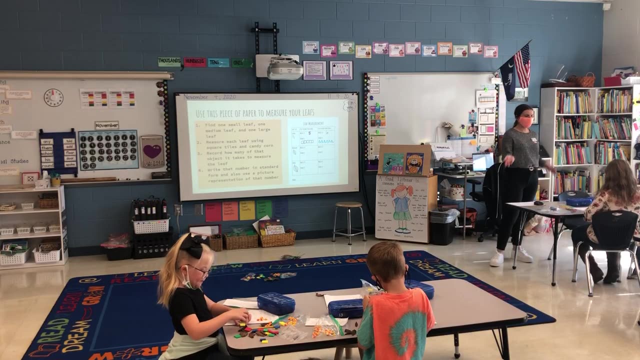 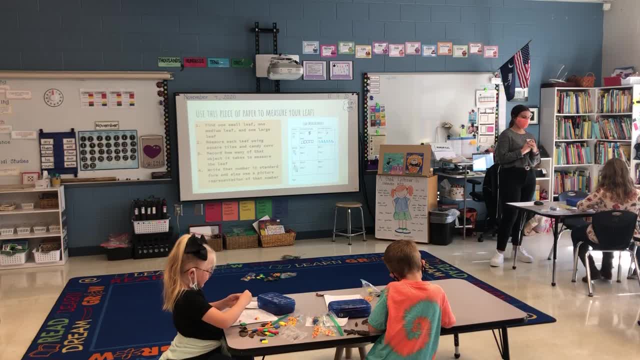 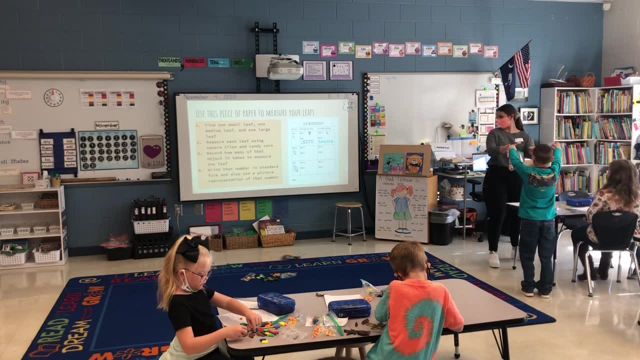 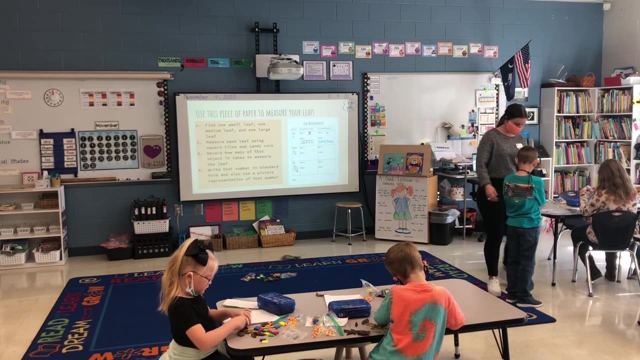 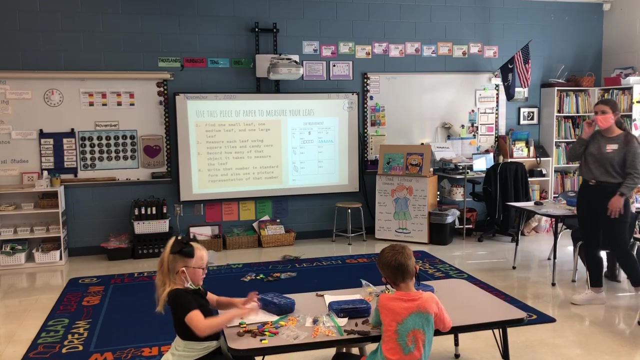 How many little leaves do little leaves have? We're curious about? about five little leaves. Now I've got a lot of candy corn. Well, I like all those. I like the holes in there. That's pretty cool. One, two, three, four. 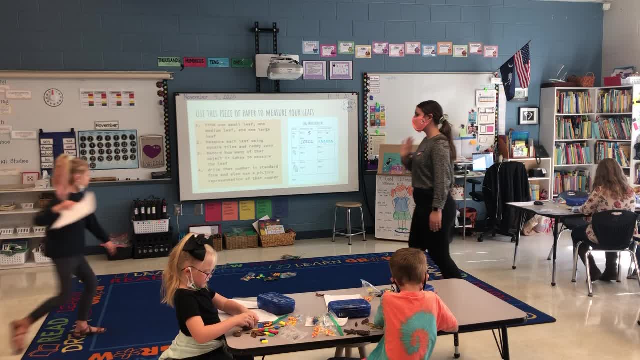 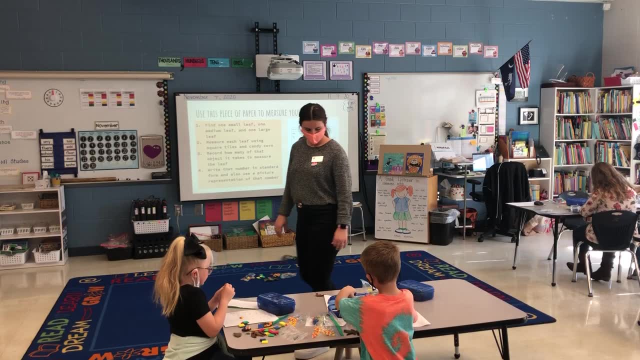 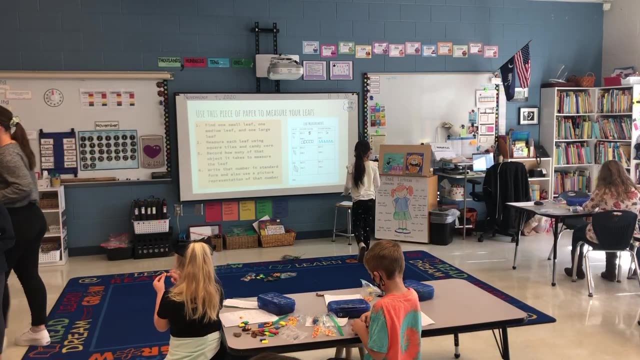 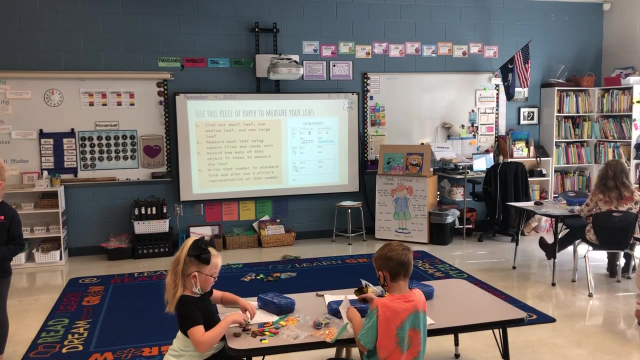 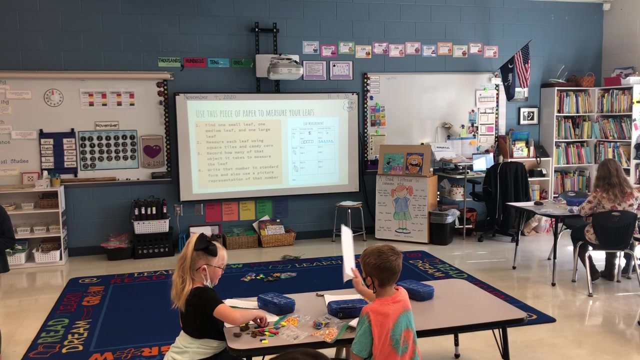 I'm going to make it past five, Four, Two, little, That's what you're doing. Five, six, six. another one can't fit on it. seven, it's seven long. it's seven long with candy corn, and now I want to eat it. four, four is longer than three, so it's seven long, candy corn, and, yeah, I eat candy corn. seven, 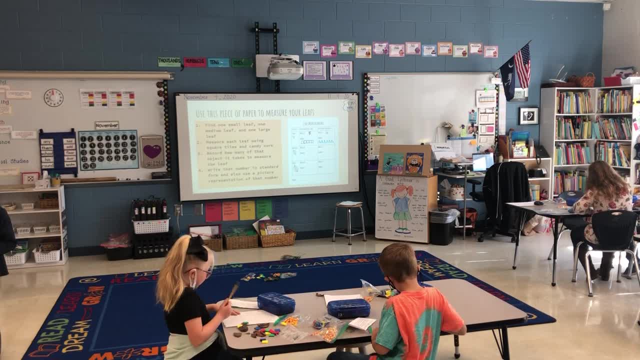 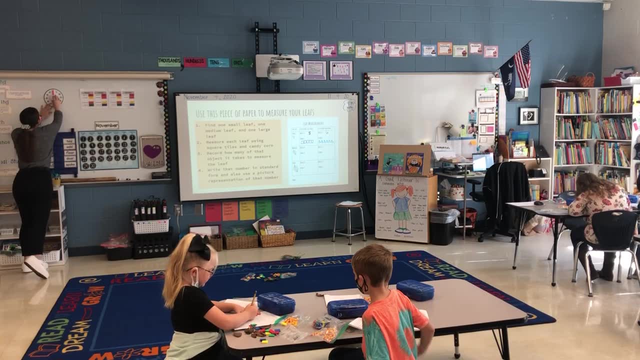 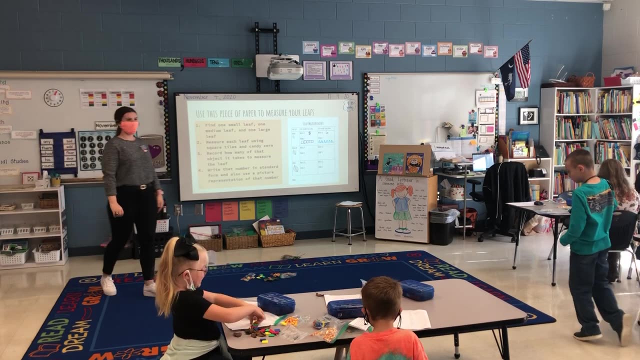 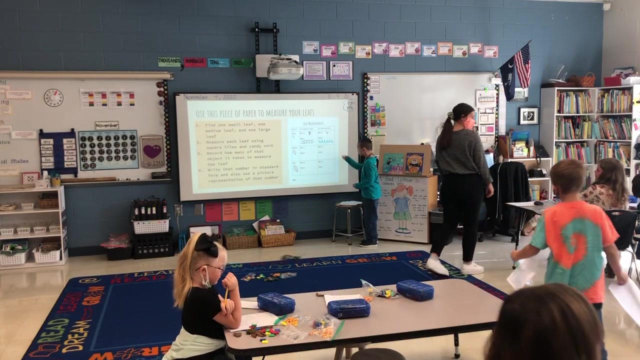 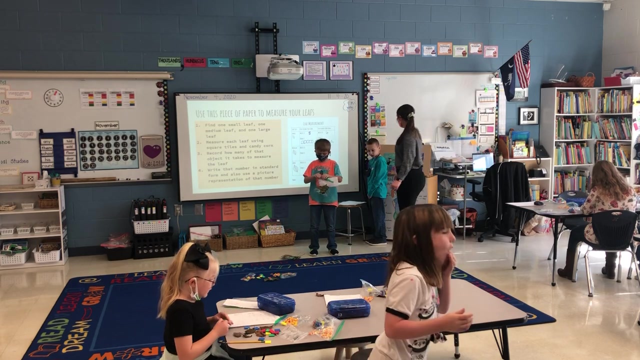 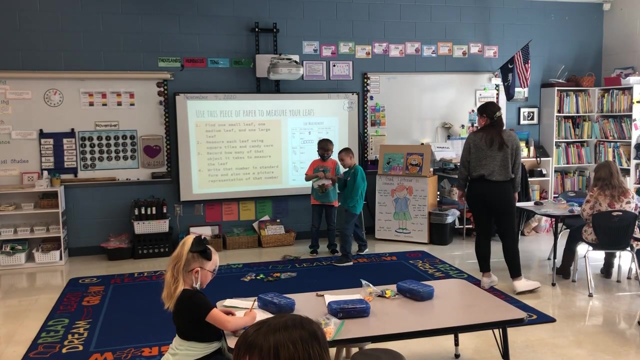 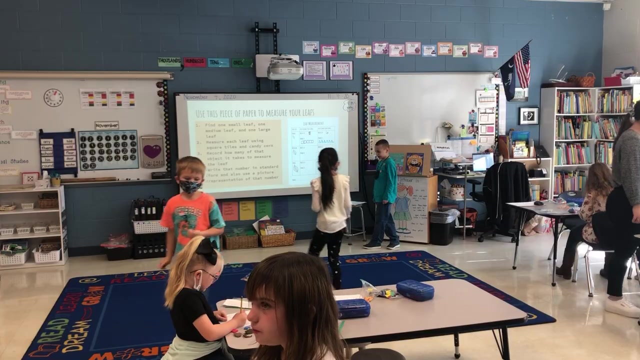 Seven long candy corn. Five, six, seven, six. Yeah, I'm gonna eat this one. Did you finish that? I still have one more? Okay, go for it. It's three blocks. The largest leaf that I did was a seven candy corn one. 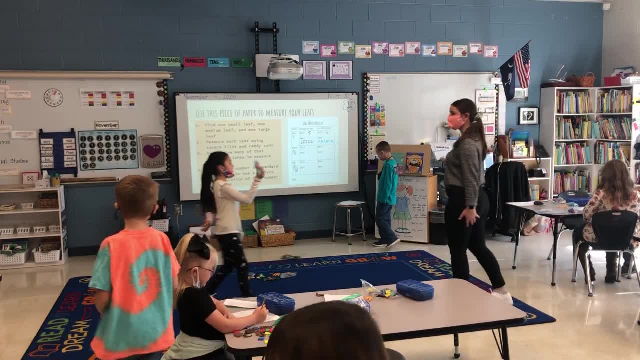 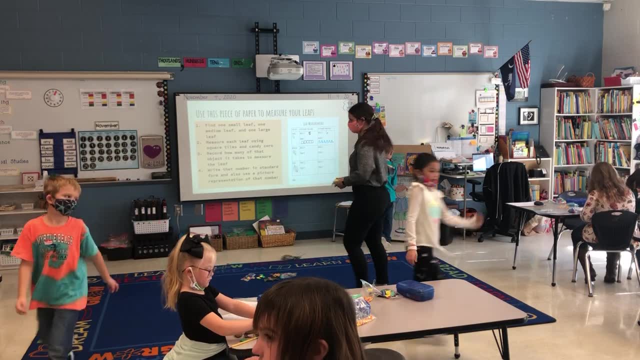 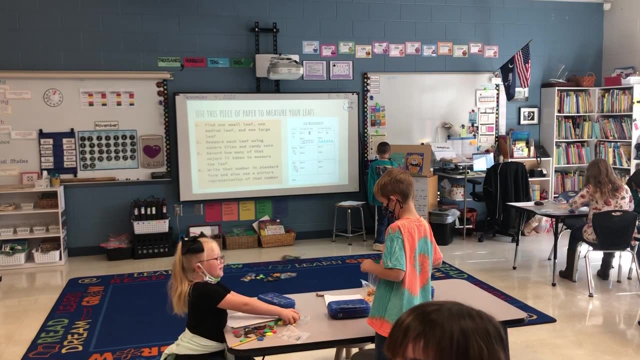 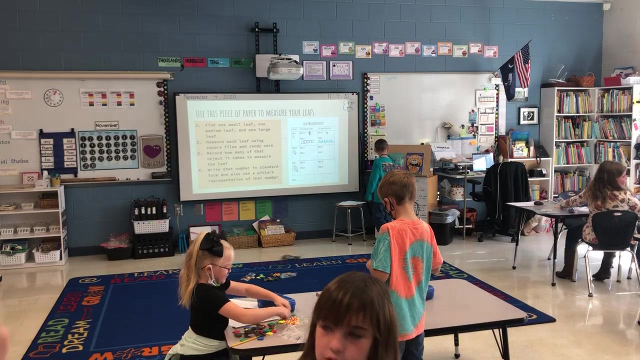 Oh, the largest one. What was the smallest leaf? The smallest leaf was two squares and three candy corn. Why do you think it was different? Because the candy corn was smaller than the squares? No, the candy corn was bigger. The candy corn took more. Why do you think the candy corn took more than the squares? 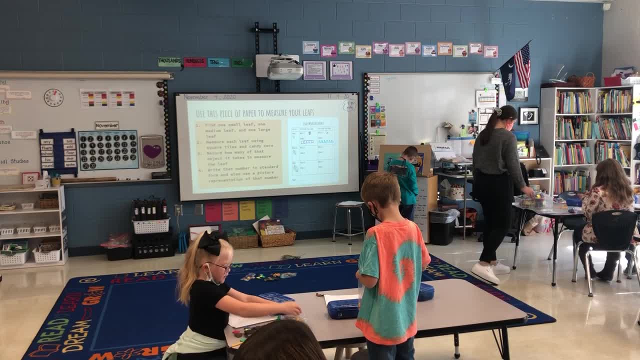 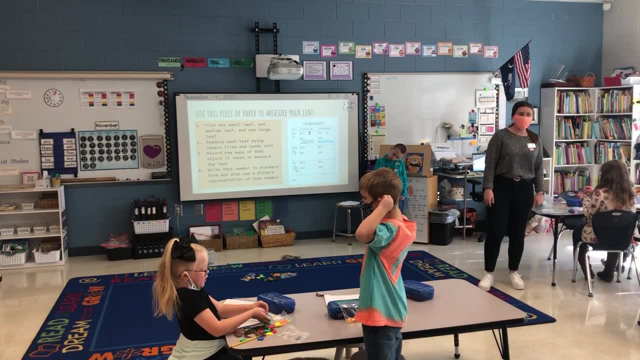 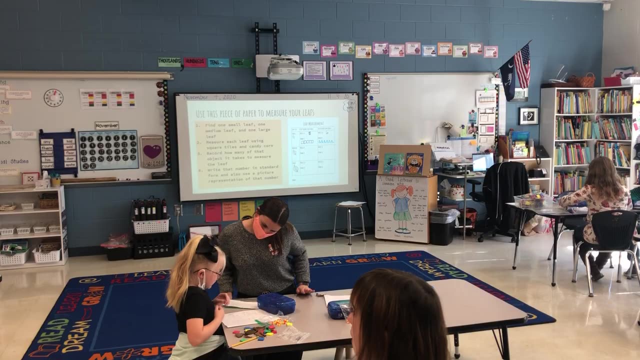 Because the candy corn is smaller. Ah, the candy corn is smaller. Oh, that's a really small leaf. I know Betsy, don't forget to come up. Five, six, seven, Okay, so it's just a little stuff. 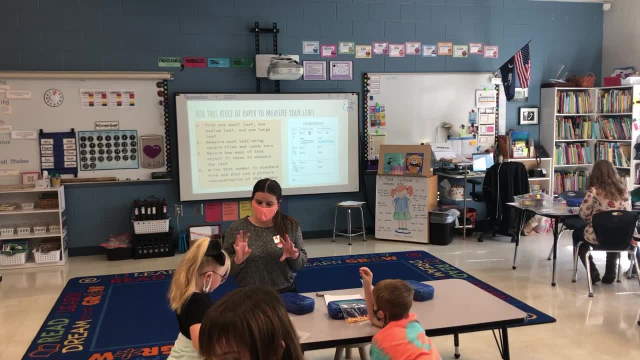 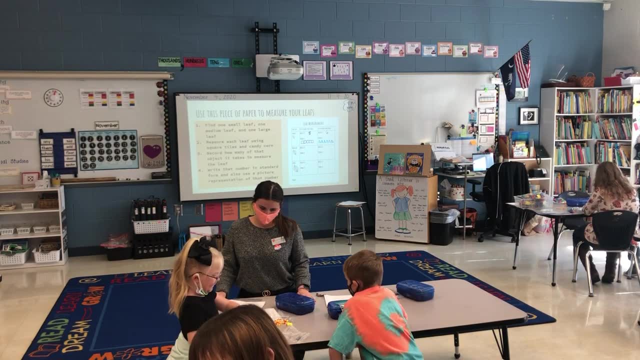 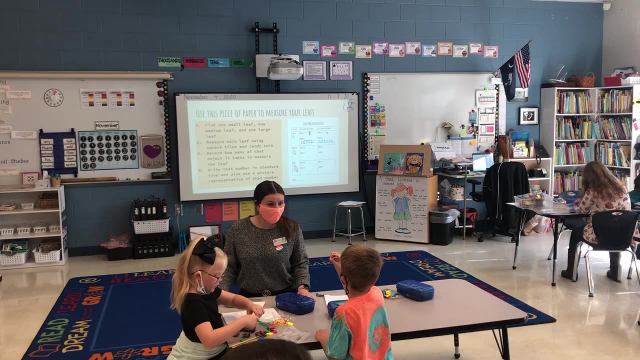 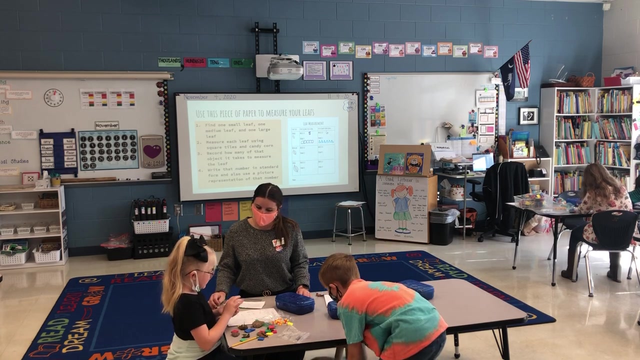 So how did you see the candy corn in the square house? I saw this one with a. This one: Five six seven. Five six seven, Are you done? Yes, Then we can. So how did you compare with each other? 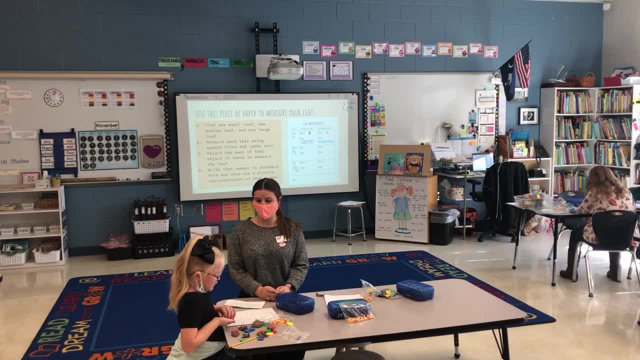 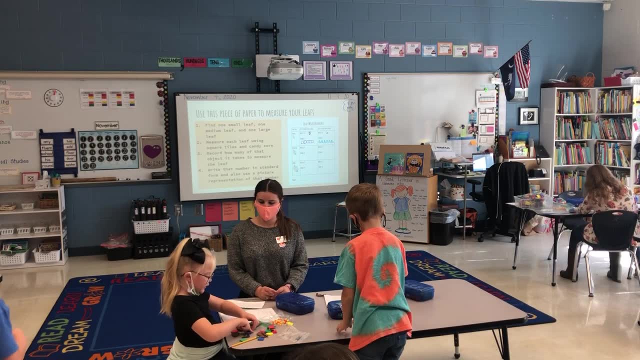 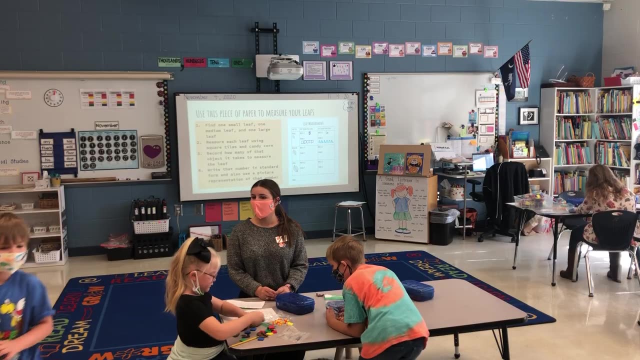 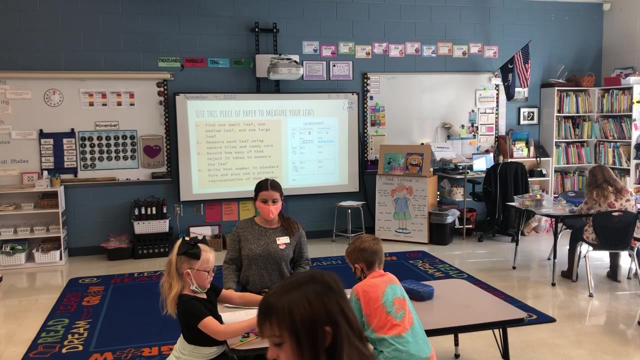 How did the length of the leaf change? I can tell by the number of pieces. Okay, so it's just cut different. Five six seven, Five six seven, eight. That means I have a total of six. outside my block of Maybelline to see my candy corn. 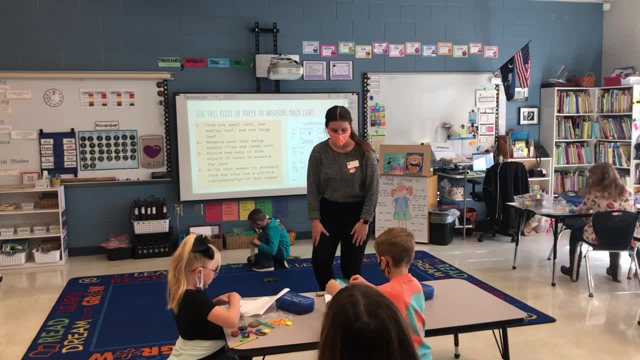 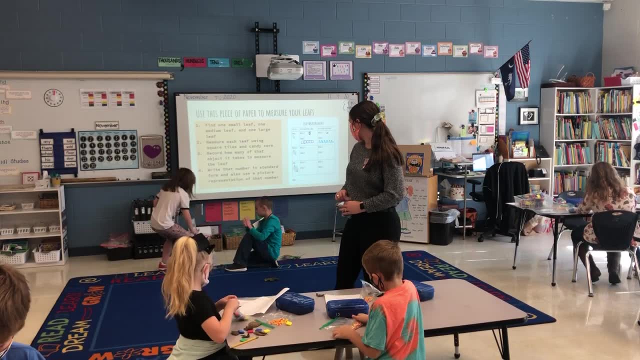 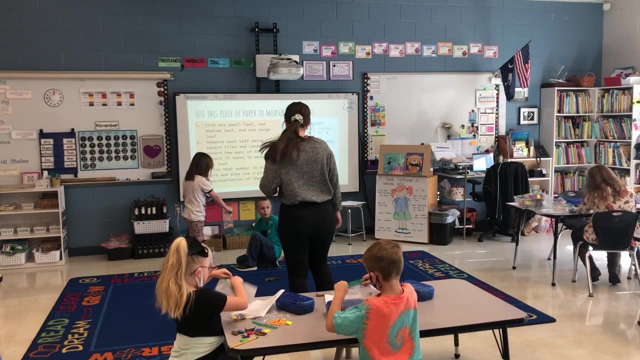 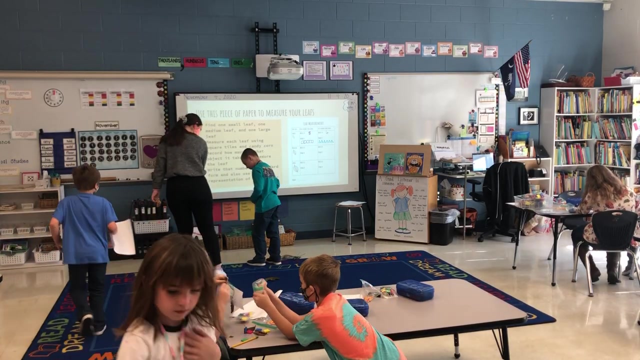 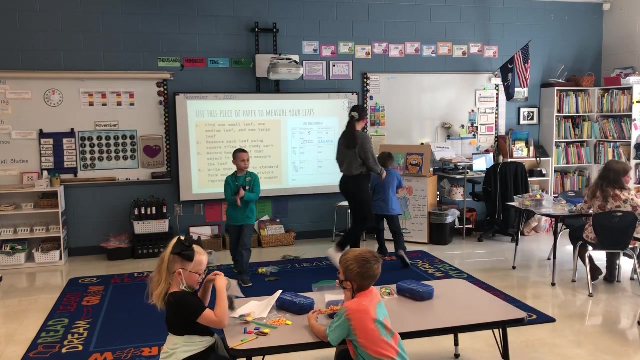 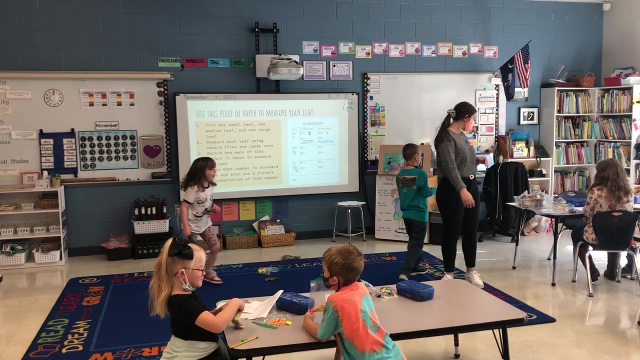 We've just got a few minutes left. Ladybug, I'm going to my room. Okay, can you put them back in the week? Okay, I don't know, I don't know. No, that's Isaac, I mean. no, that's Noah. 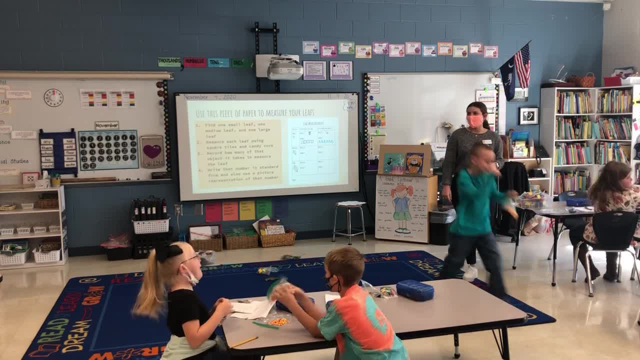 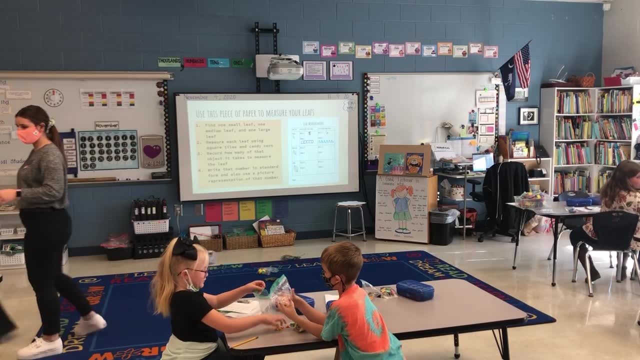 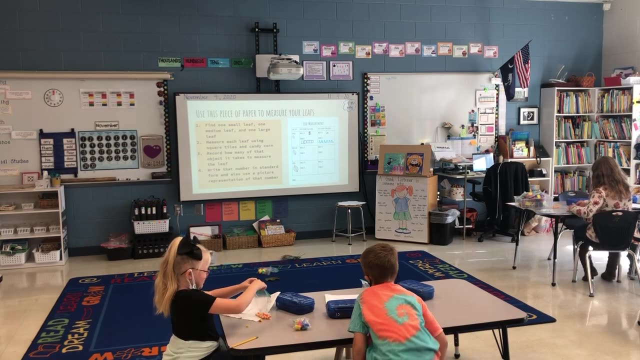 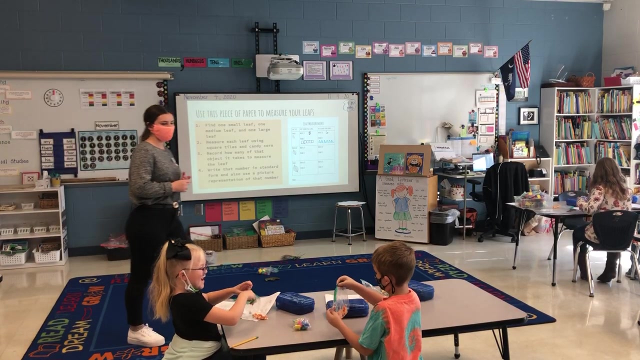 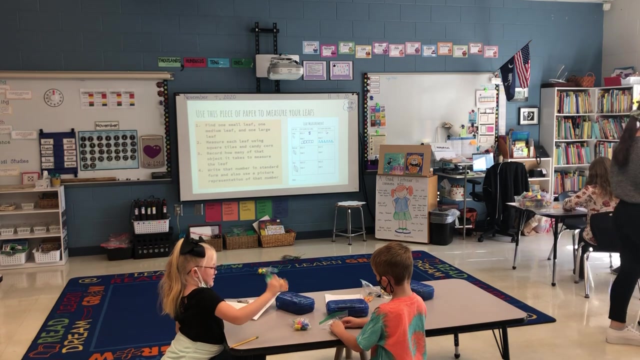 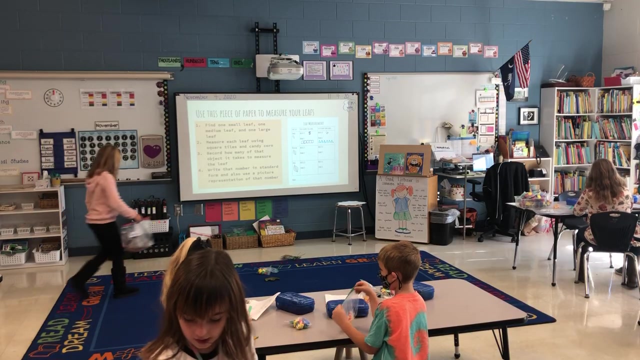 Sorry, that is Andrew. Okay, my candy car. Here is it. Are you all done? Can we clean up before? Yes, I'm going to clean this up. Oh, yeah, Yeah, Candy car, Do you just want to cross on the other side? 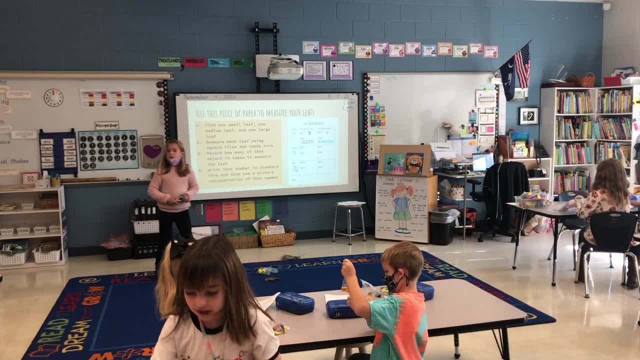 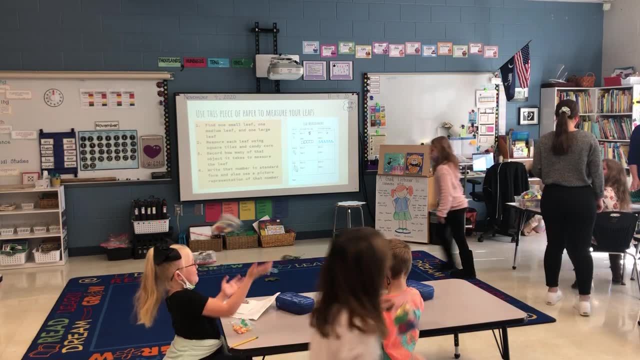 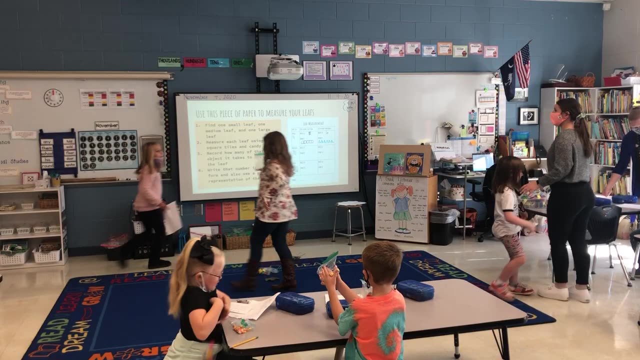 The only time I've ever put it in the biggest, it's with the stubby candy car. Now I know. Okay, Toilet paper. Yes, Oh yeah, Oh, yeah, Okay, Can you meet me back at the circle please? 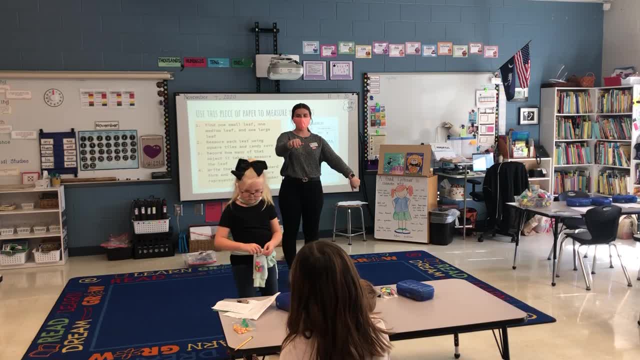 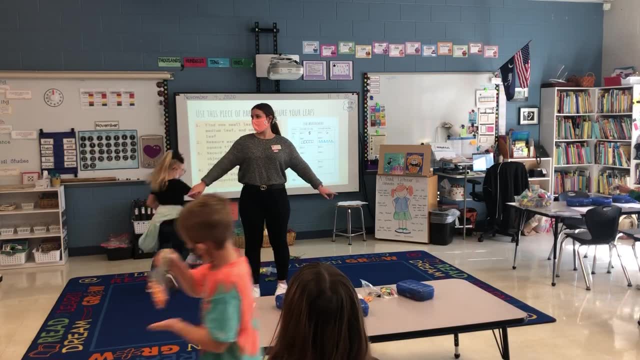 Oh, I found a인y, who I want. What if I made a? Come on, come on, Can you come over baby? Come on, I want to see your car, But the car won't let me go. Okay, okay. 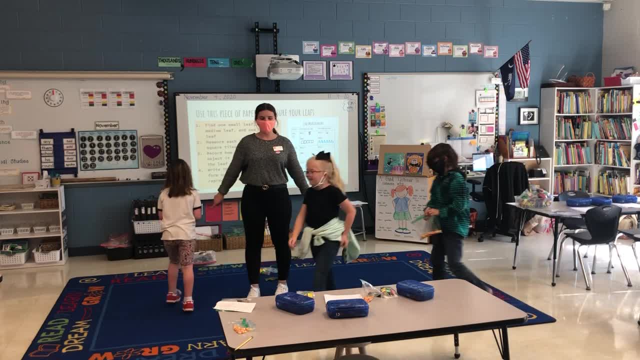 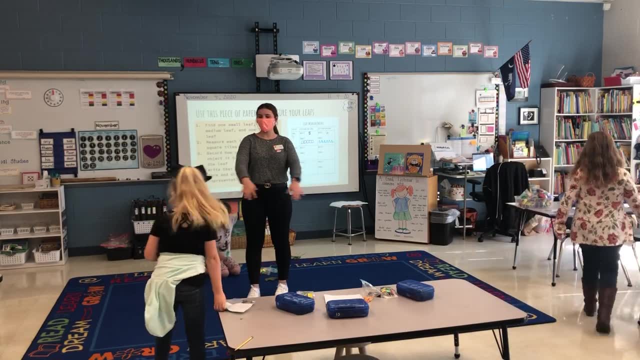 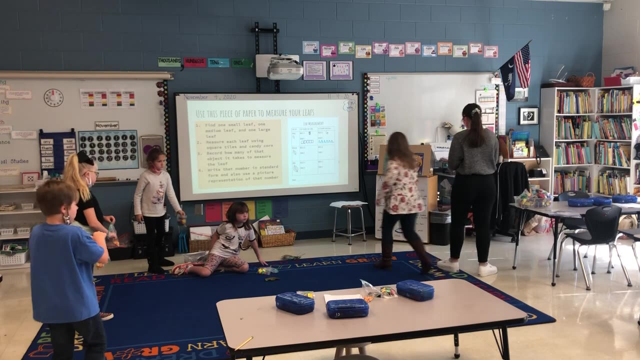 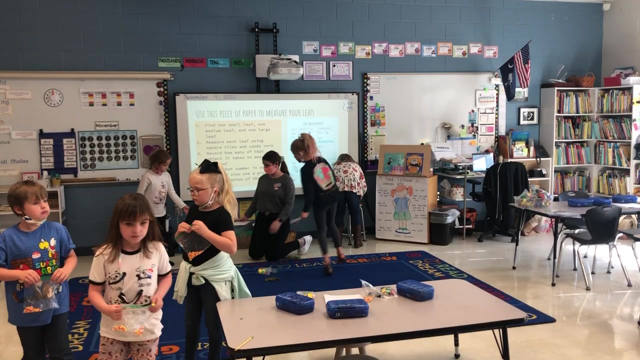 Come over. Okay, bye, Can you meet me back at the circle, At the carpet and corner Circle. If there's some more, can you bring them over to Mrs Thaler? No, I don't think there's some more in the room. 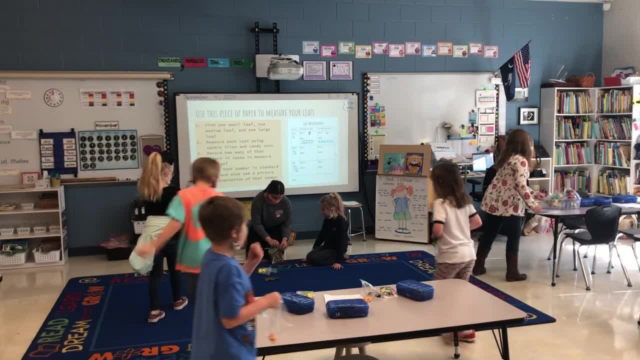 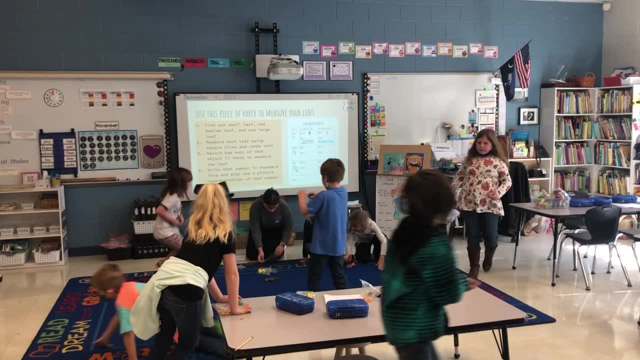 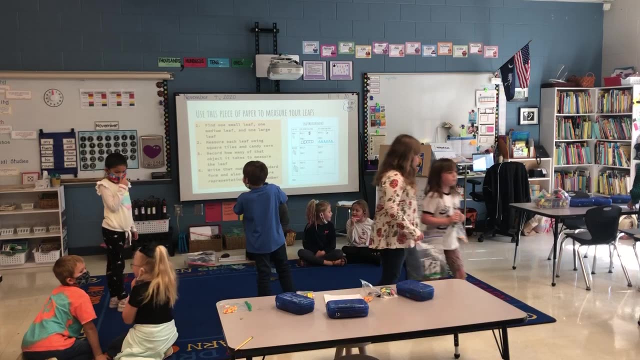 Do you have some more at the end of the course? I don't. Do you have any more in your bag? I don't have any more. Okay, can you bring them over? I've got to press them first. Five, No, ma'am. 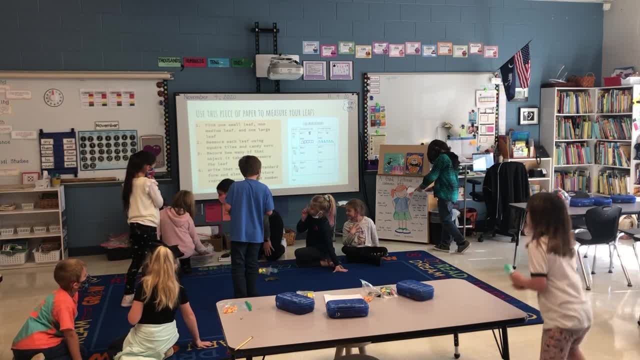 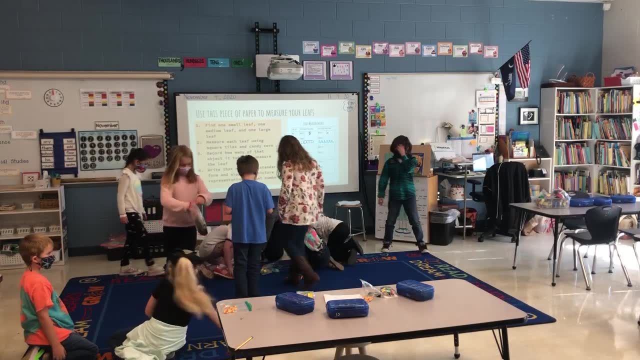 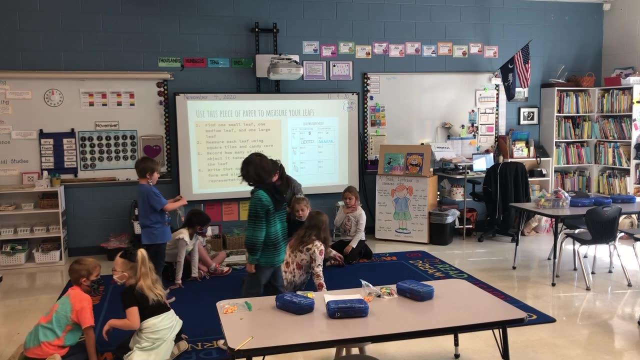 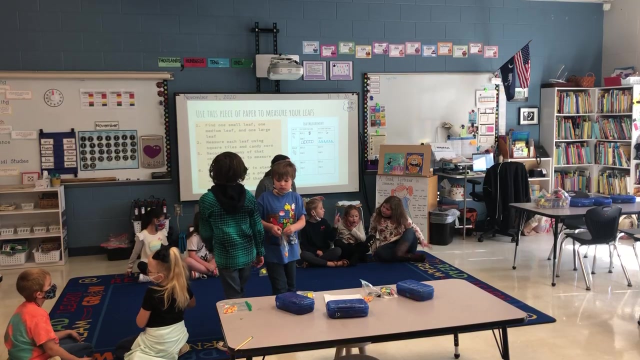 Just one more. Okay, Thank you, Reagan. Thank you Darlene. Ms Alex, do you want to do this one? This one? Yeah, Hold on, let me get a couple more. She said we can eat one piece. 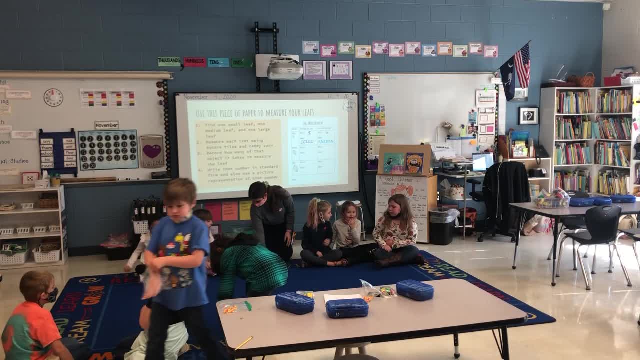 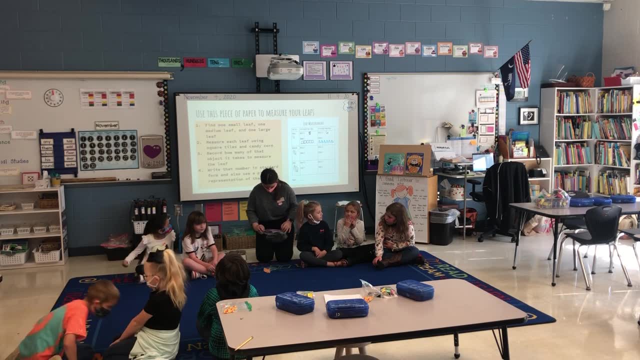 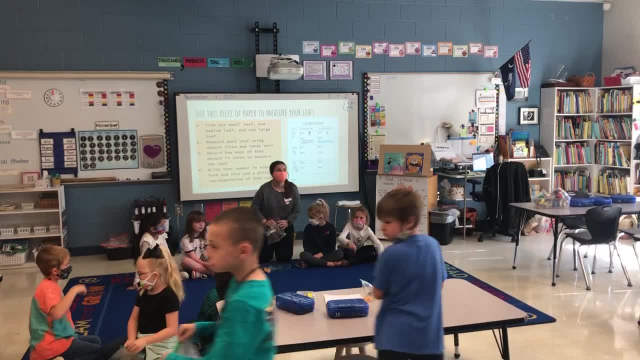 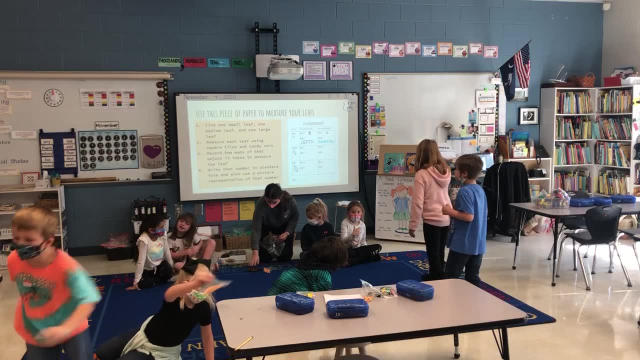 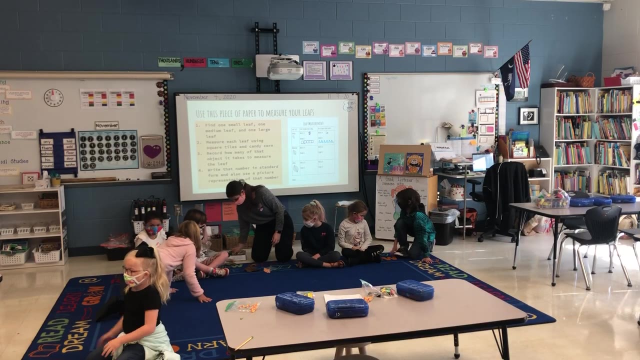 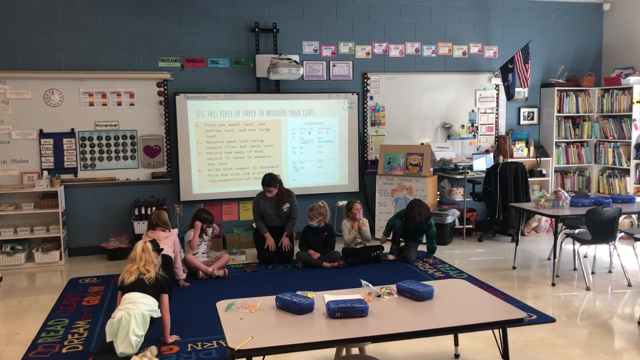 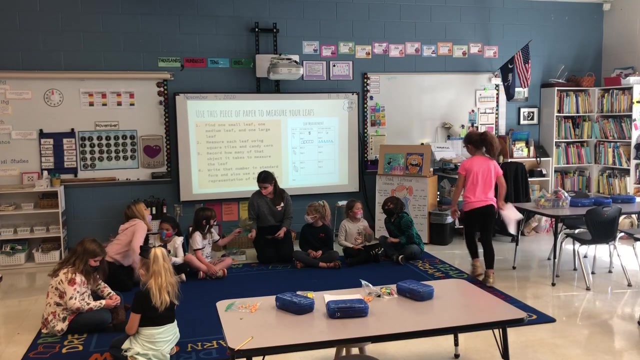 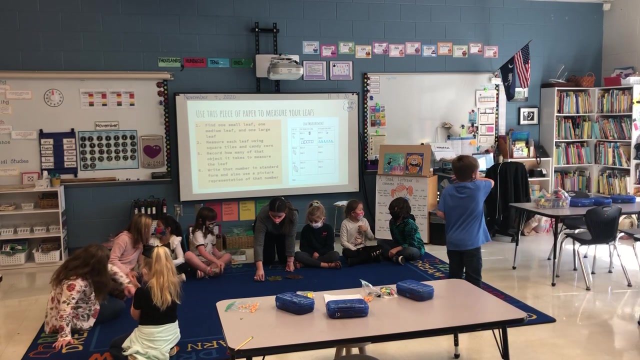 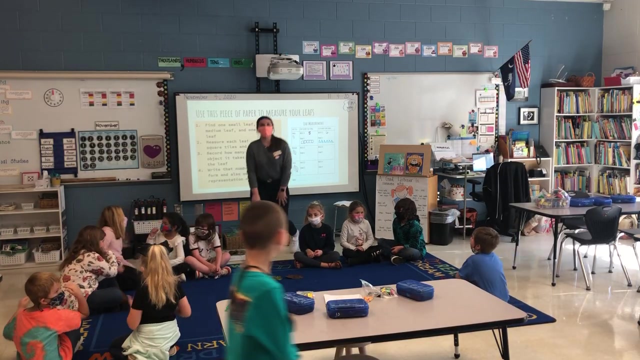 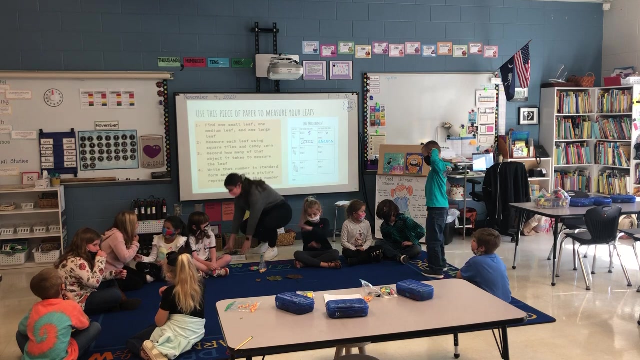 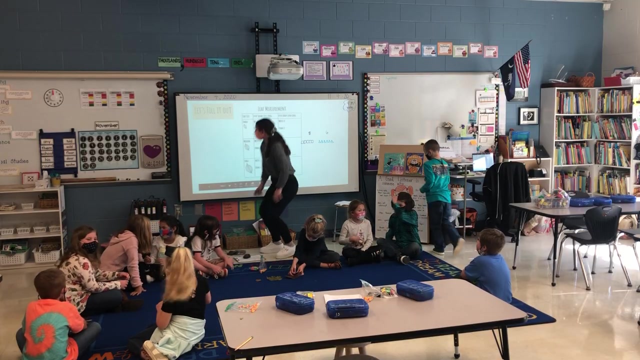 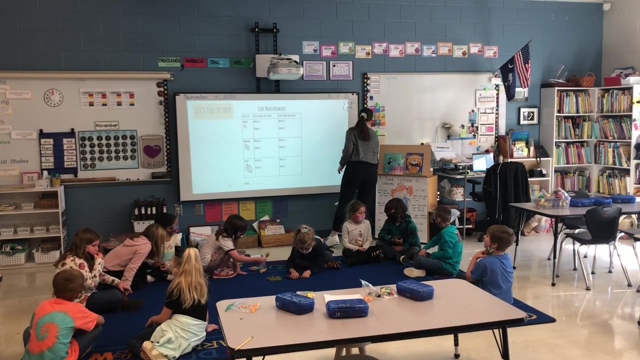 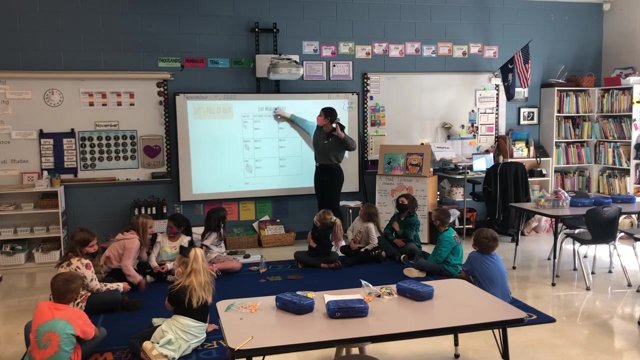 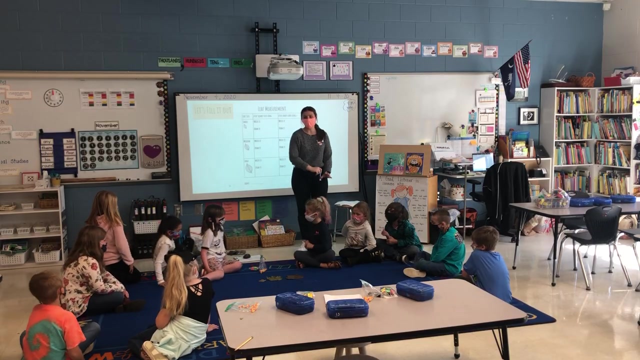 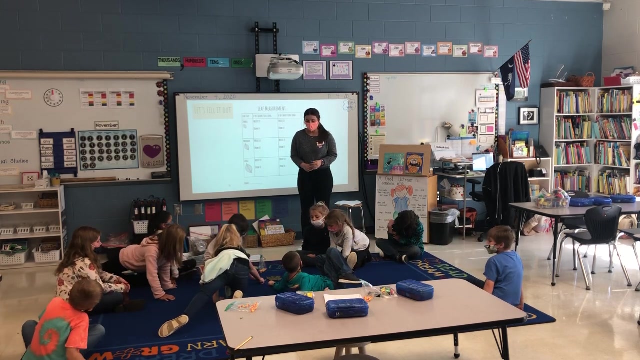 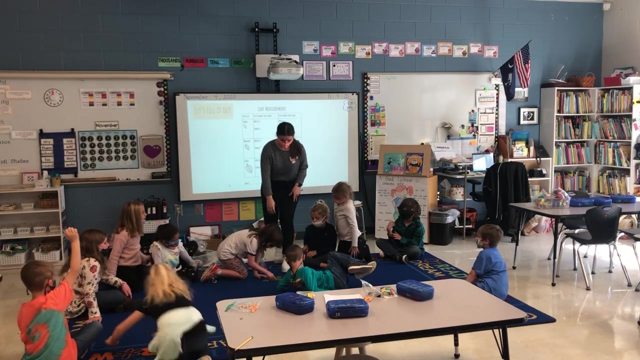 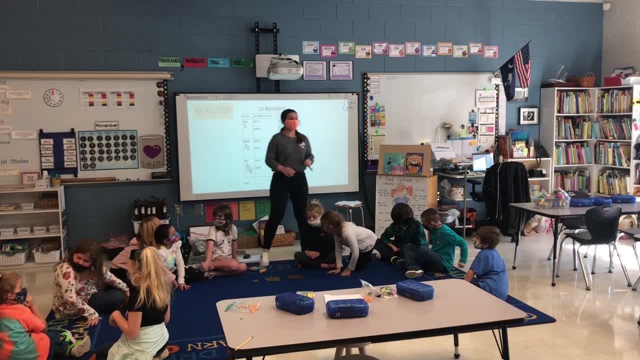 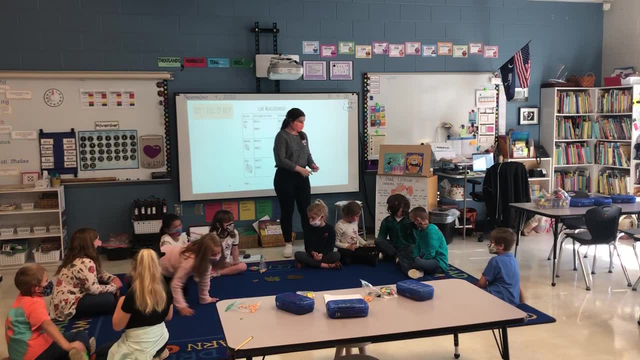 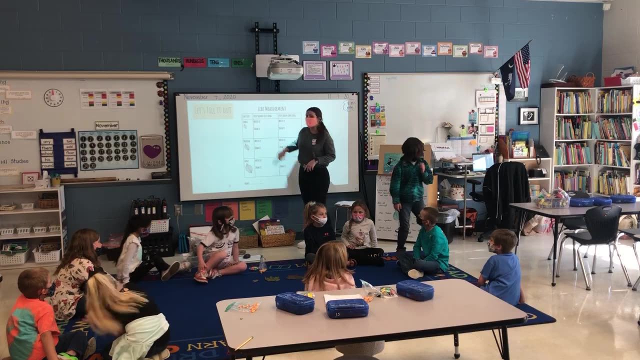 All right, so we're going to stay in our circle, okay, so that everyone can see: Wait, can you come over here And you can come move over there, so you can see that, Thank you, Okay. so which one do you guys want to start measuring? 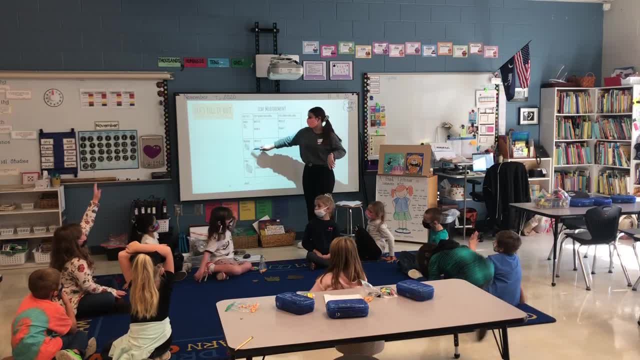 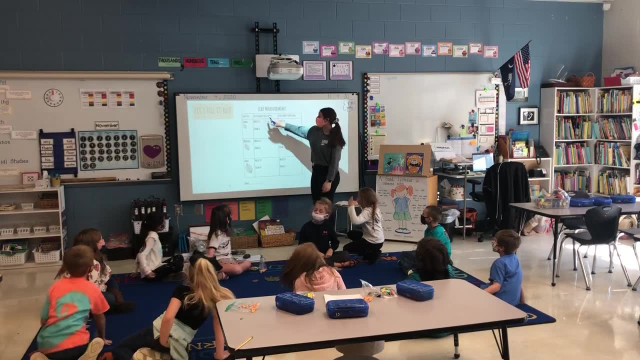 Small, medium or large? Who votes for the small? Who votes for the medium? Who votes for the large? We're going to measure the large first. Okay, so another vote. Do we want to measure with the square tiles or the candy corn? 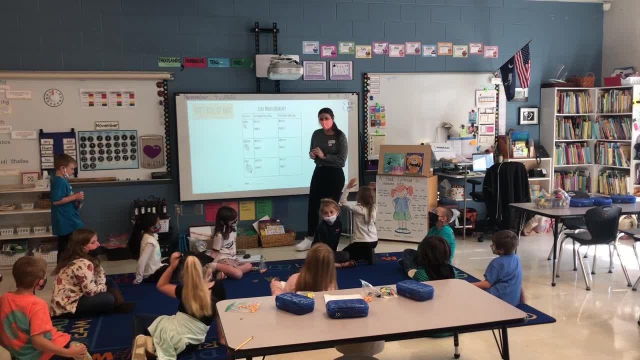 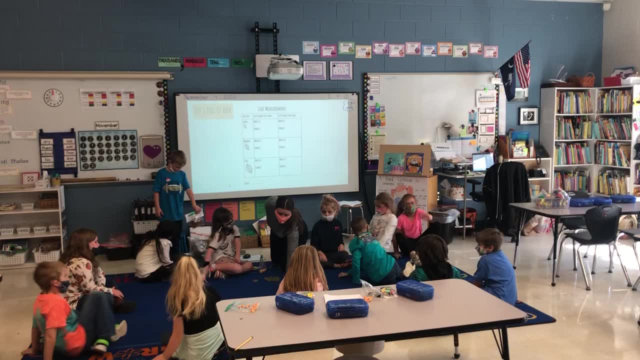 Candy corn. Candy corn first. okay, So which one was the large lady? This, This one. Okay, everyone, please stay in your seat, please. So I'm going to put this in the middle so everyone can see, and that way we can stay in our seats. 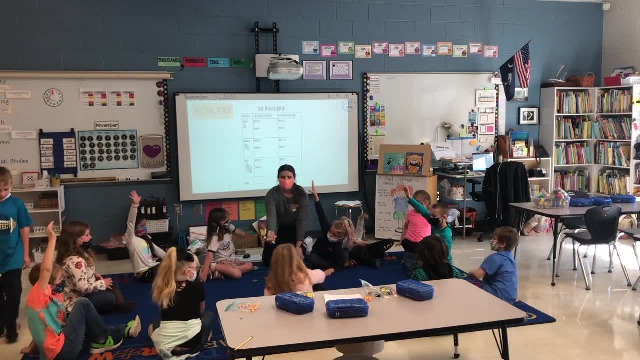 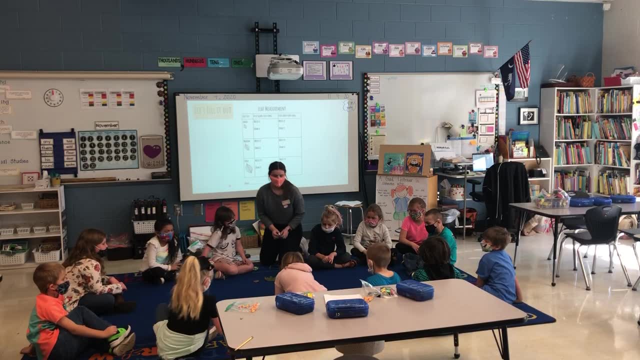 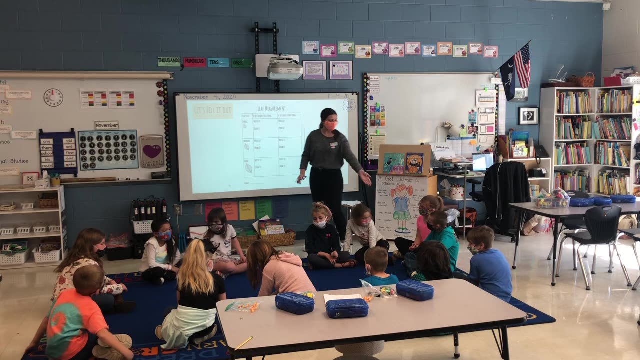 So I need one volunteer. Wakely, can you measure? show us how you measure with the candy corn you made. Okay, we're going to stay seated so that we can all see. Can you stand to that way a little bit? Thank you. 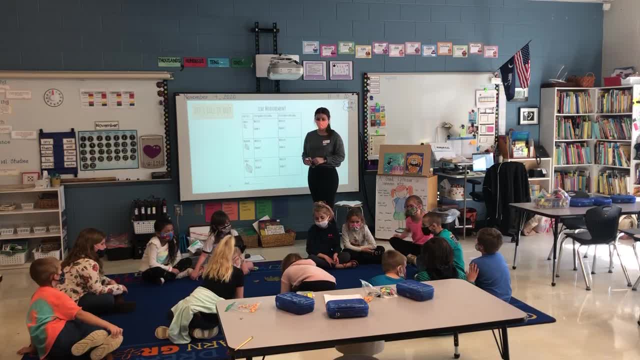 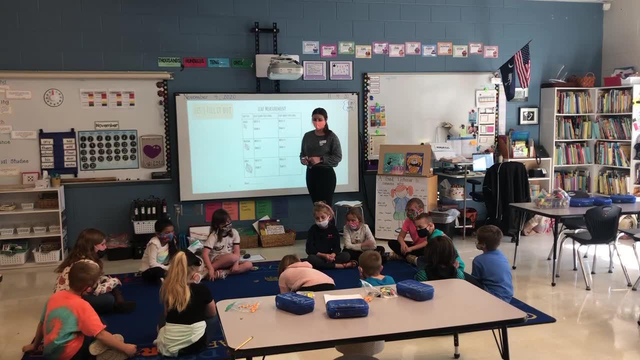 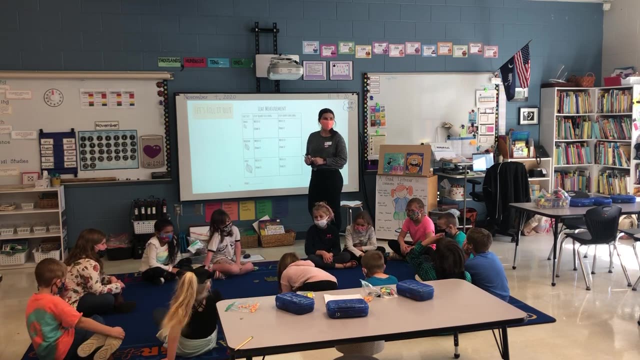 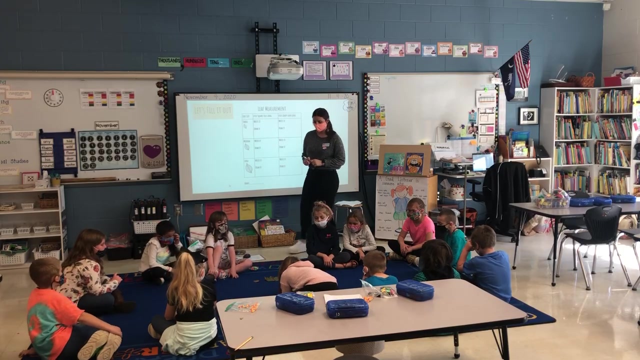 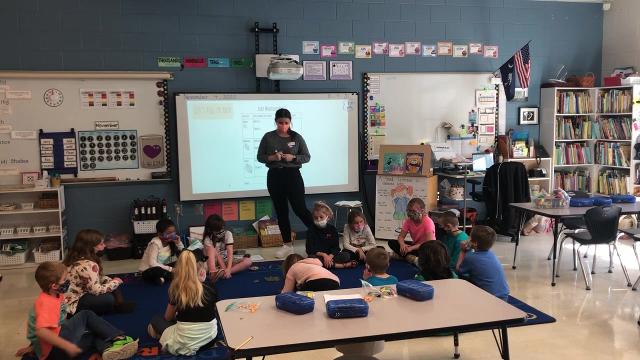 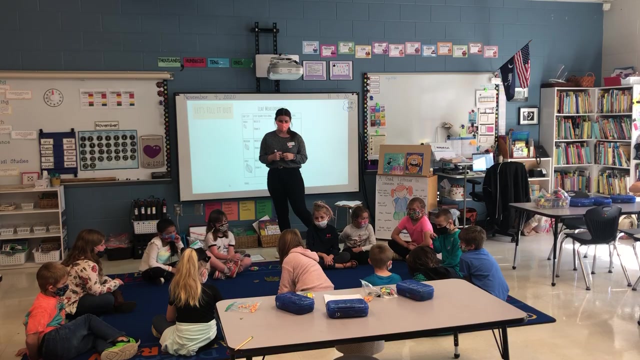 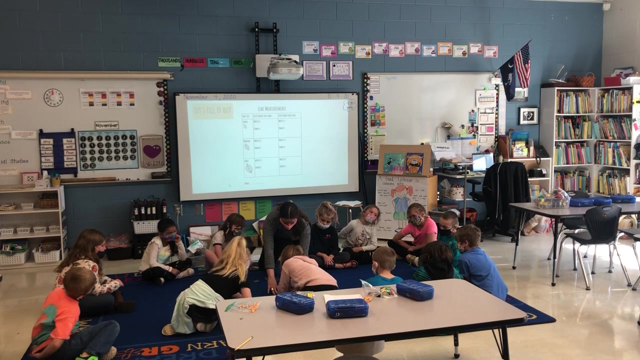 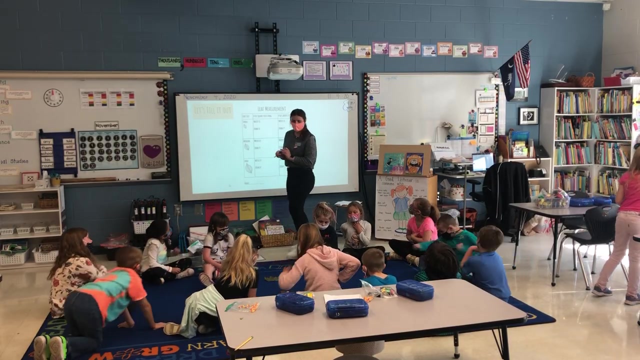 Thank you. Do we need some help, hon? Thank you, Thank you, So, Wakely, how many did you use? Six, It took six pieces of candy corn. and which leaf was that? What size? A large? Which size? 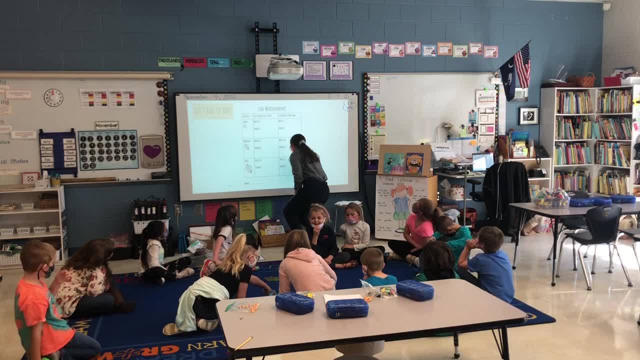 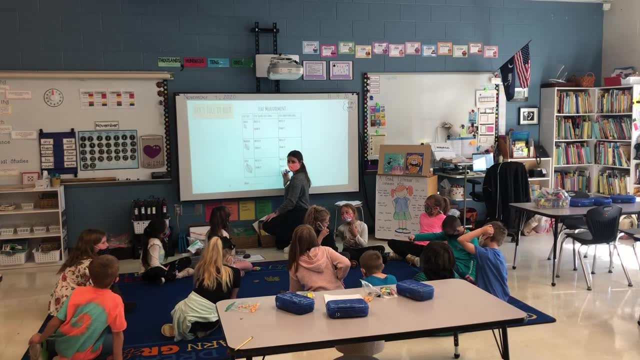 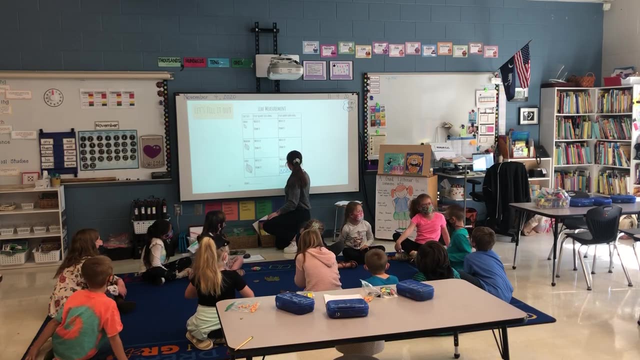 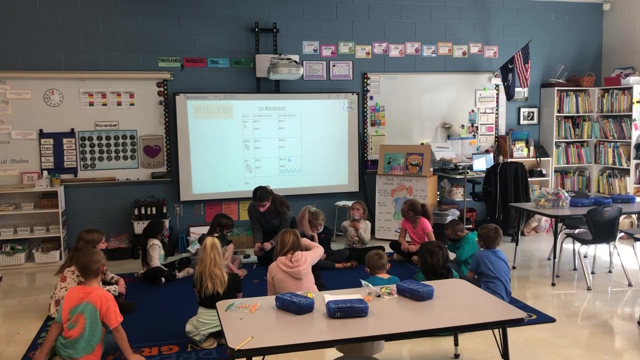 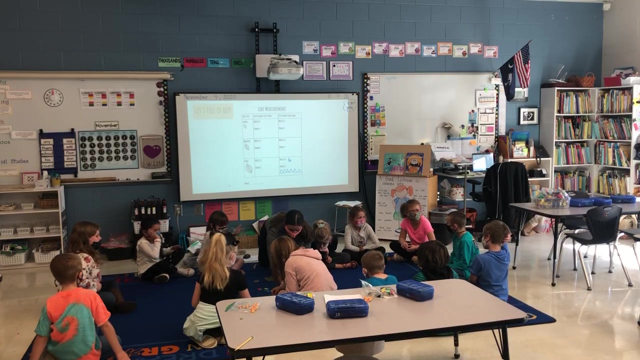 The larrybite, This one, So six. and then what should I draw? You should draw six circles, Or you could draw a triangle. A triangle, Please stop, Okay, and then I'll use the square tiles. now, Please stop. 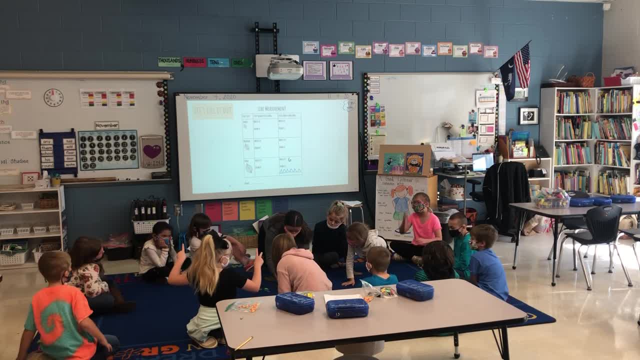 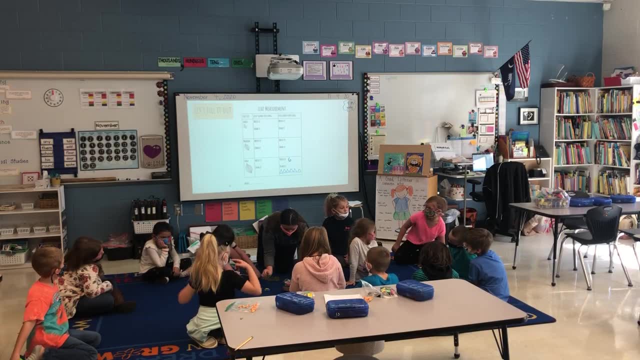 Can everyone count with me? One, two, three, four, five, six, seven, eight, nine, ten? Wait, how many are on here now? Four, Ten, Five, Okay, so what should I write? Five, 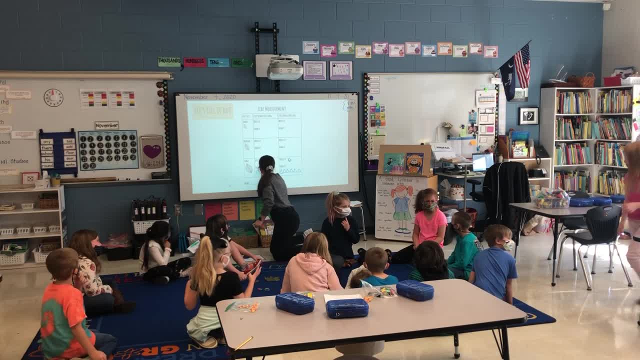 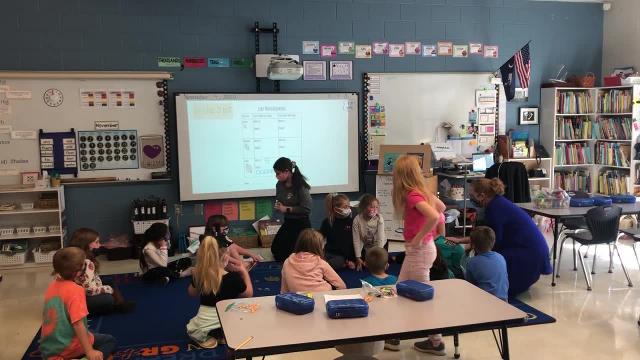 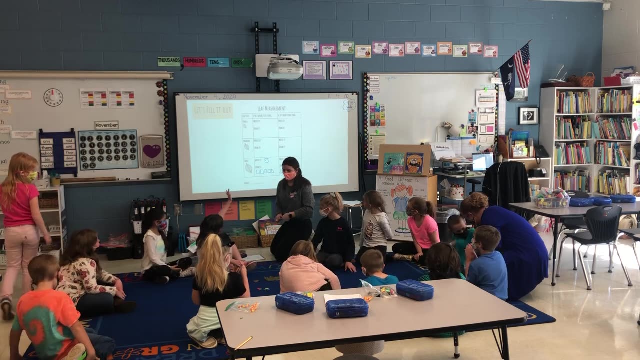 Is that all right? Five, Please stop. Ten, Ten, Ten, Nine, Please stop. Ten, Please stop. Please stop. Please stop Five. Okay, so what did we notice while measuring that leaf, Carly Sue? what did you notice? 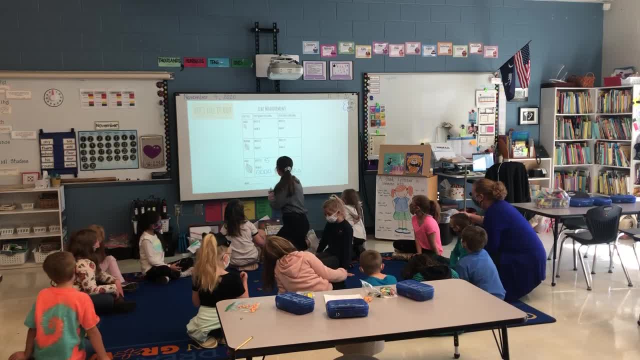 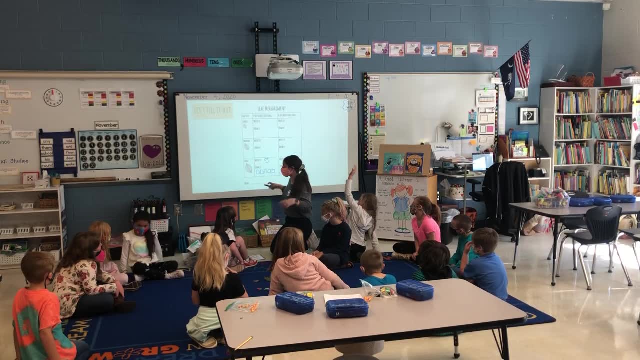 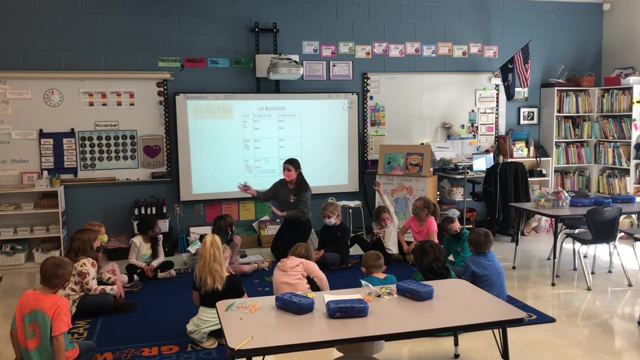 That they both had different numbers because the squares are bigger than the candy corn. Oh, Carly Sue said they were the same. She said they were different numbers and she compared our forms of measurement because she said the squares were bigger than the candy corn. so that meant there are less squares and more candy corn. 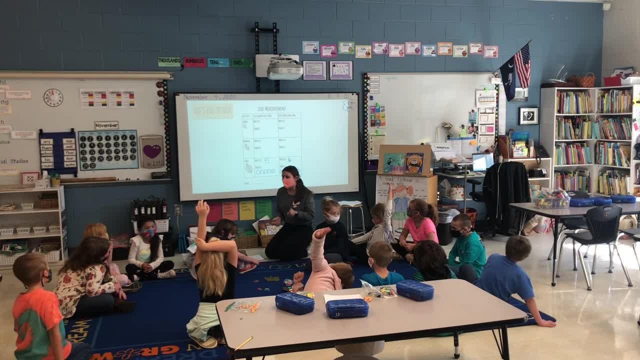 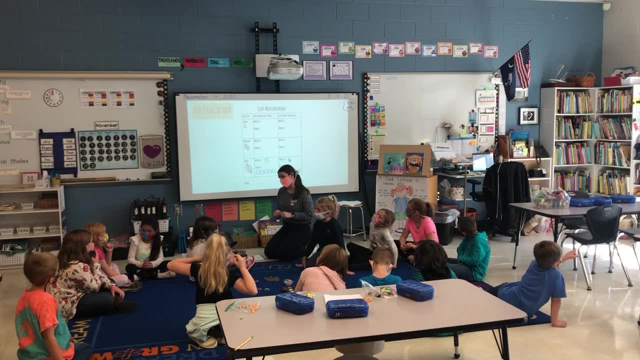 So what tool was easier to measure with What? do you think The candy corn? Why do you think that, Reagan? I think the candy corn because the square tiles they're bigger and the candy corn are easier because they can take up a little bit of space. 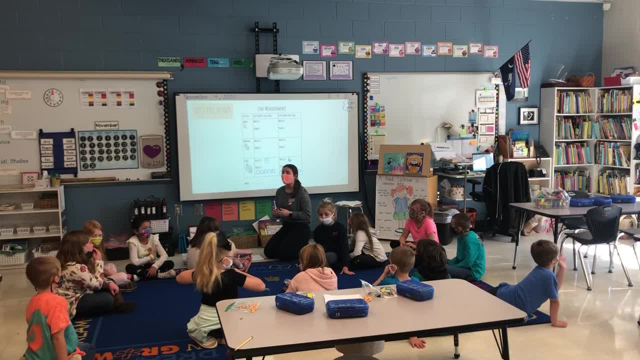 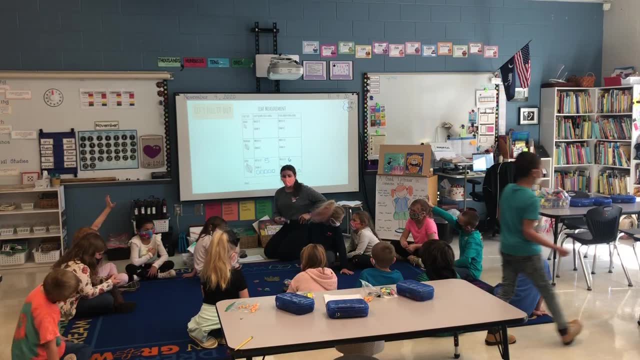 Okay, A little bit of space each if you put them down. Okay, so Reagan thinks that measuring with the candy corn was easier because they're smaller, so you could use more Mm-hmm. Okay, so what else can? what other object can we use to measure that leaf? if we were two? 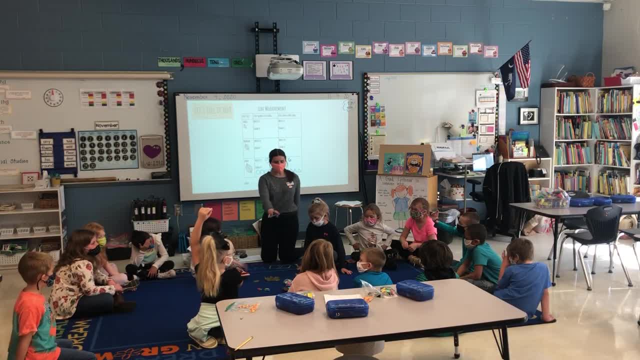 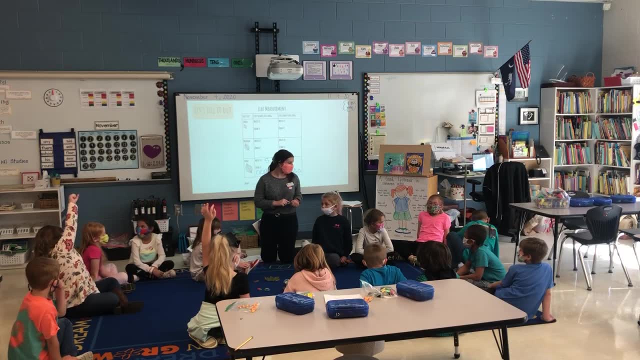 What other object, Noah? what would you use? A different object or those two? I just want to go to the safe place. Okay, Elia, what would you use to measure the objects? I would probably use some circle and that. 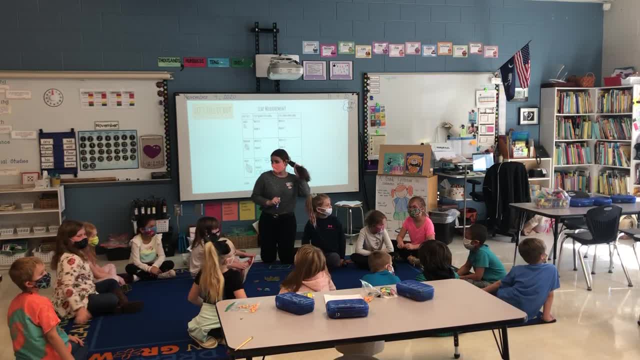 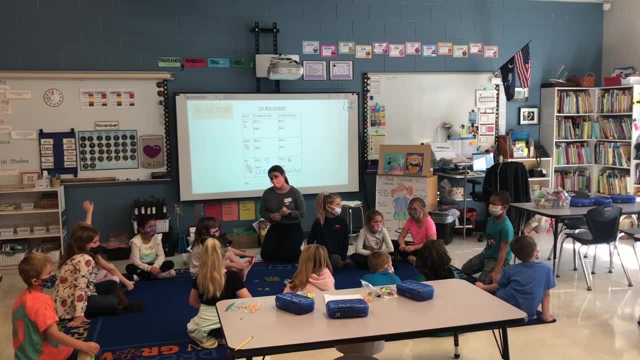 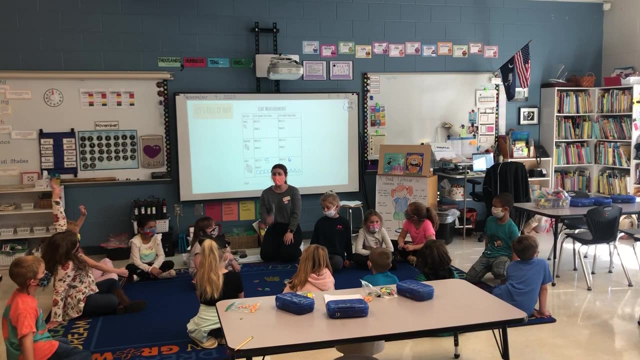 Ooh, Elia would use circle magnets. Amira, what would you use If I had a leaf and I could take it inside? I would use bouncy balls if they didn't roll A little. Okay, so Amira says she would use bouncy balls if they didn't roll. 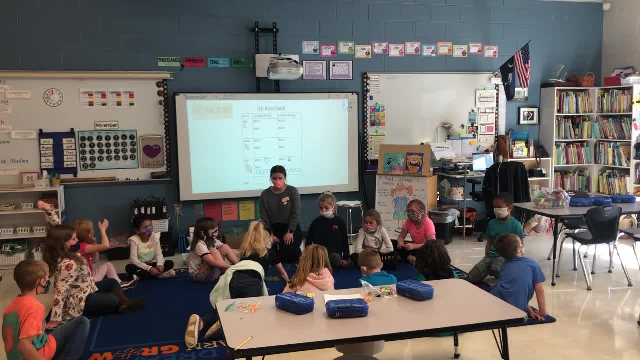 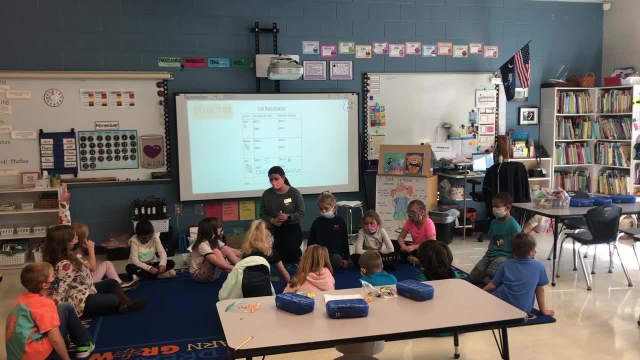 Why is it important for them not to roll So like if this was, if it was, if it was a ball, it would keep rolling away, It would keep rolling away. So maybe some space, Some space would go in between it. 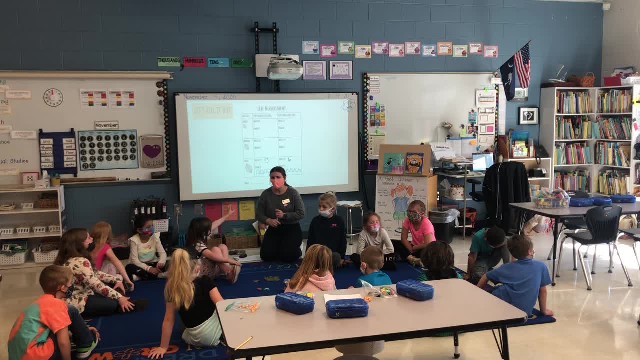 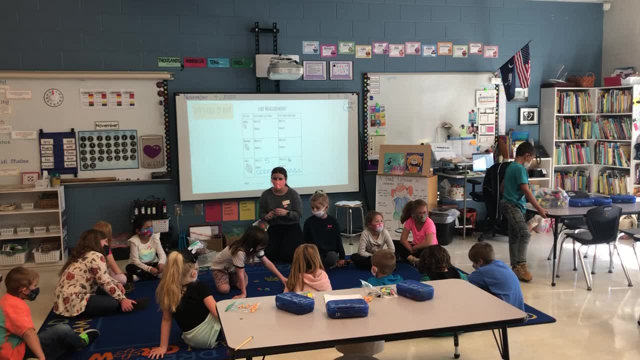 What would happen to the measurement if some space were happened to be in between each of the objects? All right, let's see what would happen. It would get messed up because, like it wouldn't be that because there's gaps. Like there's a gap, so it wouldn't choose five. 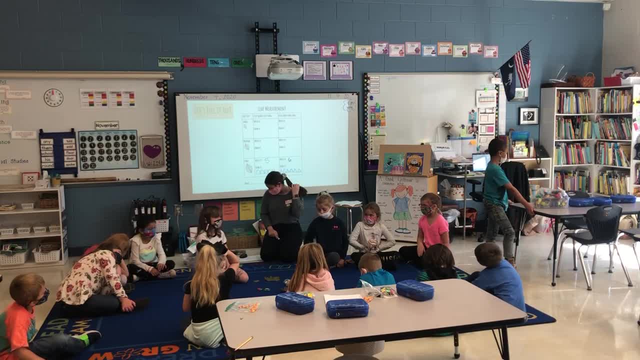 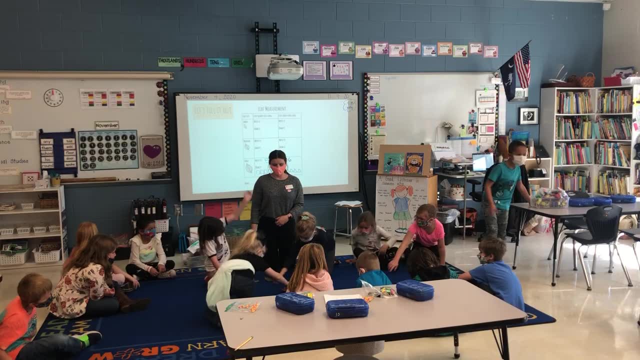 So our measurement would mess up if there were some gaps? Yeah, I think that would happen. Yeah, because if there was gaps. So how would our measurement change if we used both candy corn and square tiles? It would be different. It would be more and less. 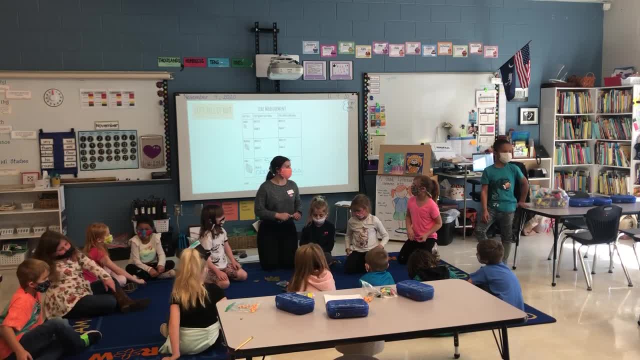 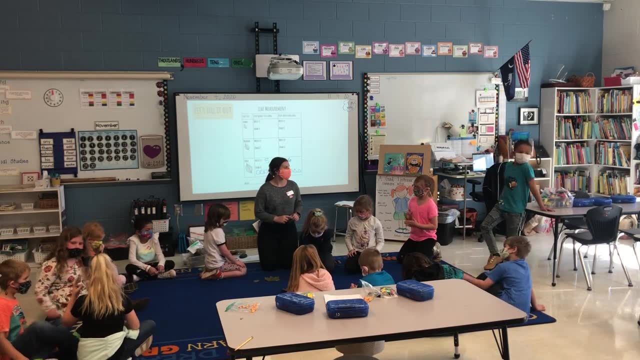 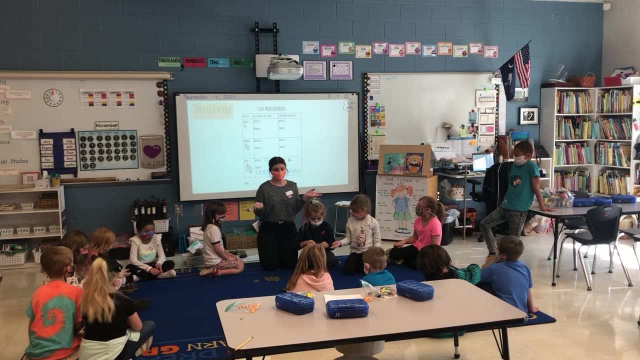 Like, like, a little bit, like more and a little bit of less. that would like probably make a big number or a small number. If it was a small leaf it would be a smaller number. So Eliane said if we use both candy corn and square tiles, our number would change. 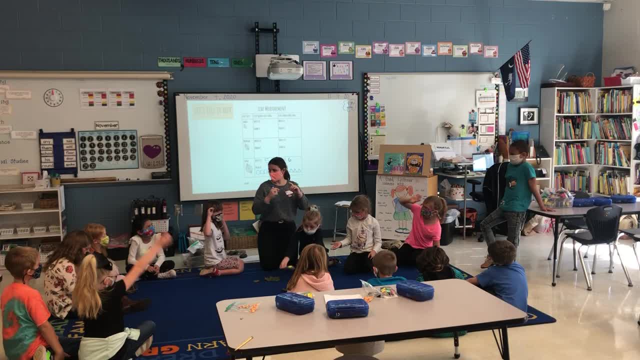 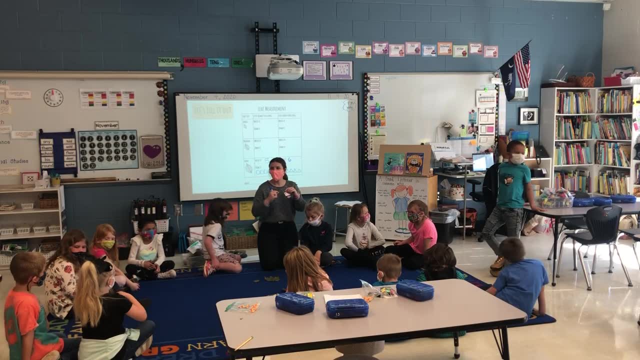 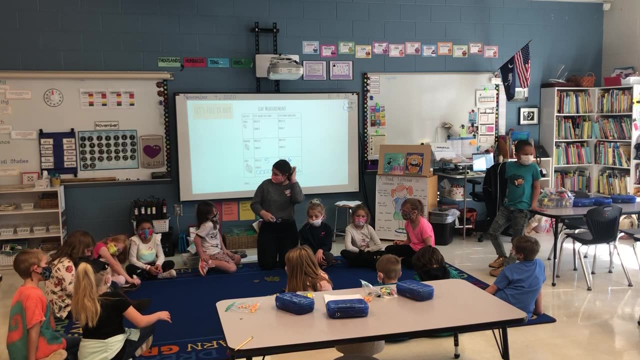 Why? why would our number change? Does anyone know, Amira, do you know why our number would change? Because we have more of the tiles And that will make our number change. It changes Like if we have six, um, candy, um, and we add one more, it will be seven. 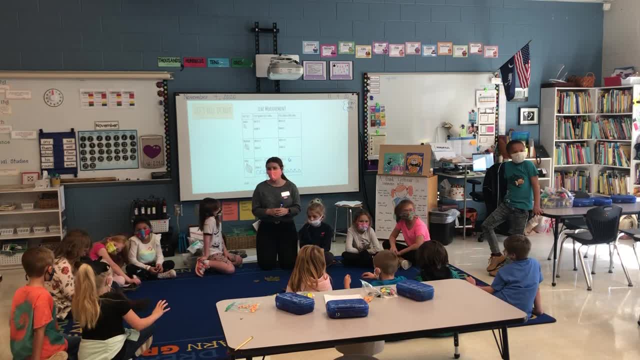 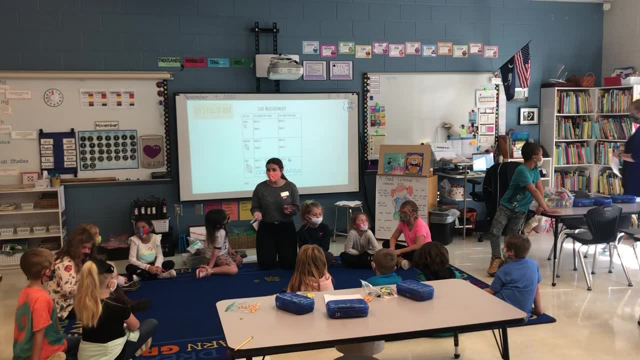 And if we have six squares, um, if we have five and we add one more, it will have six. Okay, so like just the number would be off. I think what um I saw is that if we use both candy corn and square tiles, are they the same length? 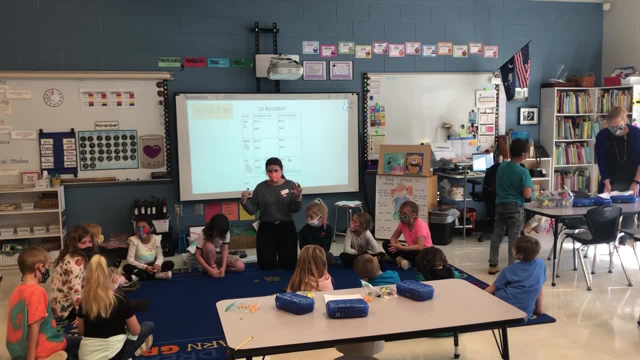 No, No, They're not Carly Sue, No, No, so our number would be messed up. So I don't think it would change. I don't think it would be that accurate, Do you guys? does that make sense? 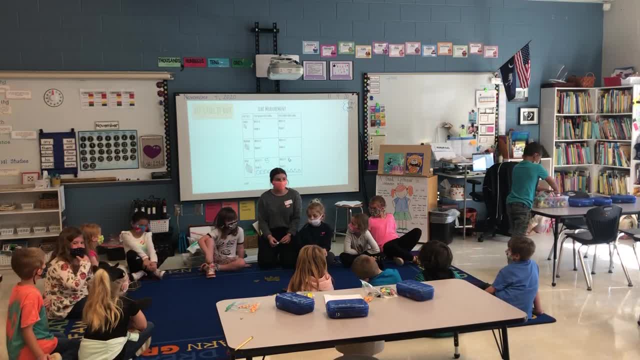 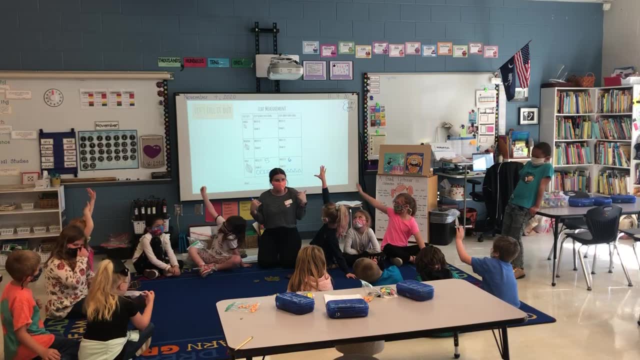 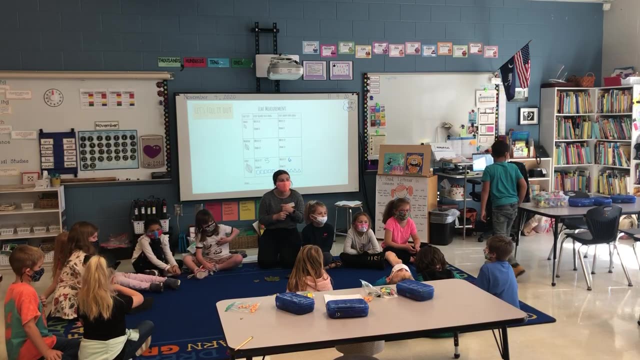 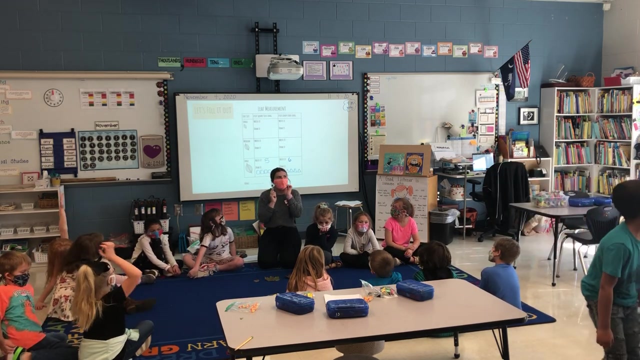 Yes, Awesome, Alright, Did you guys enjoy that lesson? Yeah, So can anyone tell me, like why measurement is important? Jackson, You have to know that stuff to measure things. Um, what um can we use to measure, like, say, um, hmm, 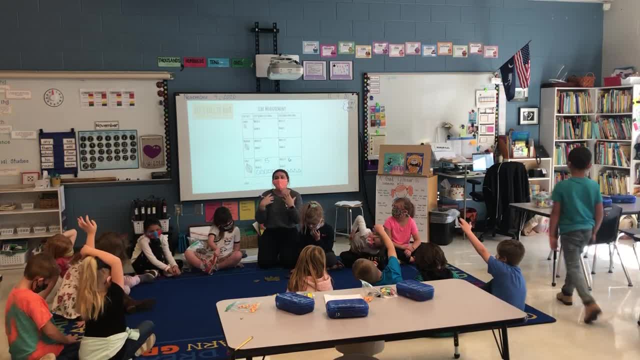 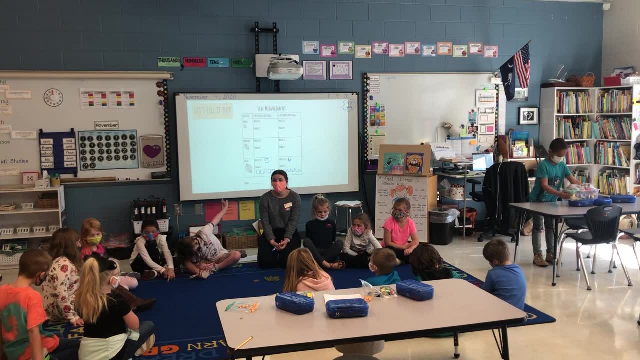 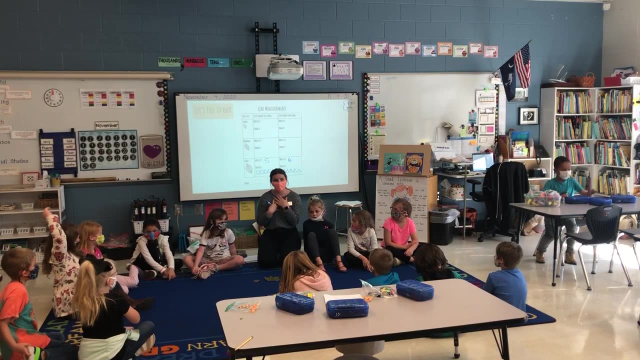 What kind of occupation would think that measuring is super important? Amira, Measuring is super important, so you know what length it is, What length it is. So I built a porch swing with my dad this summer, And do you think we just grabbed random pieces of wood and just started hammering together? 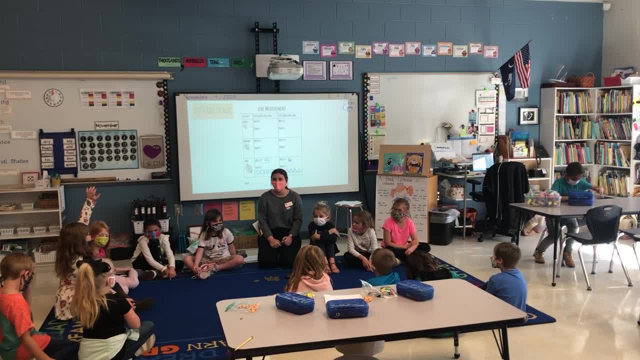 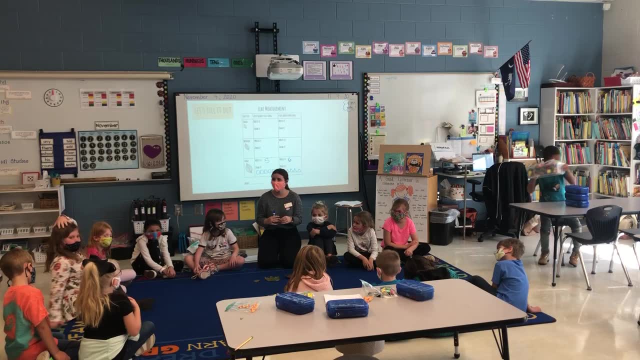 No, you know, you have to know the length of the type of wood: Mm-hmm. Or if you're trying to make something Like like um, if you're trying to make um like um, something out of cardboard. 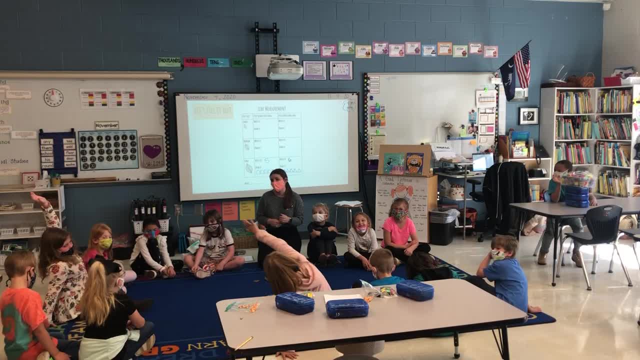 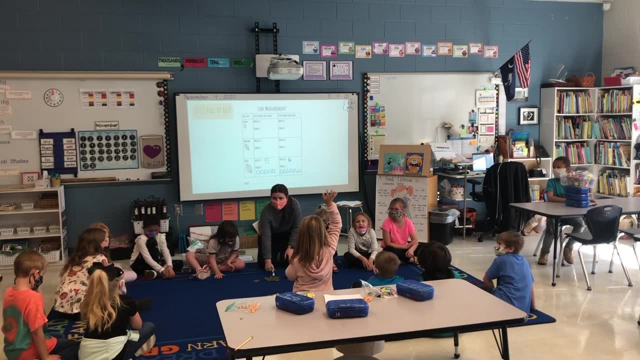 you need to know the length of the things that you need to use. We need to know the length to use um, so that everything fits together. Yeah, So did we have to use a ruler to measure something? No, No. 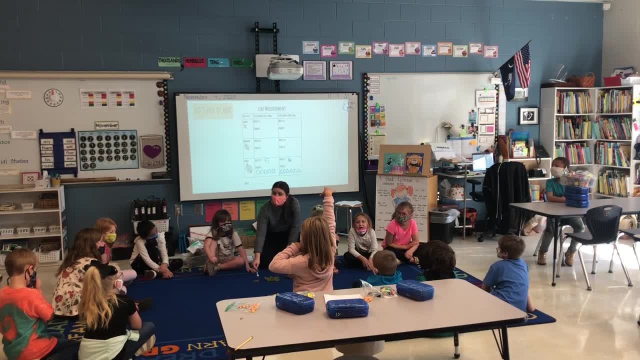 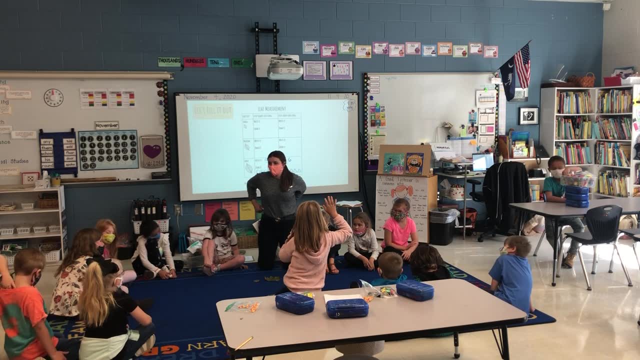 Can we just use objects that are multiple, objects that are the same? Yeah, That would be very beneficial, Like at my auntie's. we have to know the length. we have to know the length of the boxes that, um, the cardboard boxes that we need it to do. 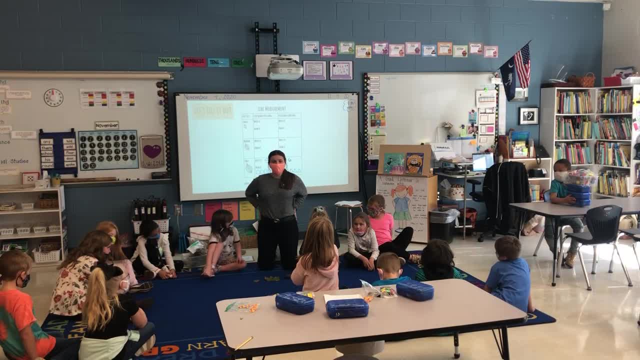 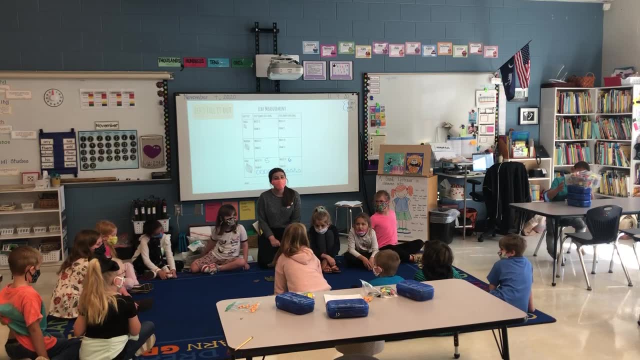 And um wires and stuff. I have a connection. What's your connection? Wait please. My grandma at her house she's making a deck and I told her we could use about 20 because of the length Of the length. 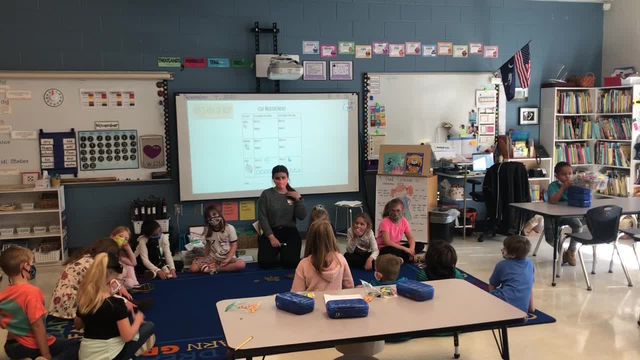 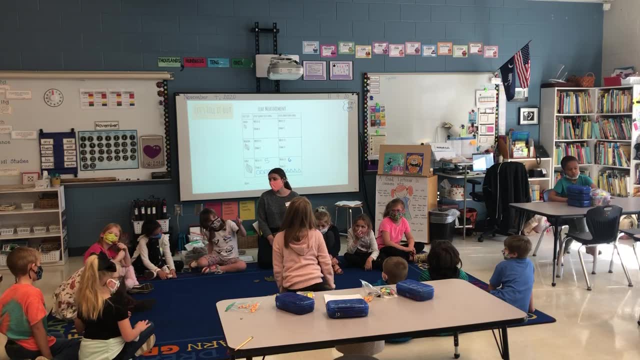 Yes, And I I just have one more that I need. I actually needed 19.. Oh, okay, So length is important for knowing how much of something that we need. Yeah, It's like how, like, how big you want it. 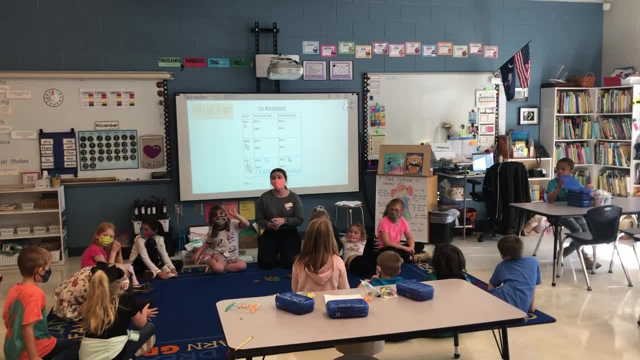 Yes, Yes, The size, Okay, so I think it is time to line up. Um. are we going to go to the restaurant? We, our lunch is not here yet, so we will. we're going to go to the restaurant quickly. 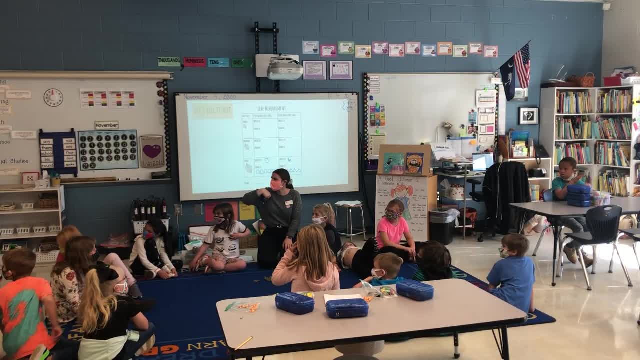 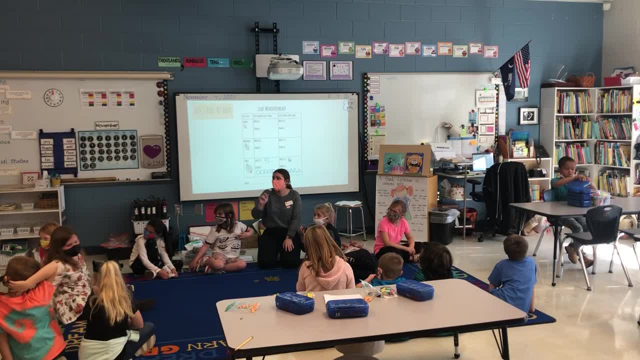 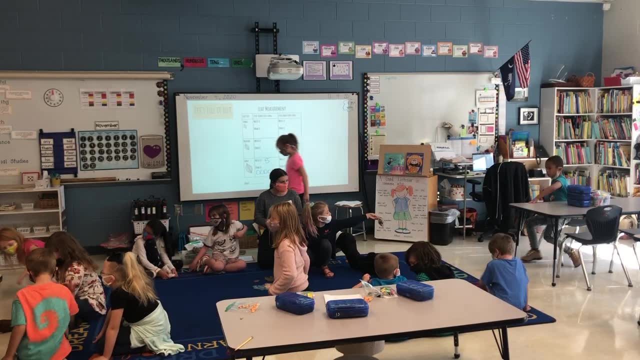 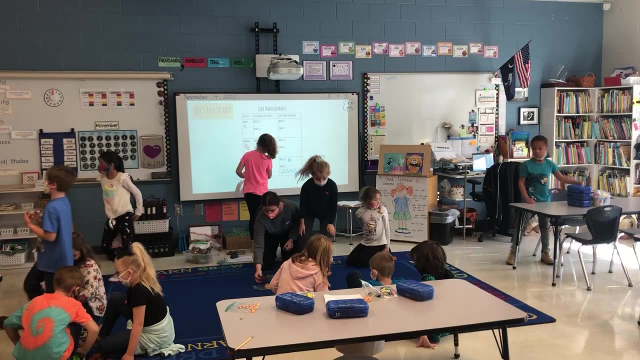 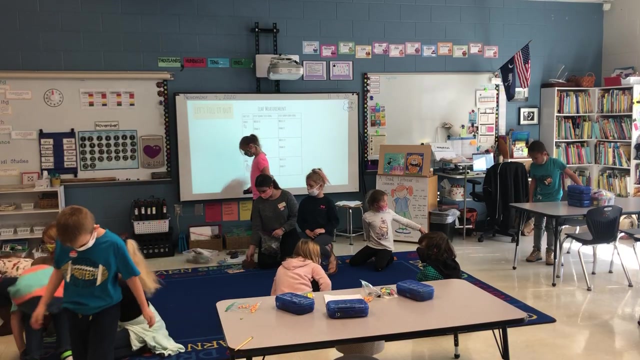 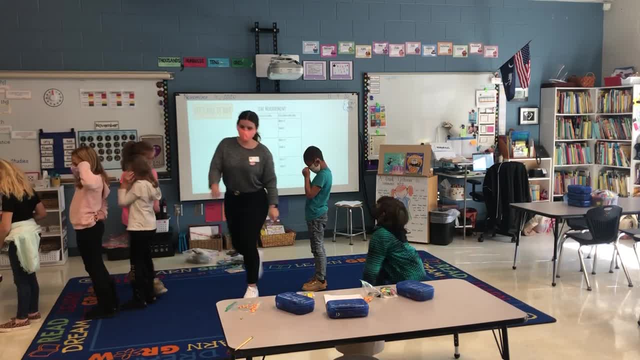 We had shoulder straps. I still have it. Be careful, Yes, Thank you.